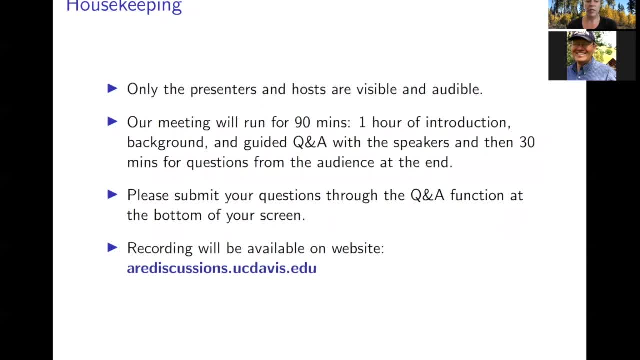 and that will be followed by approximately 30 minutes of question and answer from the audience. So please be submitting your questions via the Q&A box at the bottom of your screen throughout the webinar. Brittany will be collecting those and asking those of our webinar participants at the end. 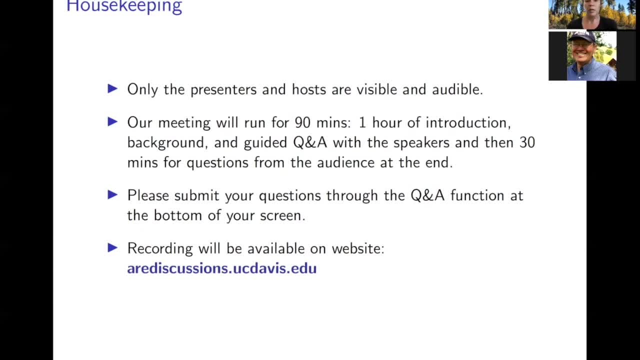 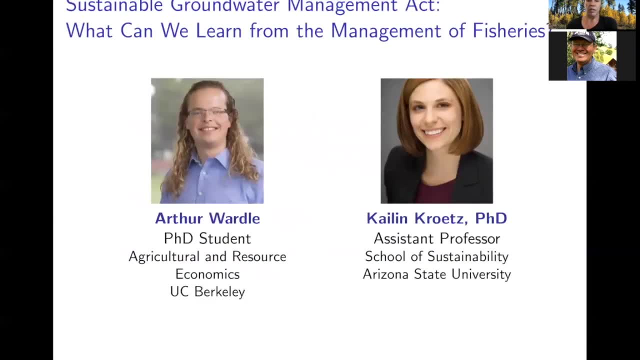 I want to remind you all that our webinars are recorded and are available on our website, which is arediscussionsorg. So, as I mentioned, this is our third in a webinar series focused on SGMA. Today, we're going to be focusing on how the management of fisheries may be informative for the development of water markets. 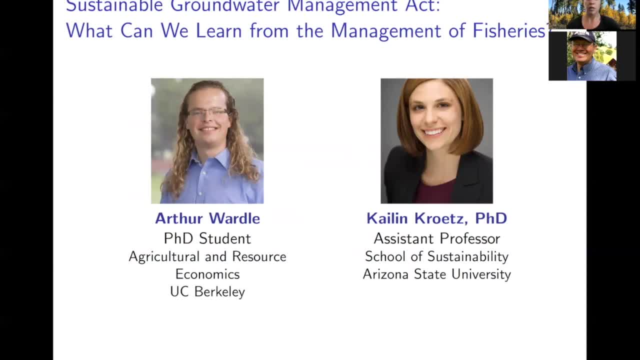 I'd like to briefly introduce you to our guests. First is Arthur Waddle, who's a PhD student in Agricultural and Resource Economics at UC Berkeley. We also have Kaylyn Kress, an assistant professor in the School of Sustainability at Arizona State University. 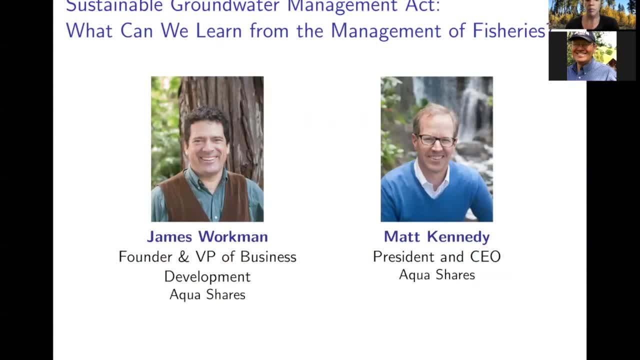 and two individuals from AquaShares. First, James Workman is the founder and vice president of business development, and Matt Kennedy is going to be joining us toward the end of the program for Q&A. He is the president and CEO, So at this point I'd like to turn it over to Arthur. 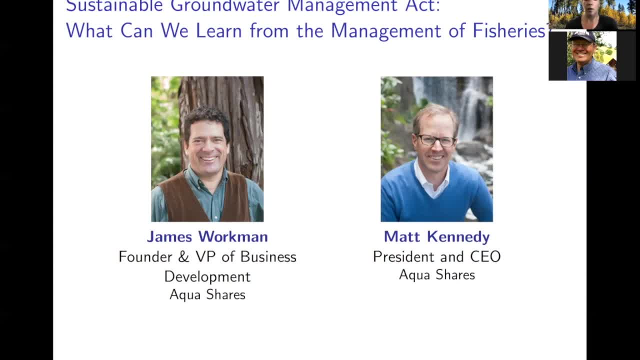 who is going to give us a brief introduction and some background on SGMA before we get started. Thank you very much for joining us, Arthur. I'm going to turn it over to you Arthur Wardle, Thank you. So, like Tina said, my name's Arthur Wardle. I'm a PhD student at UC. 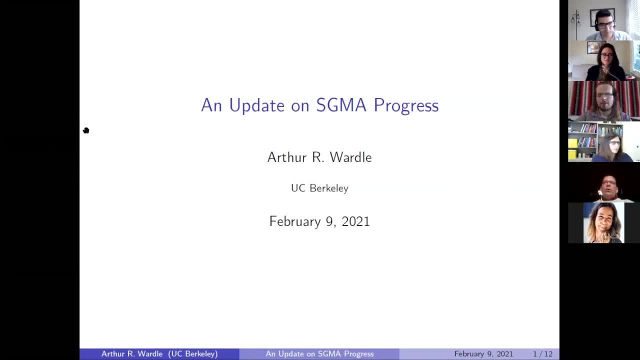 Berkeley and I'm presenting today some data and analysis of that data. It's part of a project I'm doing with Dr Bruno and an undergraduate, Paige Griggs, at Berkeley, Hoping to give some background on where we are in SGMA, since SGMA is going to be open to the public, So I'm going to take a moment. 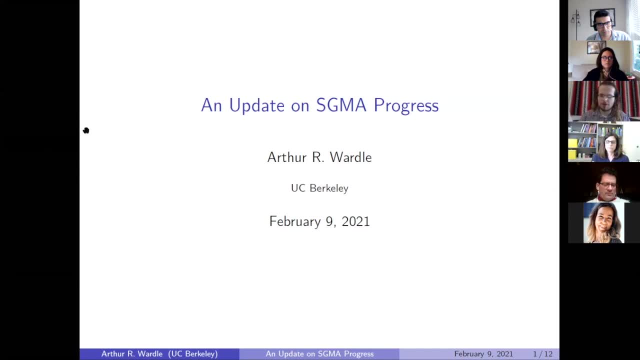 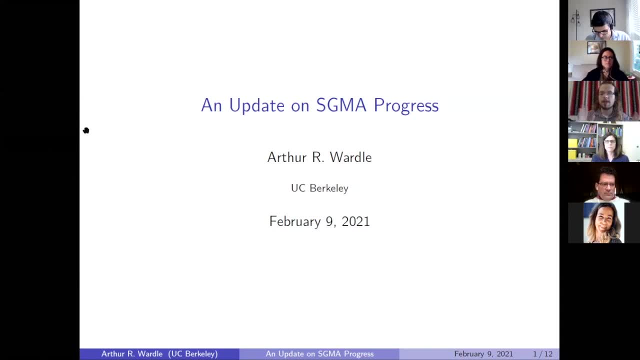 about what the role of groundwater markets looks like it might be as SGMA develops. So the basics of SGMA is that it requires groundwater basins in California to develop plans to prevent issues associated with long-term unsustainable extraction of groundwater. The getting back to sustainability. 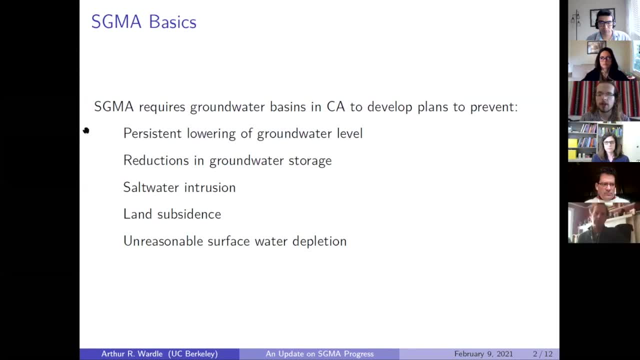 is going to require pretty sharp reductions in groundwater extraction in many parts of the state and the amount of agricultural land that needs to come out of production and other things like that is going to depend heavily on the management actions that basins decide to take. to get back to 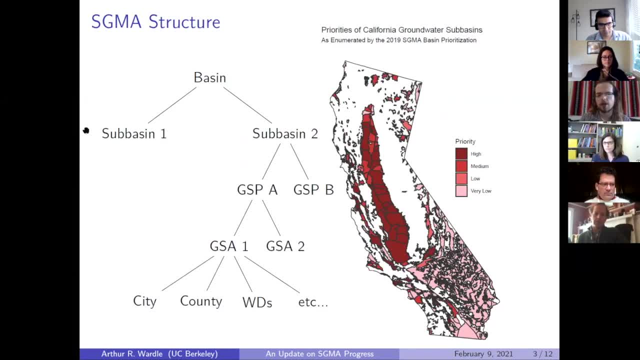 sustainability. So the structure of SGMA looks like this: on the right hand side first you see the department of water resources to split the state into sub basins, which are designated high, medium, low or very low priority, depending not only on the extent of their current groundwater. 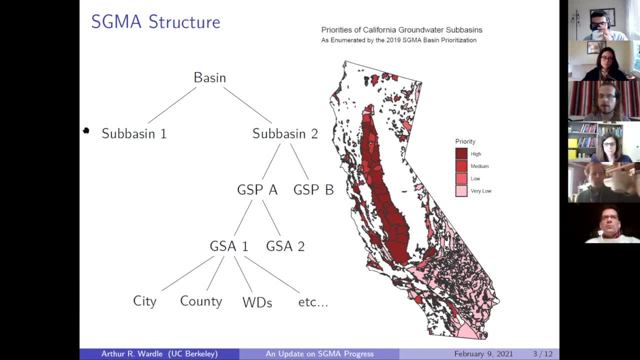 issues, but also on things like projected future demand for groundwater In the high and medium priority basins. local agencies- pre-existing local agencies with land and water use responsibilities- needed to join together to form groundwater sustainability agencies. They could do that either independently. say: a water district takes over the GSA. 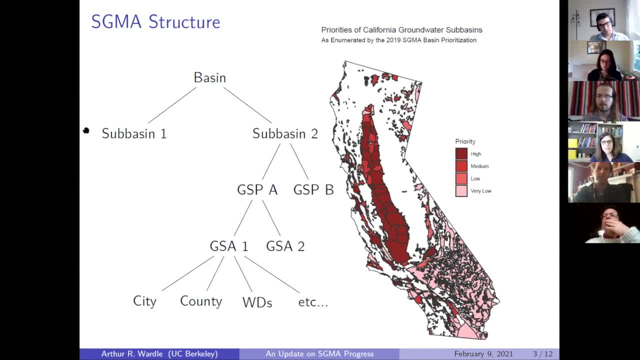 mantle for its service territory, or multiple agencies, including cities and counties, can come together and form a collaborative GSA. Those agencies are then responsible for producing groundwater sustainability plans, which they can either, again, do independently or, because these plans tend to be pretty intricate and long and expensive to write, many GSAs decided to. 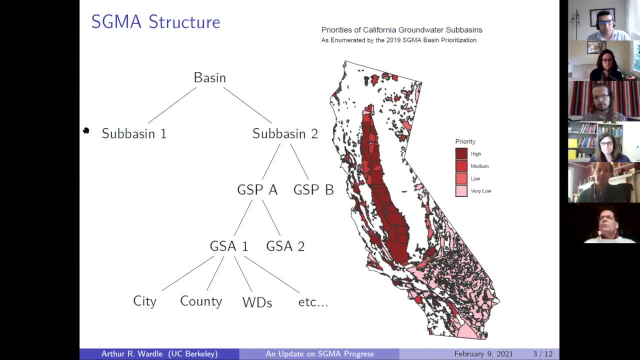 do this collaboratively, working together on a single plan, And then ultimately those plans have to be managed by a subbasin or the entire subbasins, and the subbasin is kind of the highest unit of management at issue under SGMA, and in some cases a subbasin is just the entire area of land overlying. 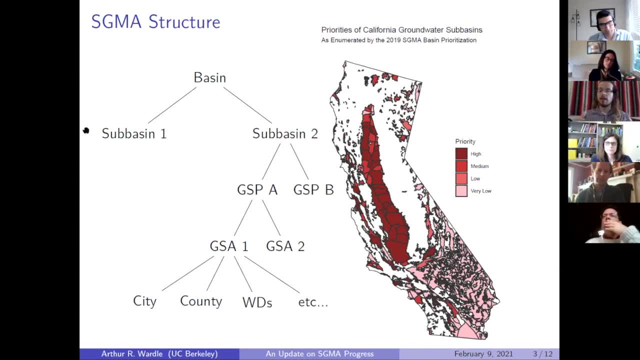 a single aquifer. but in most cases- in many of the most important cases like the San Joaquin Valley- the underlying aquifer is so huge that it would be unrealistic to try to coordinate closely demand across the entire aquifer. so instead it was split into different subbasins, So a subbasin would be. 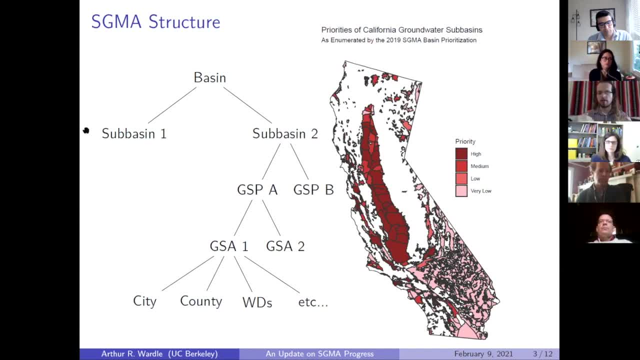 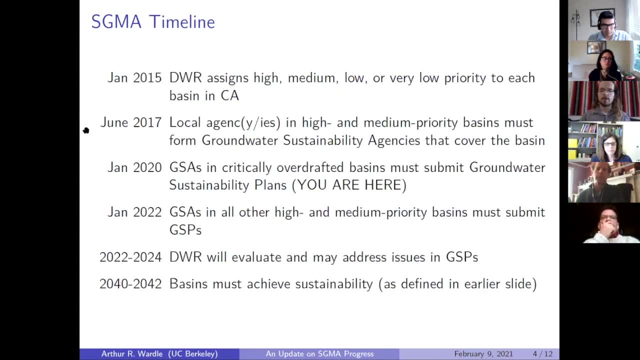 a subbasin and a single aquifer aren't necessarily synonyms under SGMA. Here's where we are in that timeline. In 2015, the basin prioritization occurred. By 2017, local agencies in those high and medium priority basins had formed groundwater. 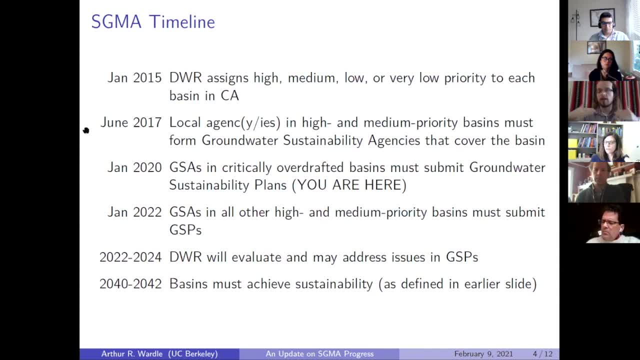 sustainability agencies whose territories jointly covered the subbasins. In January of last year GSAs in critically overdrafted basins had submitted their groundwater sustainability plans. so we have those in hand now. In January of next year we're going to get those from the rest. 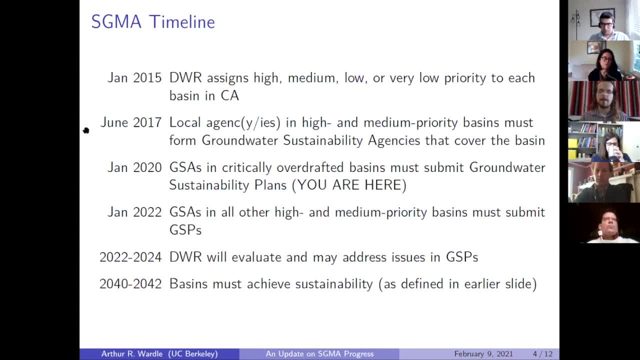 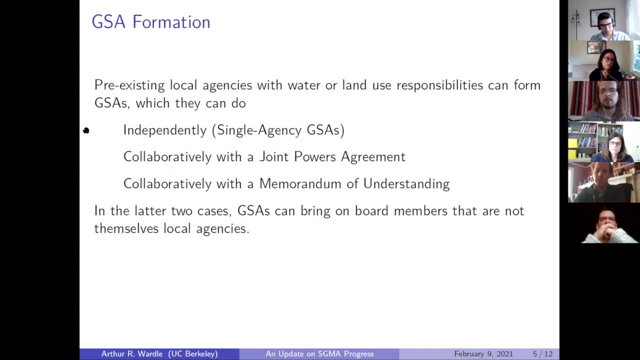 of the GSAs in high and medium priority basins Over the next couple years the Department of Water Resources will evaluate and address issues in those plans and then by 2040 to 42 basins are going to have to achieve sustainability as defined in that initial slide. So the way, the GSA formation, 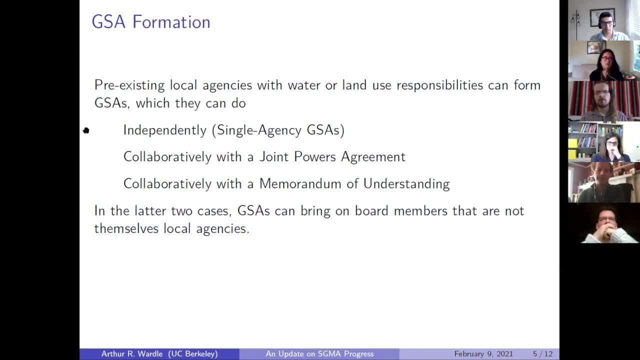 process works- I've talked about this a little already- is that those pre-existing local agencies with water and land use responsibilities form them either independently or jointly, with a joint powers agreement or memorandum of understanding And, in those two latter, collaborative cases. 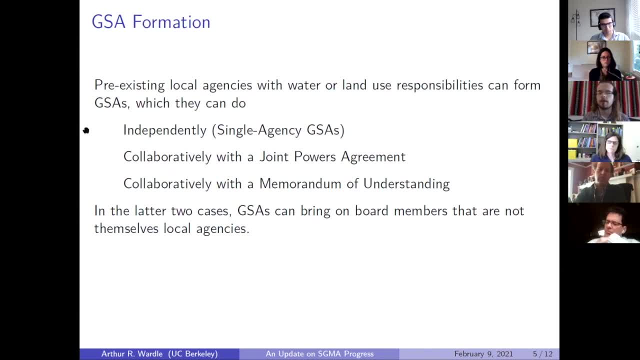 GSAs can involve board members that are not themselves local agencies. So people from a local farm bureau or environmental NGO can be given a board seat in order to influence the decision making at that GSA. There are 224 distinct GSAs In the state, 155 of which are just single agencies that have taken on the GSA mantle. 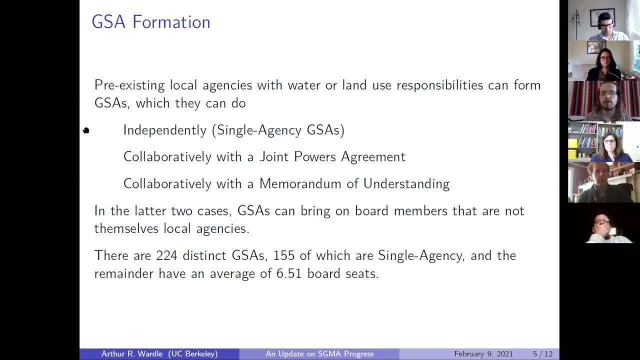 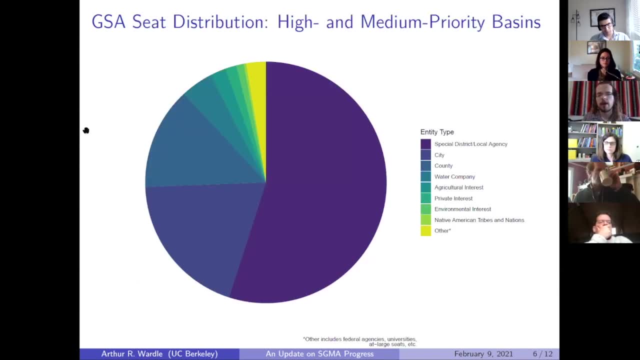 And those that are collaborative. the rest of those 224, have an average of 6.51 board seats. This pie chart breaks down who, what organizations those board seats belong to, And this treats those single GSAs as just having a single board seat belonging to that forming. 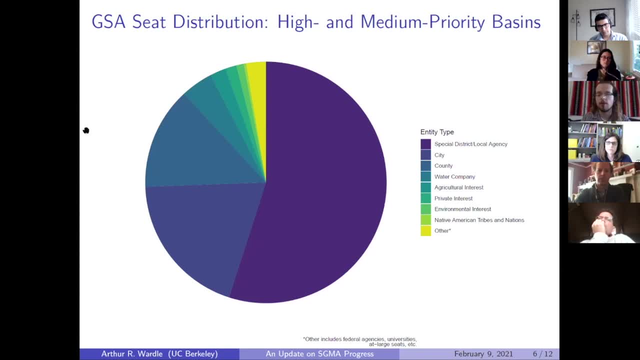 agency. So you can see the majority are special districts and local agencies and the majority are local agencies, Almost all of which are water districts, irrigation districts, reclamation districts, other districts that have a historic role in delivering surface water supplies to agricultural users. So you can see why these districts have a clear interest in the development. 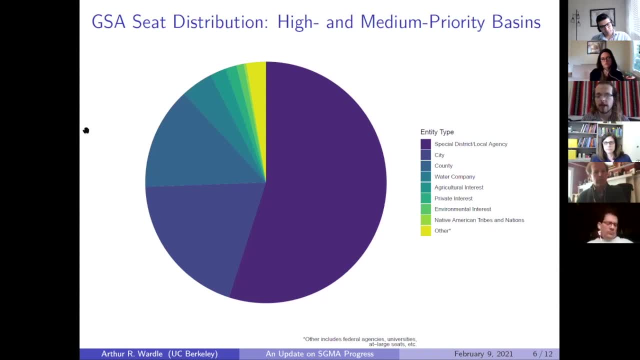 of groundwater management policy. The next biggest are the cities and counties. Counties have a unique role under SGMA as the backstop GSA for any portion of a sub-basin that doesn't organically have some other agency decide to become the GSA in that area. But both cities and counties are 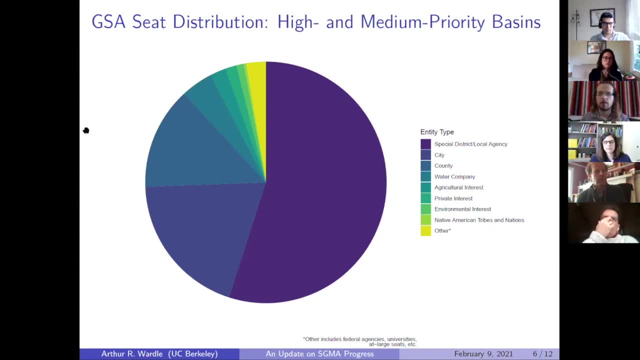 also involved in delivering water to municipal users, so also have a clear interest in how water management happens. And the remaining seats belonging to people like domestic well holders or environmental NGOs make up a very small share of the total board seats on GSA boards somewhat. 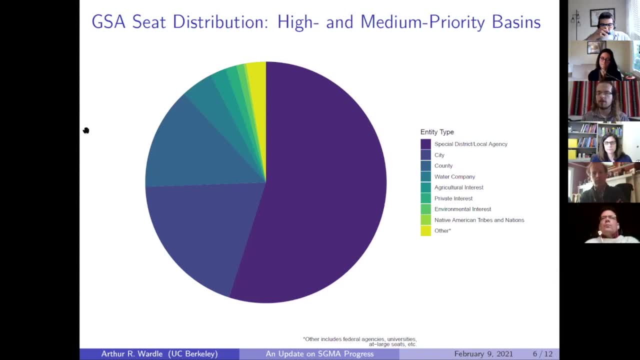 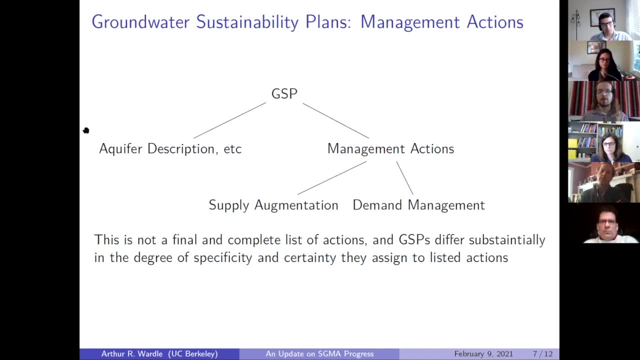 by design, since they can only be involved in these collaborative GSAs where they're invited by these local agencies. So those GSAs have to write groundwater sustainability plans which have a lot that go into them, including a lot of very scientific technical description of the 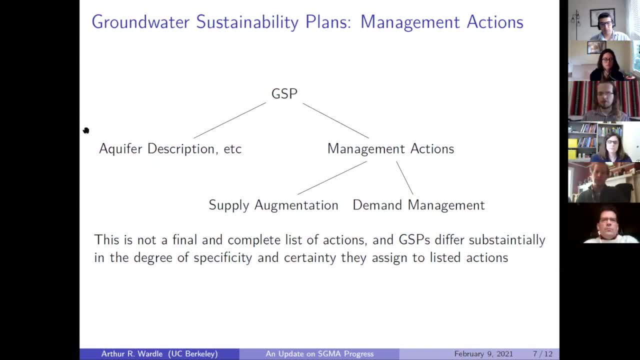 hydrogeography of the underlying aquifer, which is important, but not something we're interested in or collecting data on. But what we're collecting data on is the management action section of the groundwater sustainability plan, which is a little bit more complicated than the groundwater. 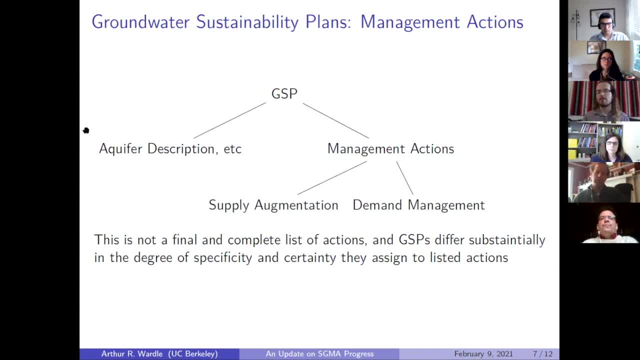 sustainability plan, which is a little bit more complicated than the groundwater sustainability plan, which is a little bit more complicated than the groundwater sustainability plan, which is a list of the projects and plans that these agencies are developing that they're going to use to try to. 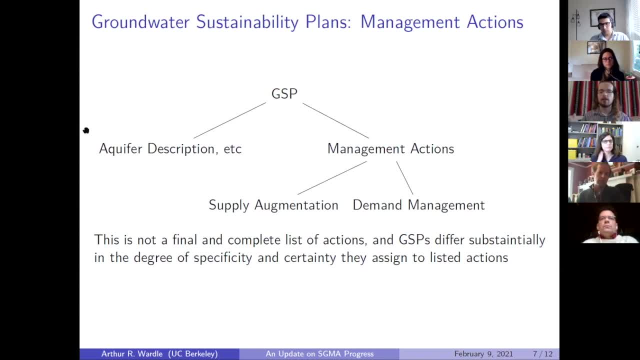 get groundwater extraction back to sustainable levels. So these can be kind of split into two big. So these can be kind of split into two big buckets, the first being supply augmentation, which is trying to find surface water supplies to recharge the aquifer with, like stormwater or wastewater. 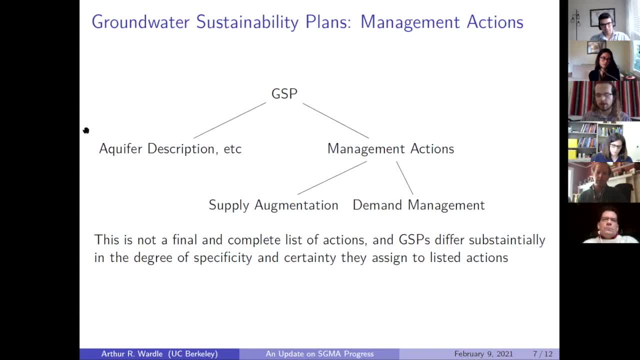 or something like that. Basically, every groundwater sustainability plan includes some amount of of this. it's very popular but ultimately this is not going to cut it for most gsps, just because there is not an adequate amount of unaccounted for surface water necessary to deal with the 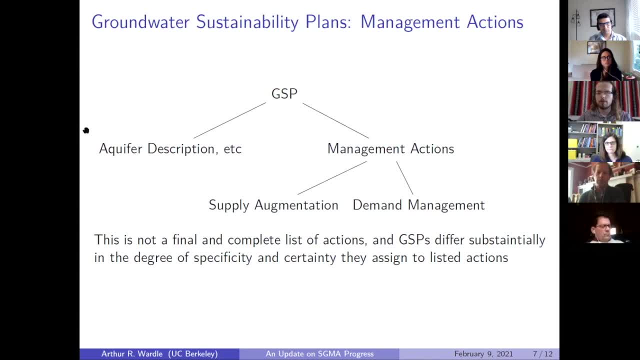 entire scope of the unsustainable groundwater extraction problem. so that leaves the second bucket, which is demand management, just broadly meaning any way that you can try to get people to consume less groundwater, which i'm going to break that up further in these next few slides. but i do want to first emphasize that these gsps don't give a final and complete list of actions. 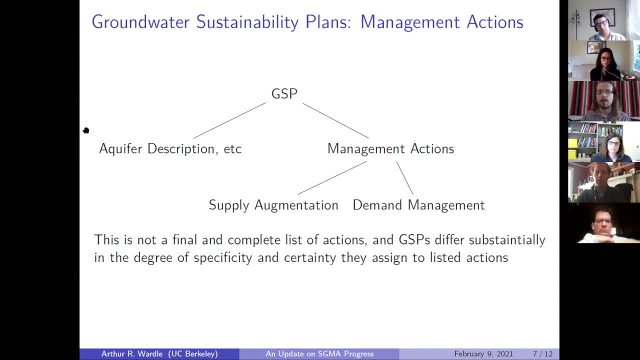 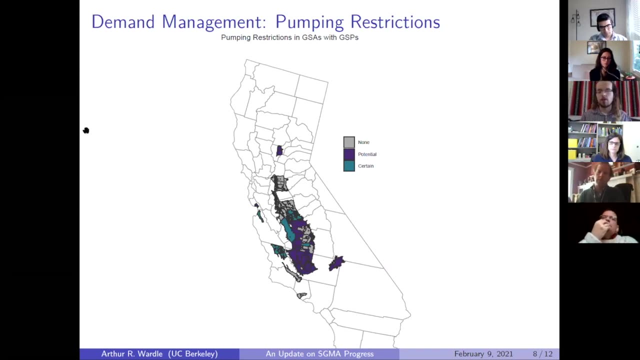 and the plans that we have looked at differ quite a lot in terms of how specific they are about what actions they're going to take and also in terms of the degree of certainty. there's a lot of we might do this, we might do that going on in the current plans. so the first, uh, kind of command and control. 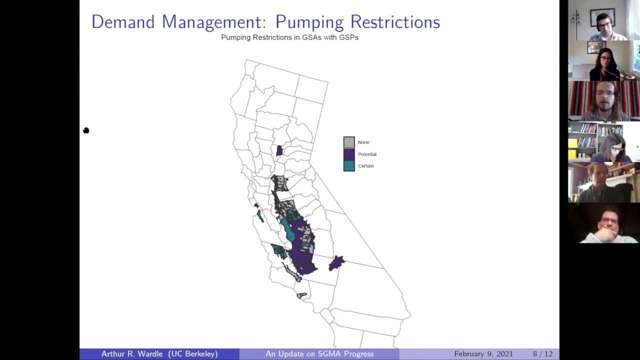 type demand management action you can take is an outright pumping restriction. this is a map of the gsas that have submitted gsps so far and you can see the dark blue is places where pumping restrictions are being talked about as a possibility, the potential, and then the lighter blue are the ones that are saying yes, there's going to be pumping. 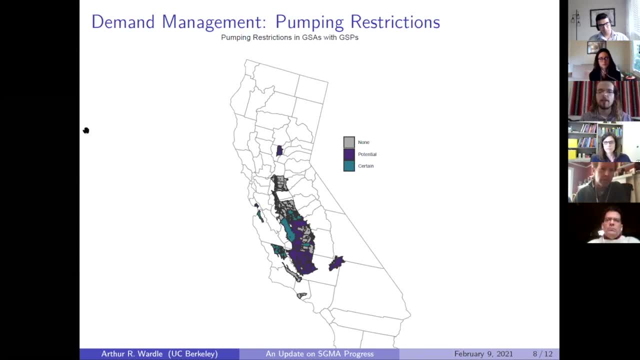 restrictions, although i want to clarify that in both cases, these pumping restrictions tend to be worded, so the pumping restrictions will only come into effect under drought conditions, for example, or after 10 years. if we haven't hit some specific target, then we're going to implement pumping. 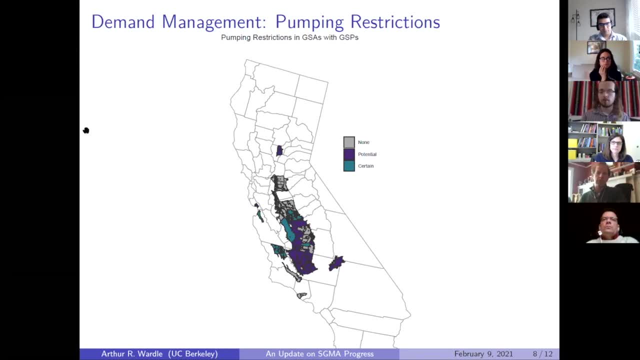 restrictions, so it's not like there's going to be a bunch of restrictions day one. but also, i mean droughts are when you want to have some flexibility in who's going to get water, because if you own, you know, a young orchard that has 20 good years of life left in it, that's a super high value crop. 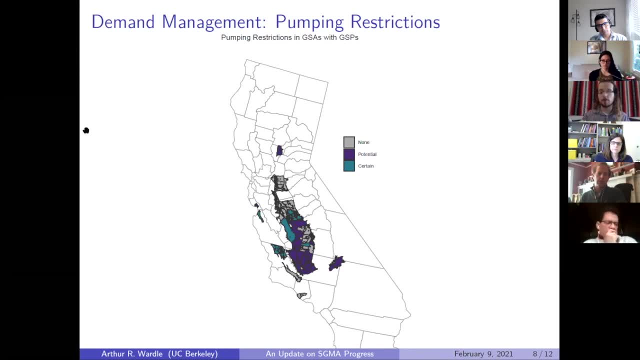 a drought, when you don't have access to enough water to keep that orchard alive, is exactly when you don't want to have a very command and control type pumping restriction on how much water you can access. another type is fees. um, you can see basically everywhere is at least considering. 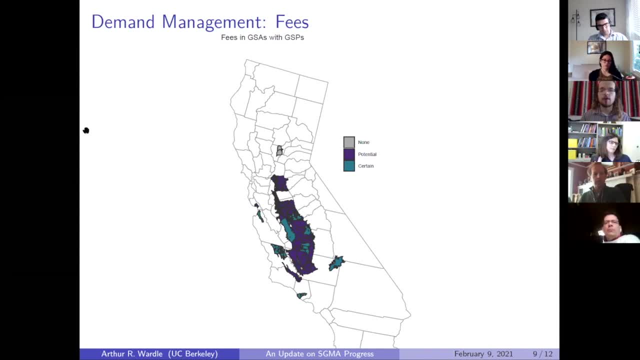 some form of fees and fees on groundwater extraction can be useful because historically, california groundwater users have been able to pump as groundwater well- maybe not quite as much as they want, but it's been very lax in terms of how much groundwater you can extract and the only price for it in most of the state has been the price. 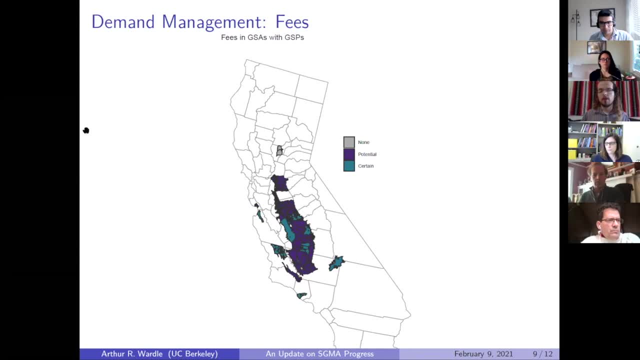 of the electricity required to run the pumps. so introducing a price on extraction itself can do things like incentivize people to make efficiency improvements, also reconsider crop choices. but unfortunately not all of these fees are on groundwater extraction itself. there are lots of costs, of course, if you plan to use a plants at a time and, for example, if you plan to use a plant. 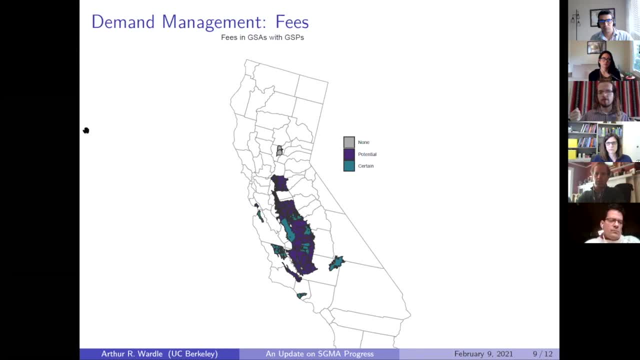 for a long time and the purposes of your strategy are not the same as they are. uh, it's only possible to use their units at a time. uh, you can't. puedes reduce their utility costs by something like one or two hundred and a half hundred dollars, and you can always use middle class systems. 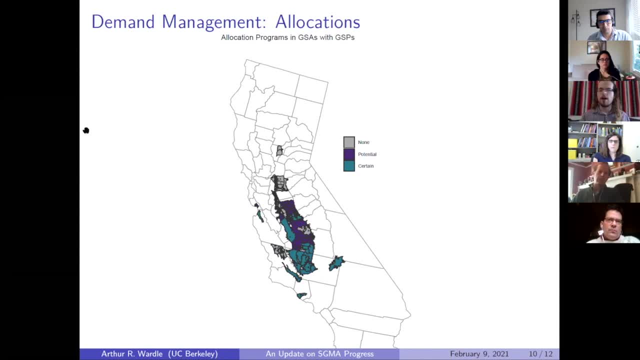 that can help you build your systems. but if you can't, you could use, you know, even those low-income systems and you could. you could do that by using artificial habitat and, in terms of property rights, they can't just straight up assign property rights, But using the powers. 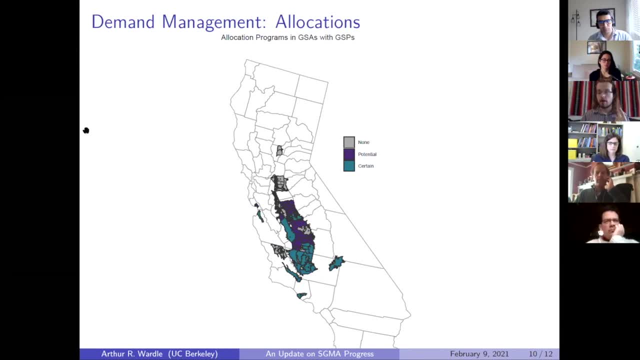 that SGMA grants GSAs, namely that they can restrict pumping at different levels for different people, as well as assess fees on extraction at different levels for different people. they're able to create some things that look a whole hell of a lot like property rights. So for 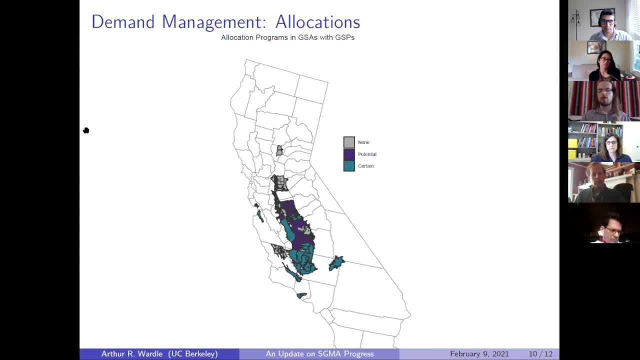 example, giving each existing groundwater user some set allocation of water for which the groundwater extraction fee is going to be very, very low, And then, once you reach that limit, the rate for your groundwater extraction after that goes way up, is one way they might implement. 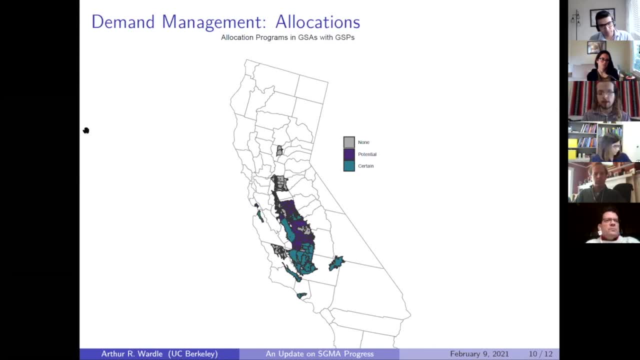 an allocation. So there's a lot of places talking about doing allocations, some with certainty, some are just talking about doing it potentially. But also, allocations on their own only go so far. So again, if you're the orchard owner in a drought, if you have an allocation, that's great, If it's. 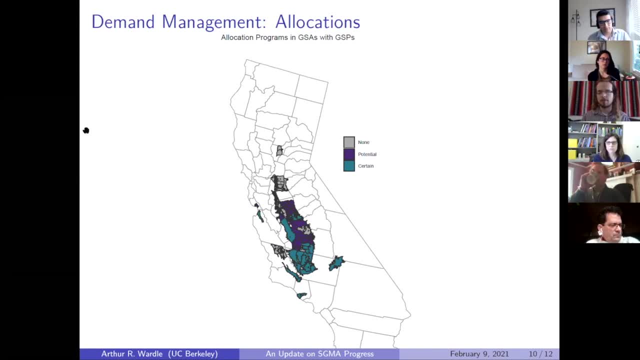 enough water. But if it's not enough water, you want to be able to trade with your neighbor who maybe is growing a low value crop like alfalfa or something in the field next door. Having allocations is great but doesn't work if you don't have enough water. 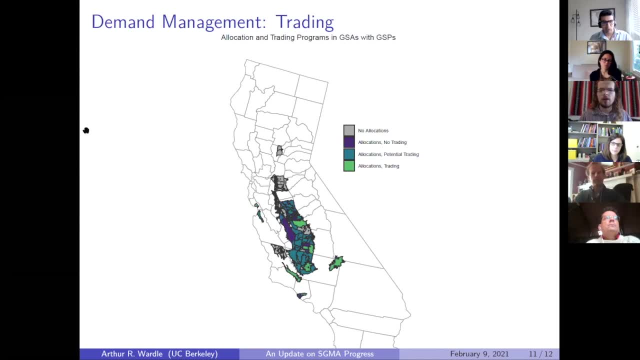 you'd like to be able to make some kind of trade. So the good news is that, conditional on at least considering allocations, almost every GSA is at least considering also allowing trading, But very few of them are communicating any degree of certainty in terms of Yes, we are going to implement trading. 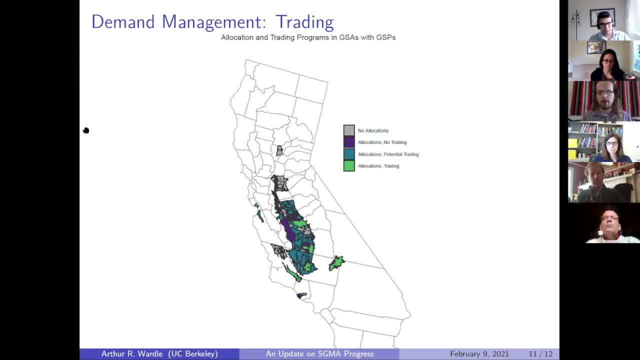 That would be the light green on this map. There's only a small handful that are talking about it with any degree of certainty. So that's where groundwater markets currently are in the SGMA governance process. So I hope that tees up some of this discussion about how ITQs have developed markets infrastructure. 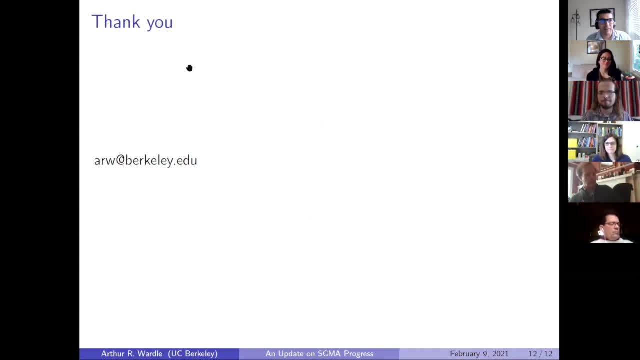 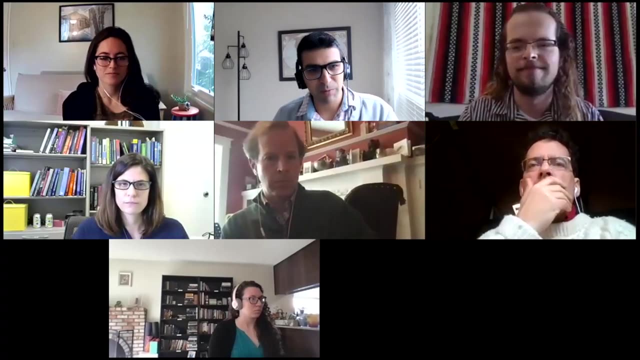 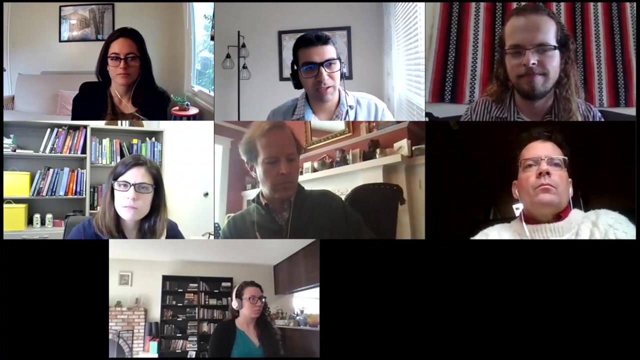 markets and fisheries. thank you. thank you, arthur. that was a great summary and update for the sigma uh. now we move to to calian that she is going to talk about uh markets to manage fisheries and what we can learn to for designing groundwater markets. uh, kalyan, if you want to go ahead and share, 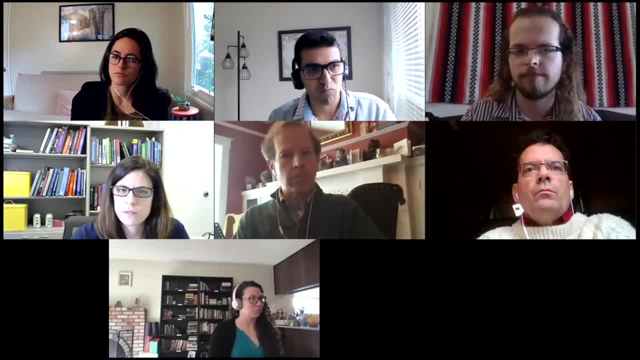 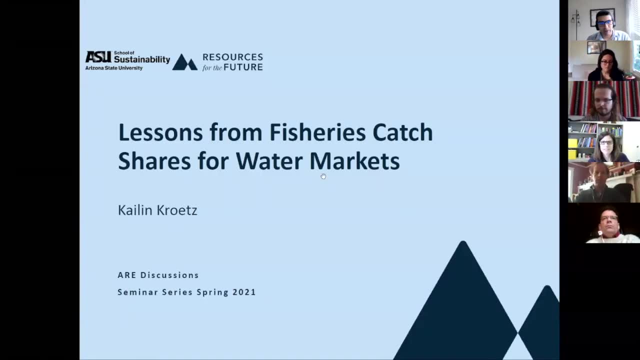 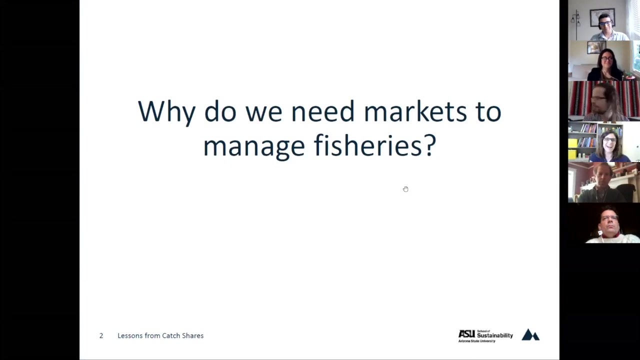 your slides and can you see that here? yes, that's, uh, that's perfect, okay, yeah, thank you very much, and carry on. to start, can you uh tell us, uh, why do you need markets to manage, uh, fisheries? uh, yes, i have a slide for that. uh, yeah, so you know, arthur, i really appreciated the the background. on sigma that i was talking about earlier and i think it's really important for us to be able to understand why do you need markets to manage fisheries and why do you need markets to manage fisheries and why do you need markets to manage and the discussion around some of the design of the 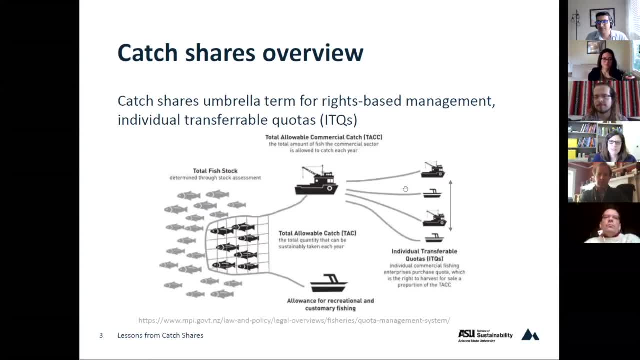 um, the sort of sub programs i guess within it. and so i thought i'd start off with a little bit of an overview and sort of fixing some of the terms that are really common, uh, to fisheries, because i think this is sort of an important thing for us to do here, um, and so i'll talk a lot about. 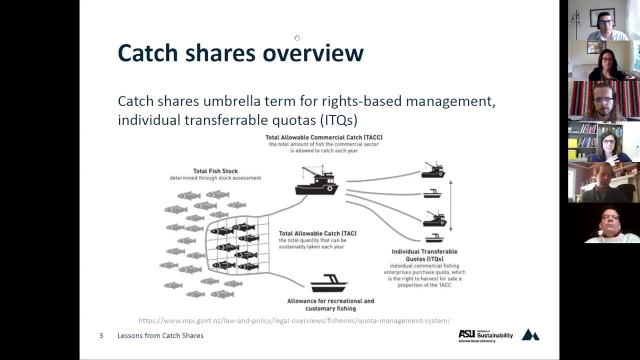 catchers, and i think that this is a good term to use, especially given what i heard of your description of sigma. so it's this broader term that is focused on allocation and trading to a certain extent, but that accommodates something beyond that sort of perfectly efficient market. 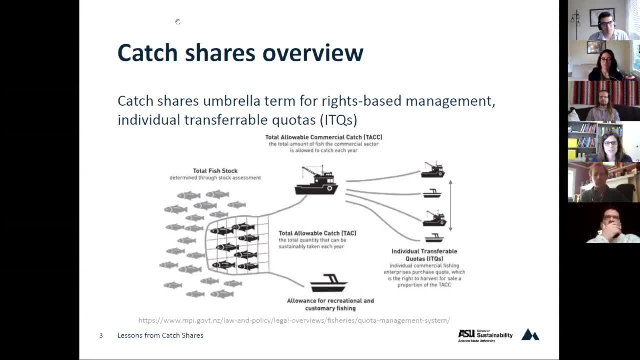 that you mentioned, arthur, that i think as economists in particular, we we always have in mind- and so this is sort of a catch-all term- uh, referring to a lot of different rights-based management program designs, and under that umbrella certainly is individual transferable quotas, and so 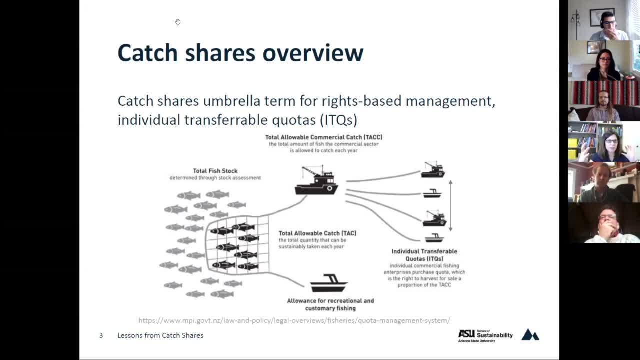 in the fisheries context, we think of the total fish stock. we assess it. we- and usually more biologists, ecologists- weigh in what's a sustainable uh amount that can be extracted. that amount is allocated. typically, if we're thinking of an itq program, we're thinking about 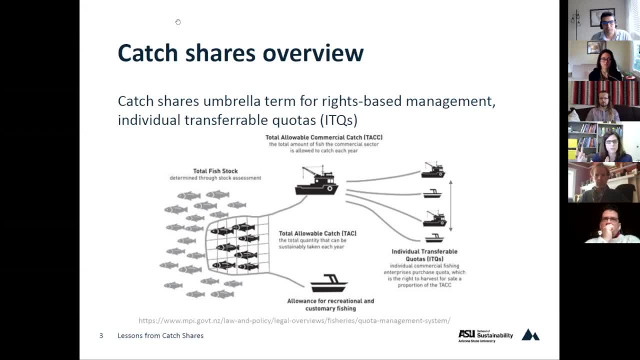 commercial fisheries. so that is allocated to the commercial fisheries sector. we usually call that allocation a total allowable catch and then from there it's allocated to individual fishers and i think, arthur, this really fits up, fits nicely with sigma. so there's an individual, individual quota program. So this is where fishers get the allocation but they can't trade it. 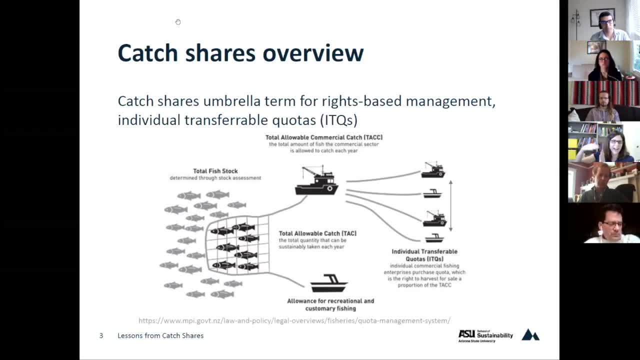 And then we have the individual transferable quota programs, which has that last piece where fishers can actually trade amongst themselves. So similar structure, I think, to what you've been talking about, but with some just different terms and transferring over to fisheries context. 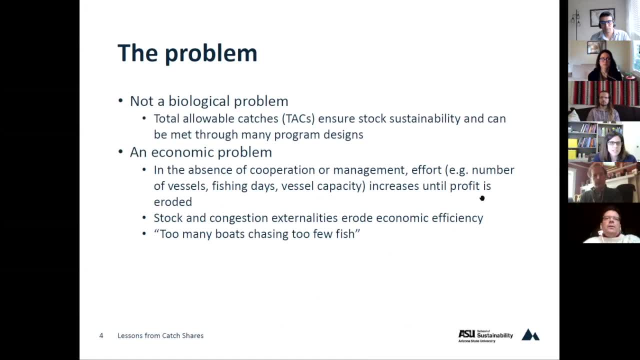 here. So when I think of catch shares and markets in the fisheries context, I think the story is slightly different, because to a certain extent we can solve that biological problem independently or historically have looked at the biological or ecological issue independently from more of the economics of things. And so these total allowable catches can ensure stock sustainability. 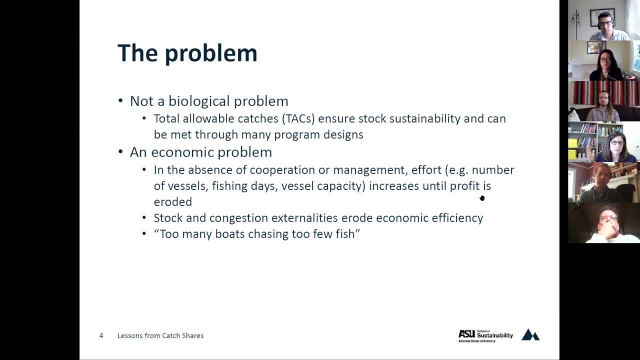 but they can be enforced with a variety of different program designs, And so one of the more common ones is that if you monitor dockside landings, you just have to be able to monitor dockside landings. So if you monitor dockside landings, you just 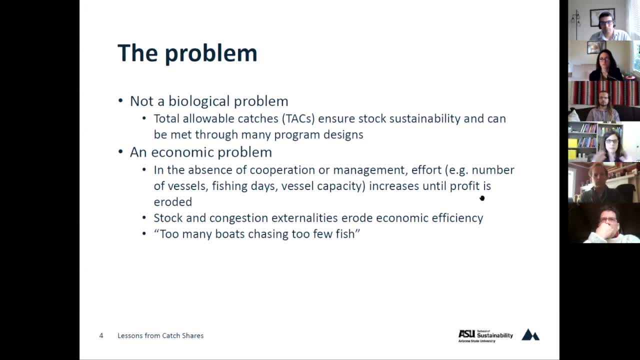 close the fishery down once the sustainable catch is hit: no more fishing. That doesn't solve the economic problem, but certainly it has the capacity to sort of separate these two dimensions. And so when I think of why would you implement an ITQ or a catch share, I think of that as more resolving. 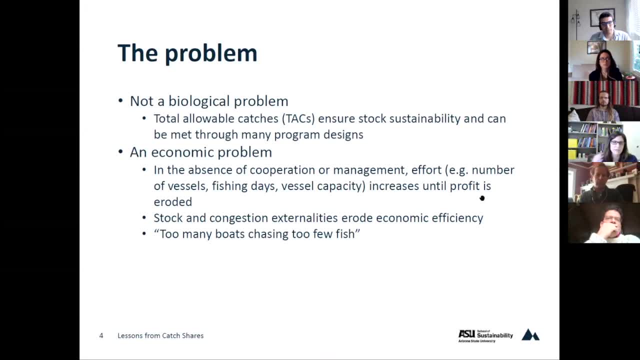 an economic problem. So in the absence of some kind of cooperation or management, we end up in this situation where we have too much effort. So in the fisheries case I think effort is multidimensional, So it's a little bit more challenging to think about in some ways. So we 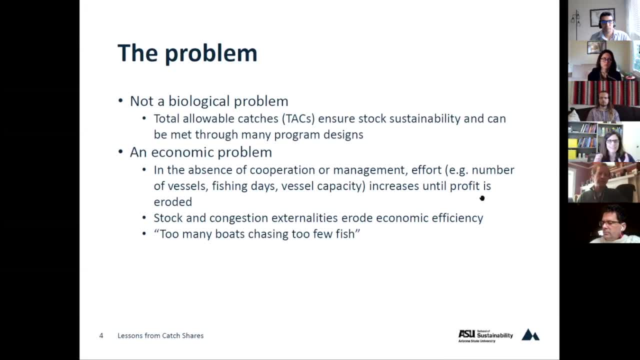 think of the number of vessels, fishing days, vessel capacity, So that effort is going to enter the fishery until profit is eroded. And so in the fisheries context- I think there's some nice analogies here to the water context- One of the big issues is the stock externality, And so 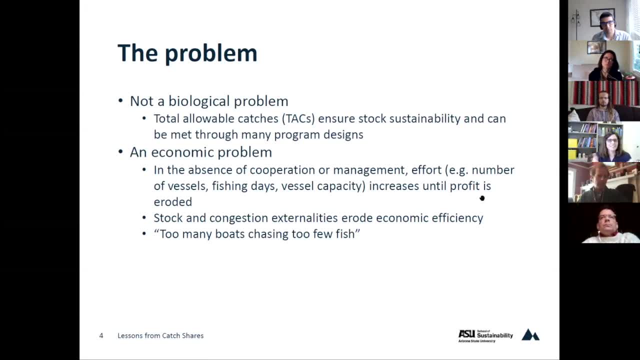 you don't own the fish. you don't own the water until you're using it, until you've got the fish on board, And so you don't own the water until you're using it. And so you don't own the fish until you're using it, And so you don't own the water until you're using it, And so you don't. 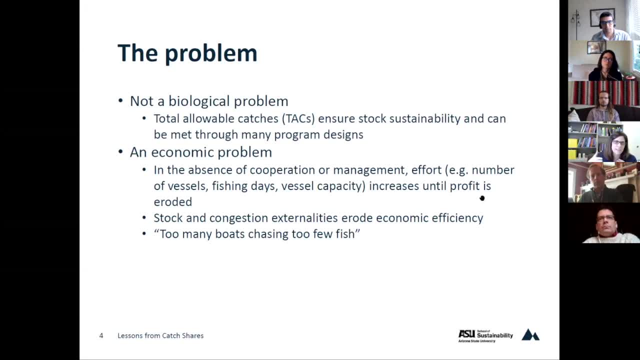 fish, because if you don't fish that fish, your neighbor or somebody else out there is going to pick up that fish. There's also the issue in some fisheries where the cost of fishing depends on the sort of density of the fish stock or the number of fish out there, And I think there's the analogy. 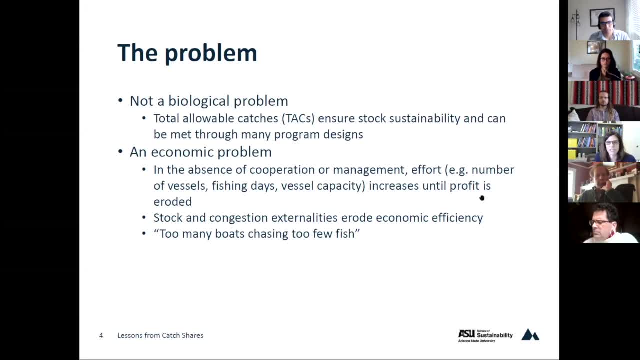 to groundwater and the pumping costs as the levels change. And so without management, without some kind of cooperation, you end up in a situation with, you know, eroded economic profit and potentially, you know you're going to end up in a situation where you're going to end up in a 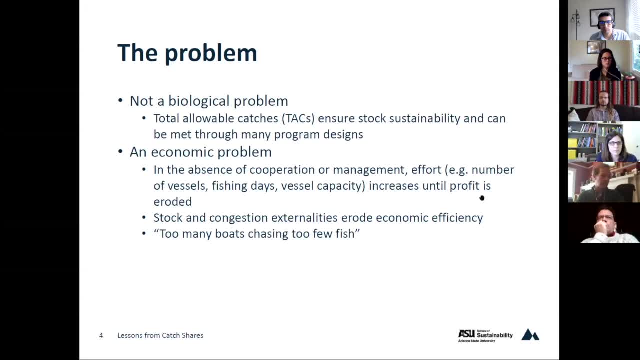 potentially, you know you're going to end up in a situation where you're going to end up in a stock issues as well, And so this is the sort of common pool resource problem- the too many boats fishing too few fish problem- And so ITQs are one way that we can tackle the economic as well as. 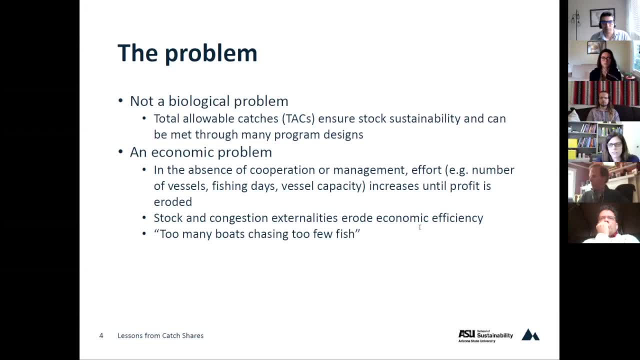 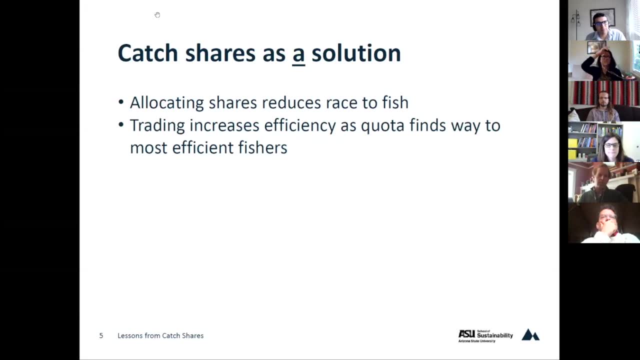 the biological, the biological challenges here. Thank you, Kelly. And what is the history of cashiers as a tool to manage fishers? Yeah, So I guess I it's. I've got, I think, one or two more slides that may bridge these. these couple of questions. 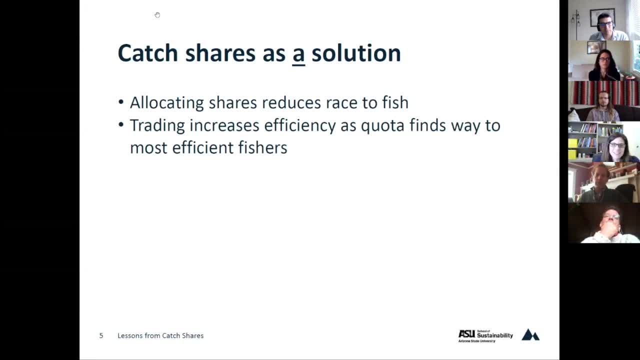 here. So let me just touch on this really quickly And I think Arthur was talking about this a little bit. So, allocating the shares, you can get rid of the race to fish or, in the groundwater case, you might resolve some of the common pool resource issue, but without that trading. 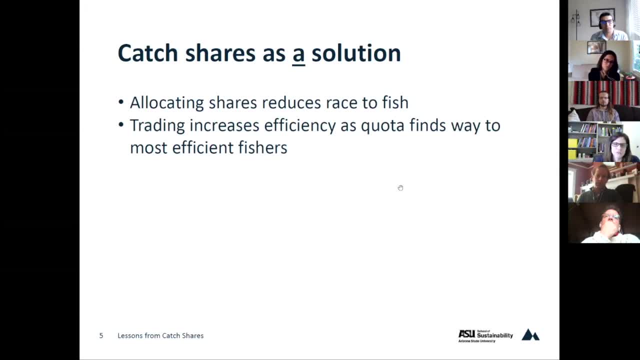 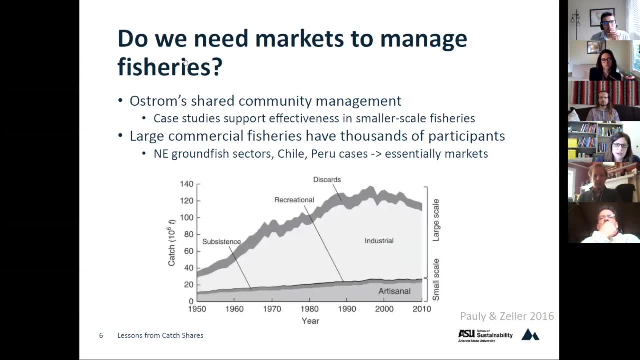 I think you don't get the full efficiency gains, And that's true for the fisheries cases as well. And then I wanted to just touch on this question that I think is also very important, as we think about porting over some of what we learned to the SGMA context, and that's do we actually need? 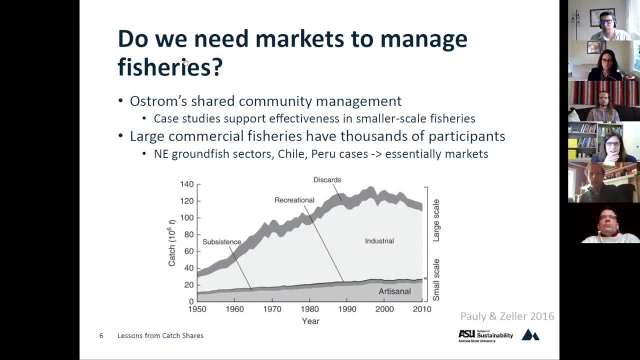 markets to manage fisheries And you know when you look at a lot of Ostrom's work and some of the case studies, there's a lot of support for shared community management as an effective strategy, especially in small on a scale fisheries. And so I can see in in ground water contexts where the community is much 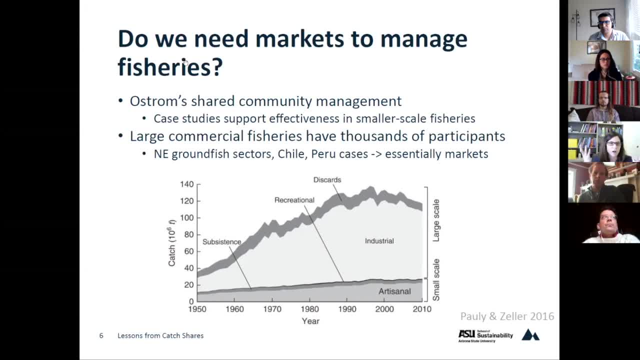 smaller, maybe you don't need the infrastructure of a market, And so one of the things that we see in fisheries is this kind of bifurcation. So a lot of the small scale fisheries contexts are these great examples that are more shared community management. But then we see a lot more. 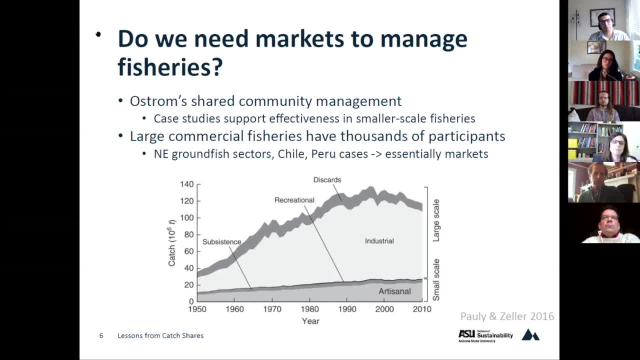 of the market-based programs, the ITQs in these cases. where have large commercial fisheries? So a lot of the work I do, a lot of the fisheries that I look at. there are thousands of participants And so in cases like that it's a lot harder to think of. 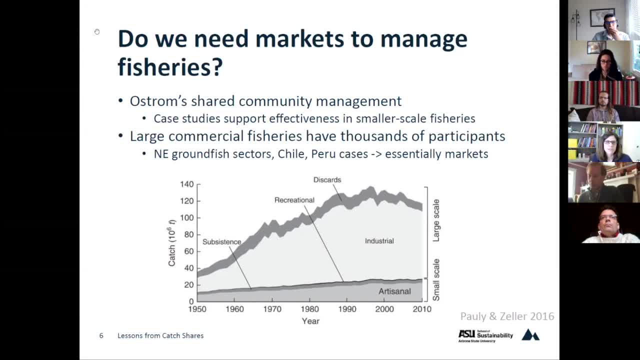 how shared community management could really work. So there have been a number of programs as sort of a backlash, I think, to this market approach. We call these catch shares now a little bit in the US as a backlash against the ITQs. So there have been these sort of more combined. 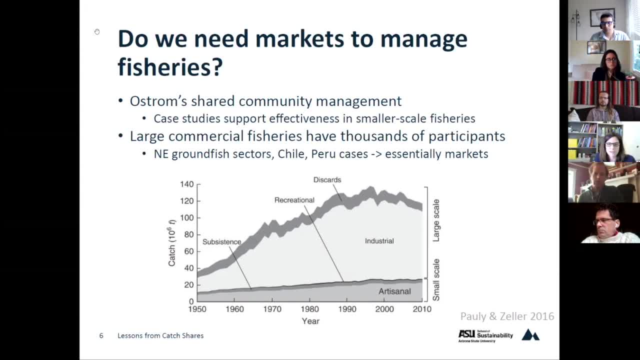 kind of programs. There's the Northeast Ground Fish Sector Program, There's a couple in Chile and Peru. And what these programs did? they're a bit of hybrid in the sense that the aggregate cap is set, Fishers are given an allocation if they want to join the sector or this cooperative. They bring their allocation After property is imported from the fishies that they were in, and then that sector or cooperative can decide how to use that allocation. who would fish it? So if you value equity, if you value specific communities, you can push that allocation there. And what's happened? 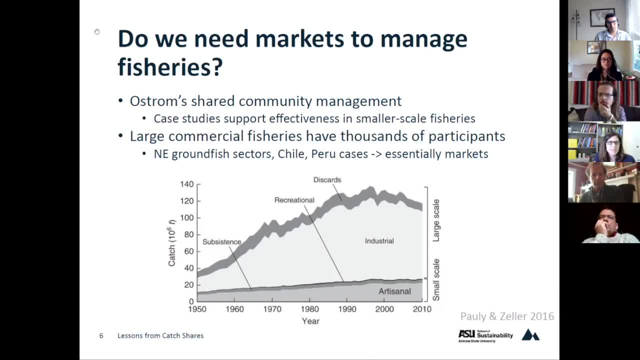 though, again and again, if you actually go and talk to participants in these fisheries, is that they've essentially created mini markets And so it's a little bit more devolved, more decentralized, But effectively of the allocation is moving within these sectors or cooperatives in more of a market structure. 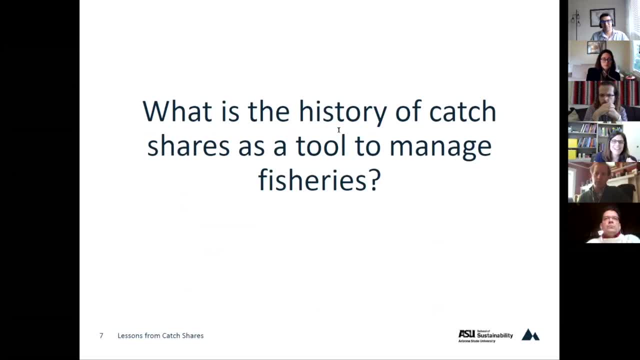 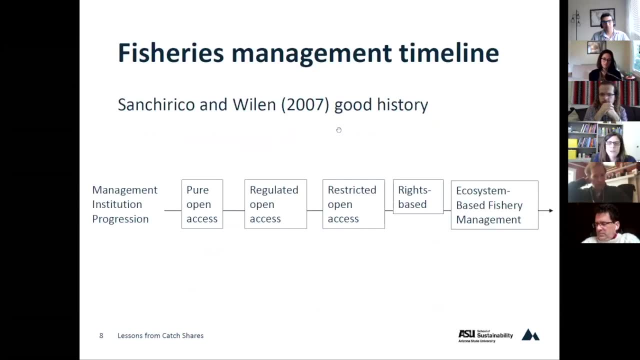 So now I think, Maddie, I'm going to go ahead and get into a little bit of the history here as well, And I think this will dovetail nicely with some of what Arthur was talking about. And so the history of fisheries, I think, is a little bit different in the sense that 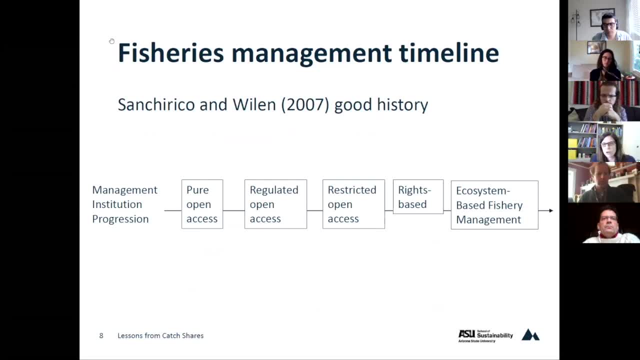 you know, historically there were the pure open access fisheries, no regulation at all. But then there was this move and sort of ecologists made this really persuasive argument: We've got to manage these stocks sustainably if we're going to have productive fisheries. 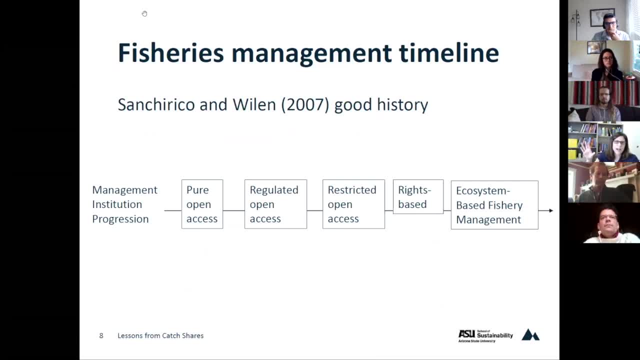 in the future. And so this is where you get into the regulated open access management regimes where the catch is capped and the season might just be abbreviated. You shut down the fishery when the cap is met. There's these other, more intermediate type of program. 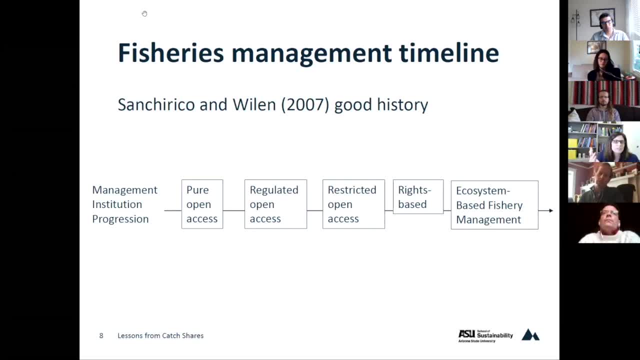 restricted fisheries, Open access, where you restrict who can enter the fishery. And then we think of our more kind of traditional rights-based programs. The last sort of management institution progression, or last management institution that I've got up here on this progression, is ecosystem-based. 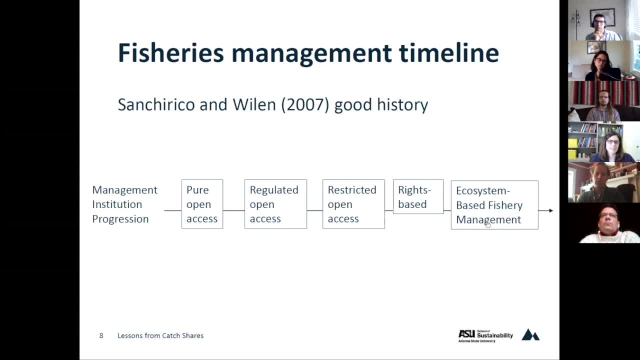 fishery management, which is more of a new way of thinking. Just over the last few years, I feel like this has really been pushed And so you can think of. you know, going from the pure open access to the rights-based, you're sort of moving along this property rights spectrum and increasing the. 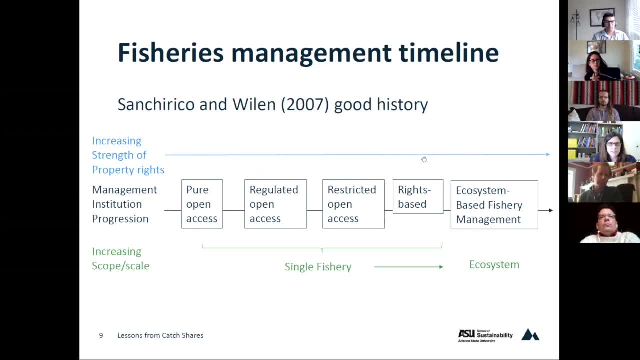 property rights. But then, more recently, we've really been thinking in the fishery space about expanding the scope or the scale of the management programs that we would use, So moving from beyond just a single fishery to more of an ecosystem scale, And I'll give some examples of that. 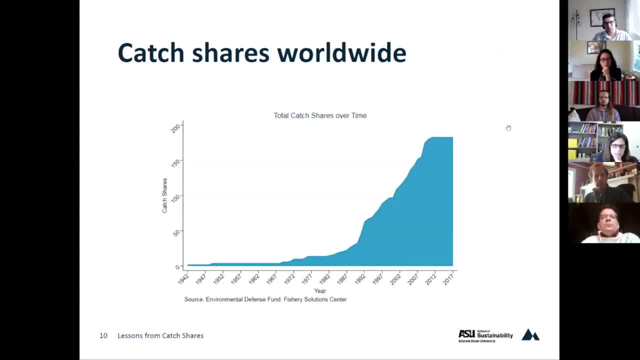 later on. So yeah, So in terms of the history worldwide here, and when these programs came into place- really in the 70s, I would say- a lot of catch shares started to take off, And this figure here ends at 2017, I guess, But you know, I'd say at least around 200. 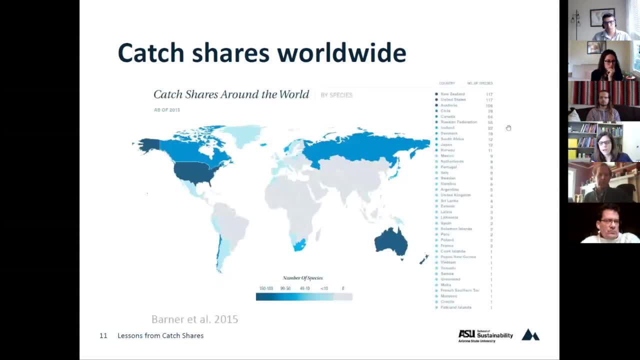 programs are in place worldwide today And across a range of different countries. So this is sort of counting the number of species by country And you know, one of the trends here you might see is that these tend to be implemented in more developed country context. 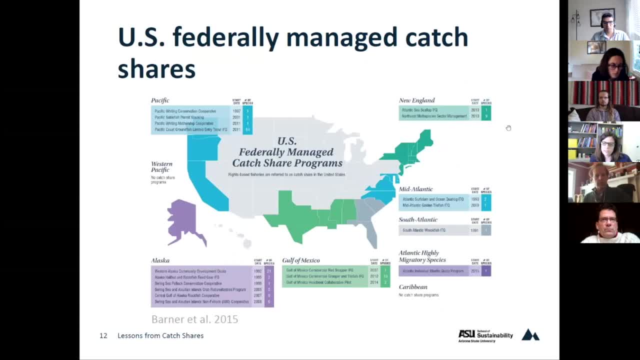 And then, finally, I just have a figure here showing that these are implemented in a variety of fisheries around the United States And, looking through this list, I would say most of our, or many of our- higher-value fisheries in the US are managed via catch-share, And that's really a big part of how we're able to manage our 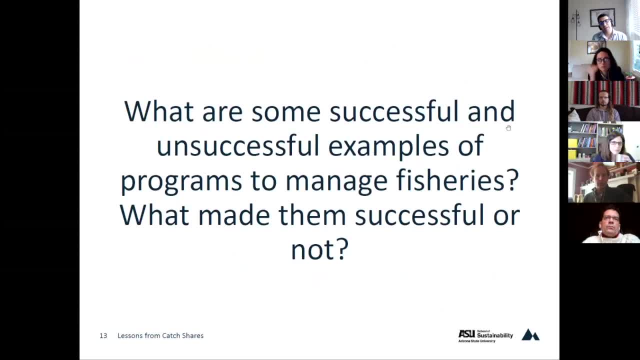 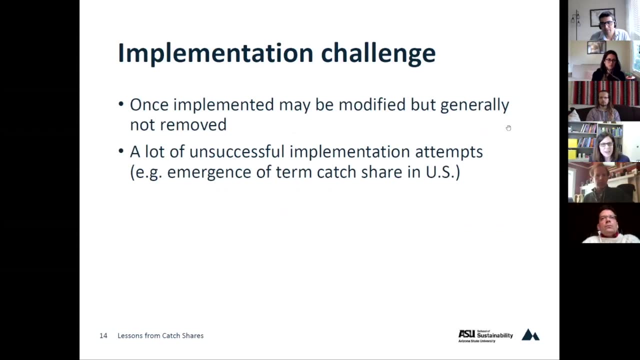 shares. Thank you very much, Kenyan. And we have the question here: what are the some of successful and unsuccessful examples of programs to manage fisheries and what made them successful or not? Yeah, let me jump in here. So I reframed this question a little bit because I think in the 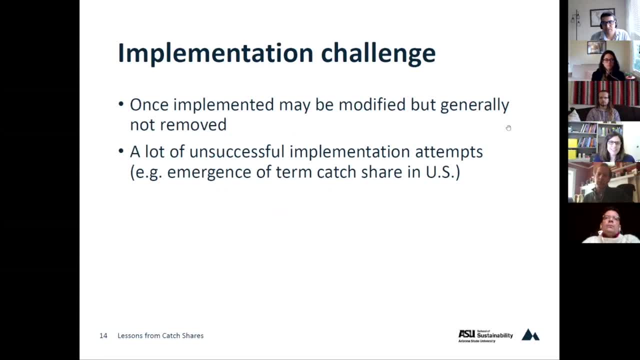 fisheries case. this is more a story of implementation, And so I wouldn't say there's been a program, or at least it's very rare for these programs to be, say, so unsuccessful that they're removed. Generally they might be slightly modified once they're in place, but the real 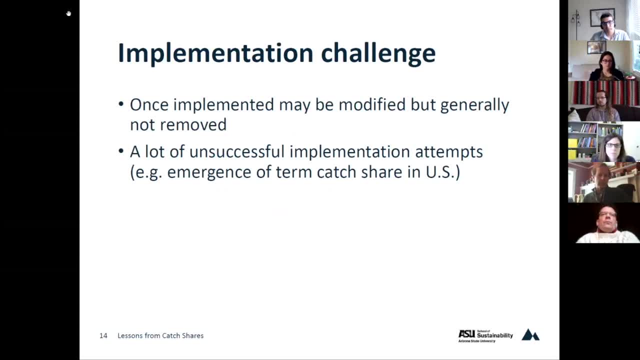 challenge is actually implementation, And so I gave a little bit of a history here, a few slides back, but this is one of the reasons we talk about catch shares instead of ITQs. There is some resistance to more market-based approaches By fishers early on and I think there one of the problems was not enough sort of stakeholder. 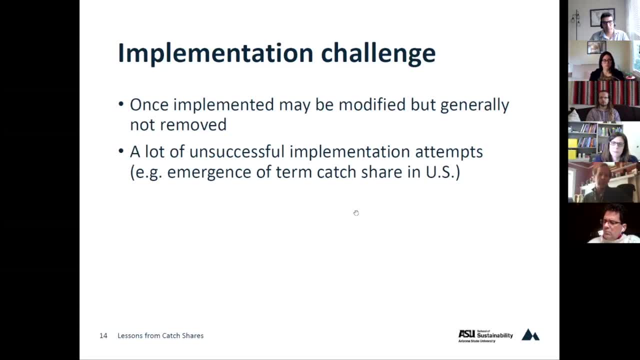 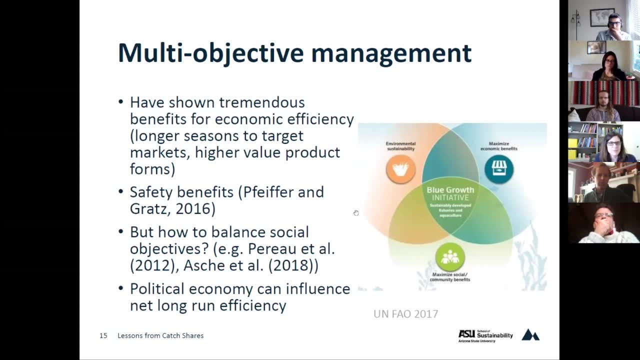 involvement in some of the program designs, But I think also incorporated in this word, success, is: what are your objectives? So, to measure the success of a program, I think we need to be really clear and articulate about what the objectives of the program are. And so, as 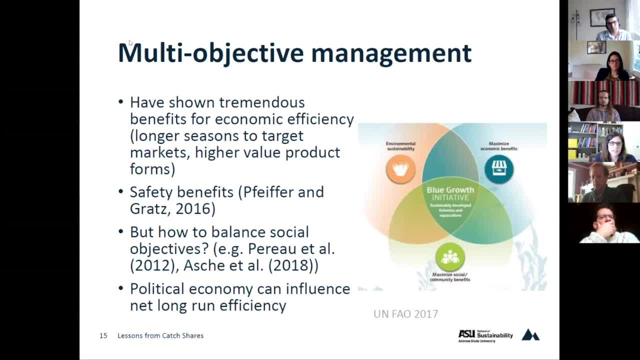 economists, I think we are prone to thinking of economic efficiency. But if you go through fisheries regulations and you all can tell me more about the water context, the objectives of management are not just economic efficiency. So we sort of have this tool that is designed very well. 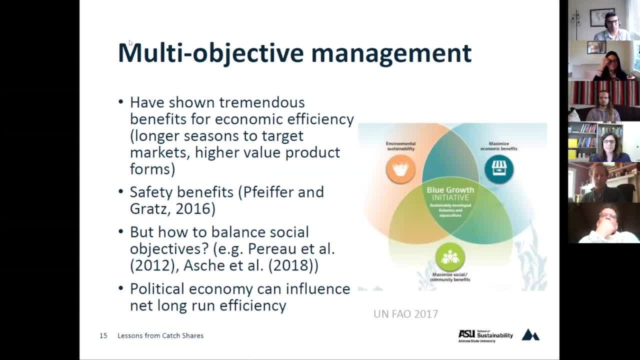 in terms of addressing economic efficiency, But then, in reality, a lot of the goals of fishery management programs go beyond that, And so there are a number of papers- economists, I think, have done a great job- showing that these programs have tremendous benefits from an economic efficiency. 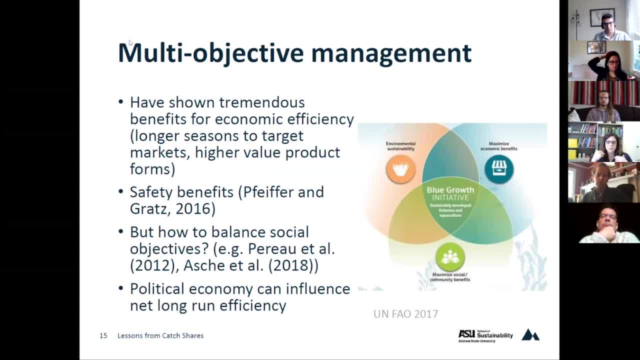 perspective. We've seen seasons elongate. Fishers can time their catch to win the market. The price is high. It also has opened this opportunity of switching product forms. So maybe some of these programs or fisheries used to stay open for just a couple days, like the halibut up in Alaska. 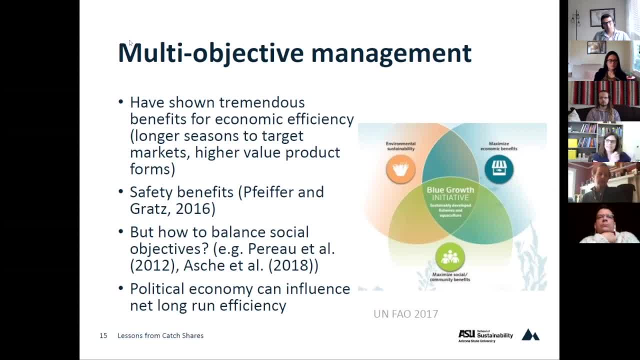 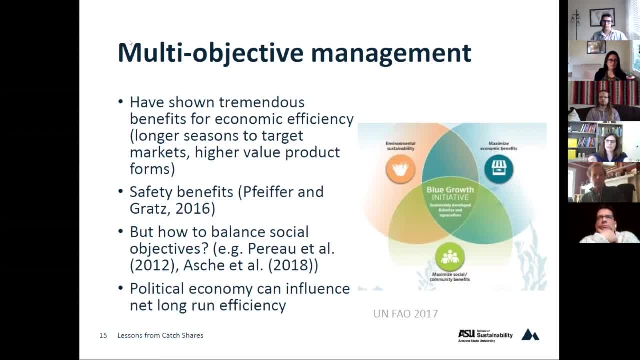 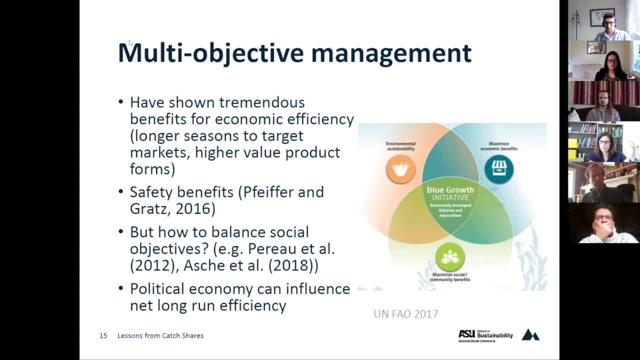 And after the ITQ program went into place, then there's the option to sell this higher value sort of fresh producti are quite different share and every year you're missing out on, you're missing out on the the sort of profitability of each of these years. 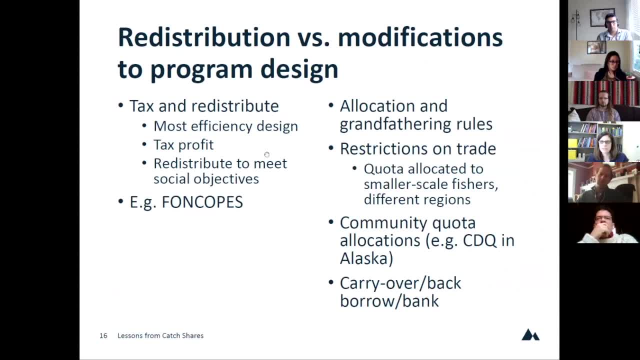 And so some of what's been talked about and operationalized in the fishery space relates to, well, what can we do to try to balance these different types of goals within this program structure, program structure? and so I think the first is the sort of obvious one. 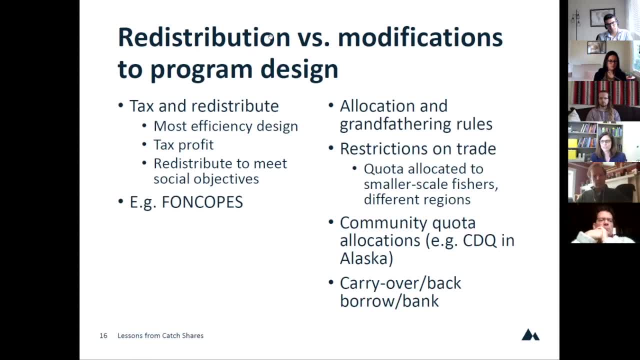 One too. The first was changing î pants in the years and showing off the 2022 aquaculture activity to economists, which is redistribution. So design the program to be as efficient as you can: tax the profit and then redistribute it to meet your social objectives. So, in the fishery space, if 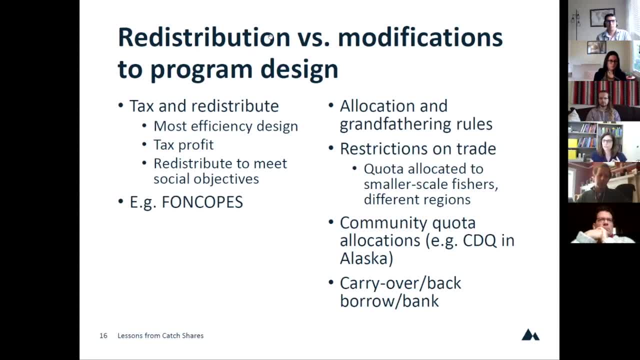 it's community well-being if it's keeping small-scale fishers in the fishery. you know what are the concerns that are sort of tied to that. And in the case of this from COPE's program in Peru, some of what they did was allocate some of that tax to retraining retirement incentives. 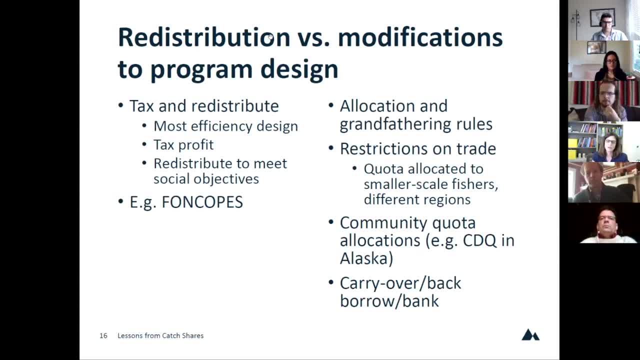 and things like that, to try to sort of ease the transition into this new program structure. That's relatively rare, though A lot more common- and I think this might line up with some of what folks are thinking about in the SGMA space- is modifying the program design itself. 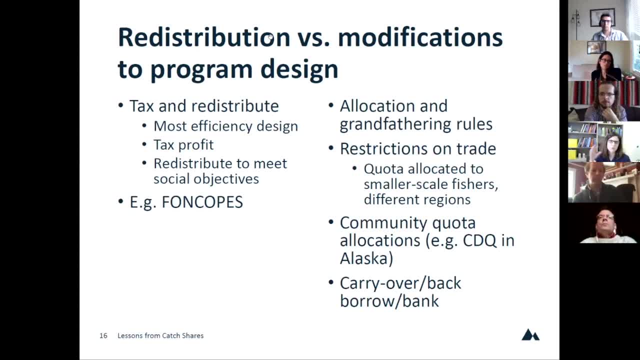 So who's allocated allocations, Sort of? what are the rules around that? One of the things we see a lot in the fisheries context is restrictions on trade. So quota or the allocation is given maybe to small-scale fishers, to different regions. That's something that I 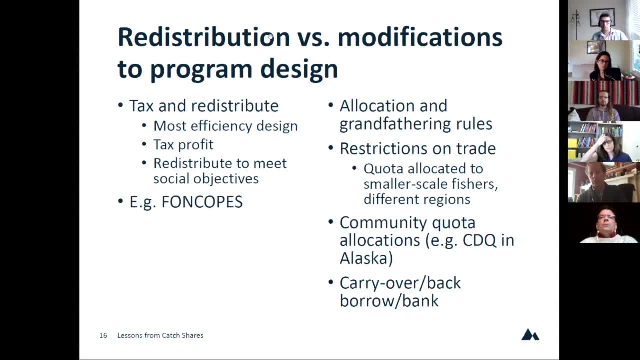 think I heard Arthur talk about in the SGMA context. There's been allocations to communities themselves and then there's sometimes some additional flexibility built in. So maybe can you go over a little bit one year and then pay it back the next, or vice versa. 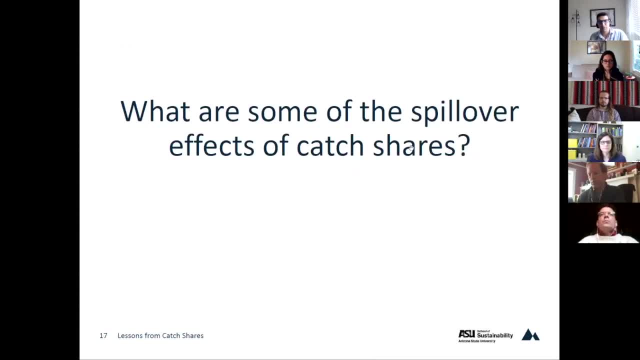 Wow. Thanks, Kellyanne. And what are some of the speedover effects of cash shares? When we talk about SGMA, this question comes up a lot. Yeah, I think this is a really interesting one, and it's interesting to me. that's something that 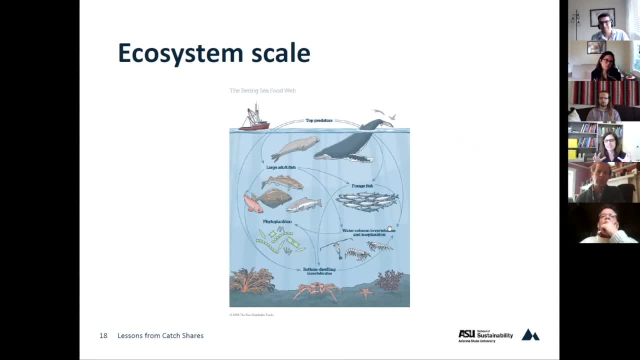 you all are thinking about in the SGMA context, because I feel like this is something that we're just thinking about recently in the fisheries space, And this was sort of motivated first by ecologists who have this more systems approach to what's happening under the water. 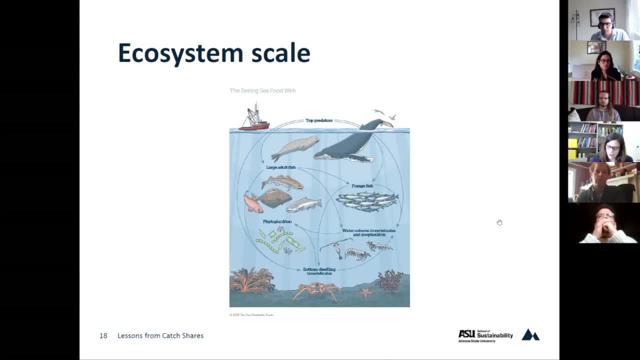 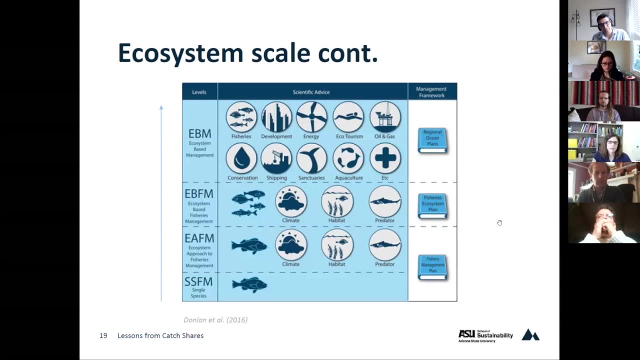 and thinking about sort of a food web, And there's been this push to sort of increase the scope of management program design and evaluation. And so when I show those other slides, a lot of showing the cash shares that have been implemented in the world, a lot of them are single fishery specific. 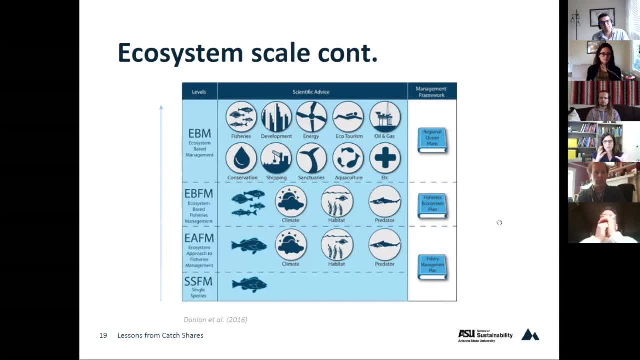 So the Alaska Halibut, for example. So that would be specific to a particular fishery, But now there's there's this push to think beyond just one fishery, to think more at an ecosystem scale and acknowledge some of the connectivity that exists between these different ecosystem. 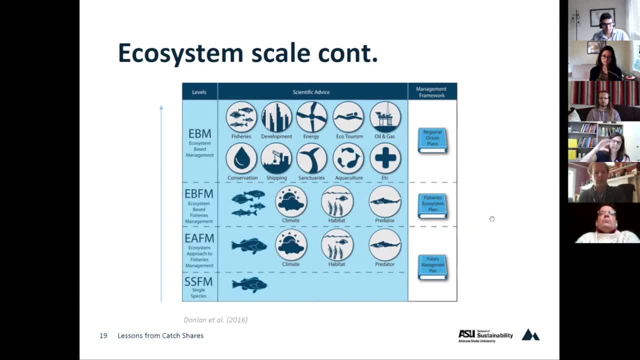 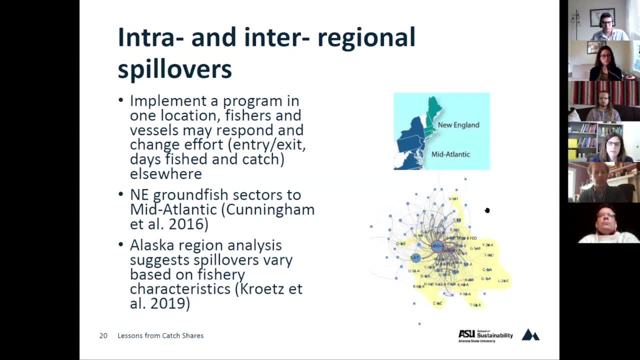 components and then sort of segmenting that into more ecological and human there, And so some of the work that I've been involved in has looked at this question, And so the basic idea is that you could implement one of these programs in a particular location. 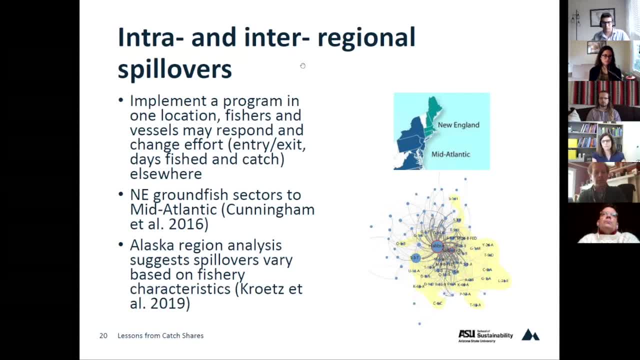 a particular target fishery, that fishers and vessels may respond and change their effort So they might exit and go somewhere else, They might increase the day's fish, they're catching another fishery And so you might be thinking: well, you know. 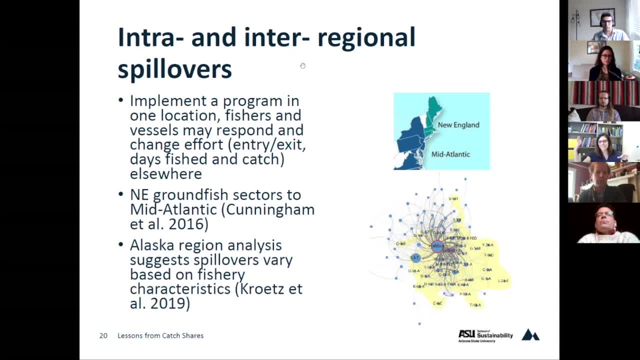 I did a great job in this particular fishery, increasing economic efficiency or whatever your goals are. But maybe you're generating this externality somewhere else, And so you've essentially resulted in effort shifting into another fishery and maybe decreasing the economic efficiency or sort of creating another issue over there, And so this: 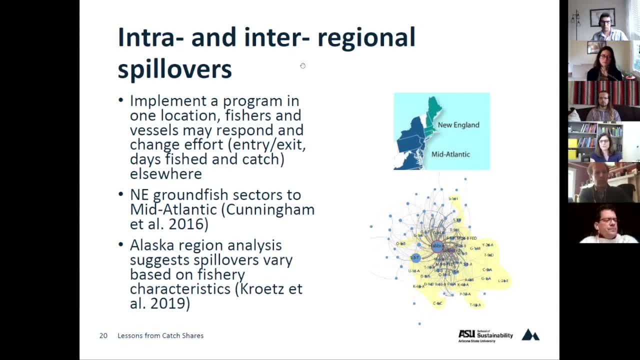 is the sort of idea of spillover that's emerged in the fisheries context, And so there's some work by Marty Smith and some co-authors showing that spillover happened with the New England ground fish sector program. So from sorry. 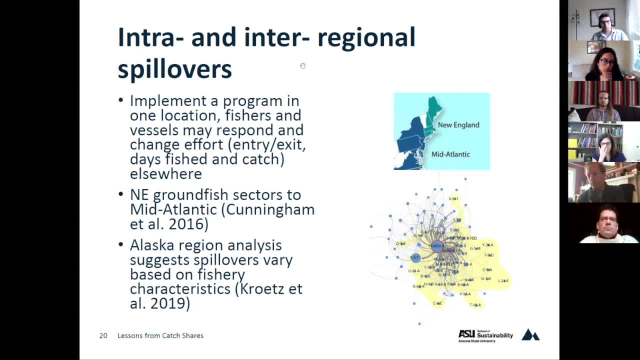 from the northeast down to the mid-Atlantic region, And then some of my own work. we looked in the Alaska region after these catch shares were implemented. What we saw was that, depending on the fishery characteristics, there was sort of more or less of this spillover. 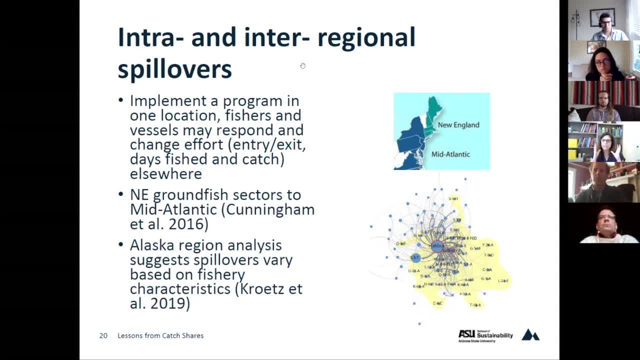 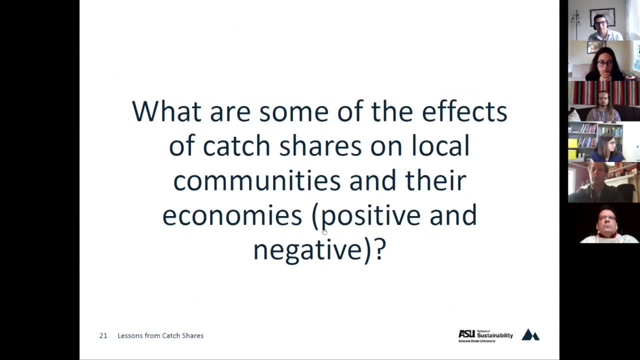 but that indeed these fisheries are connected And so, looking on just sort of a single fishery basis, you may be missing some really important externalities and potential efficiency gains. Thanks very much, Kellyanne. That's in line with what we are thinking about. 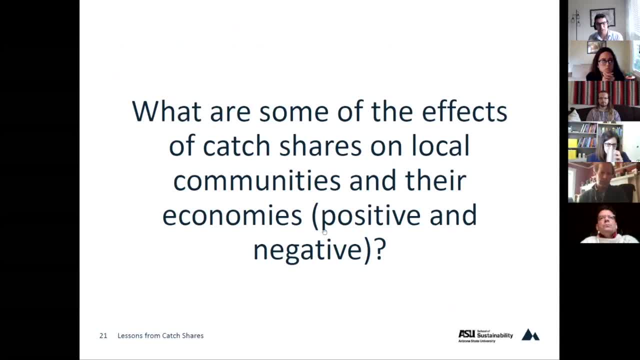 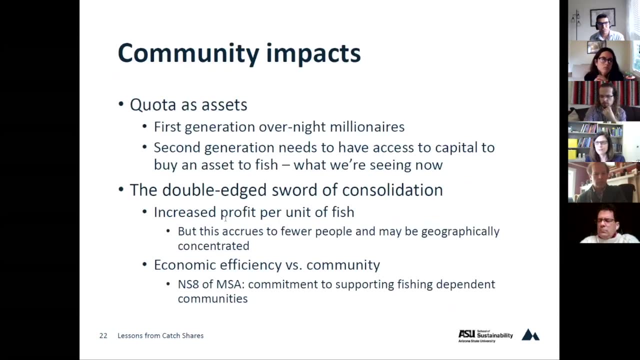 SGMA And same here. when we talk about designing groundwater markets, there are talks that can have a positive or negative effects on local communities. What do you see? these effects are in catch shares. Yeah, So one of the big first things is that these- we call them quota in fisheries, but you 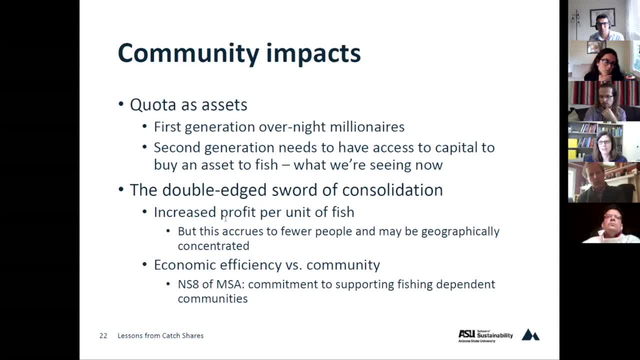 get that initial allocation and it's an asset. And so there's that sort of first generation and we heard this in Peru a lot when we visited and were evaluating their catch share program there Overnight. there are millionaires in some of their communities. This asset is worth a lot. 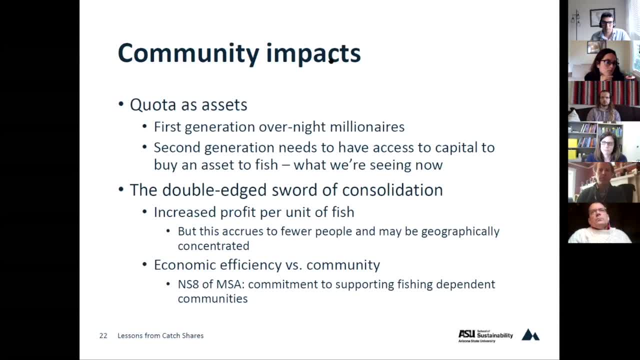 and fishers can sell it And you know, it sort of really changes their personal portfolio. But then some of the challenges arise and we're hearing that a lot now in the fisheries context or remember these have been in place since the 70s, 80s and a lot there's that kind of huge. 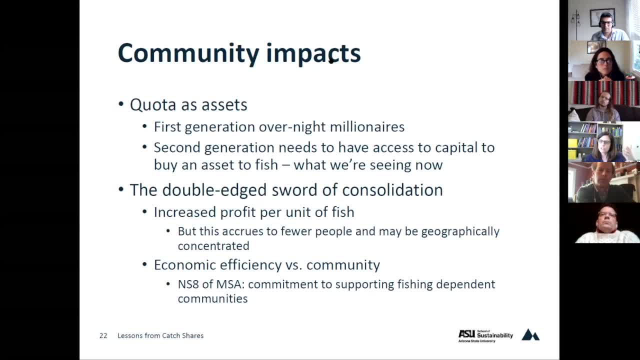 spike in the 90s. And so, as this new generation of fishers is weighing whether or not to, or new generation of potential fishers is weighing whether or not to fish, now we've run into this problem of fishers needing access to capital to buy an asset- to fish, And so what does that really? 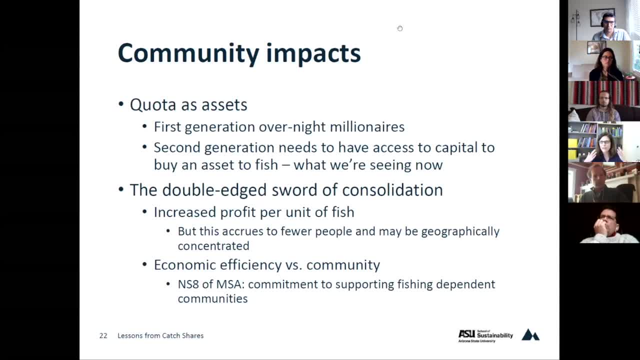 mean in terms of who has access to this fishery. So it's got to be somebody that has access to capital or can at least get a loan or something, And so I think, from an equity perspective, that's raising some flags for folks. I think the other thing that's really important to think about 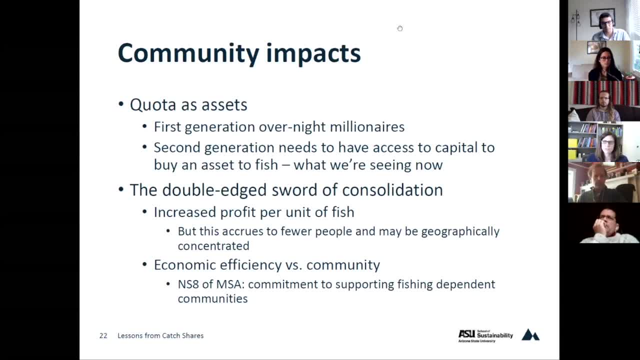 from a community impact perspective is this sort of double-edged sword of consolidation, And so, as we remove excess capacity and effort from the fishery to make things more economically efficient, what we're actually doing is we're taking and changing the nature of fishery labor across these. 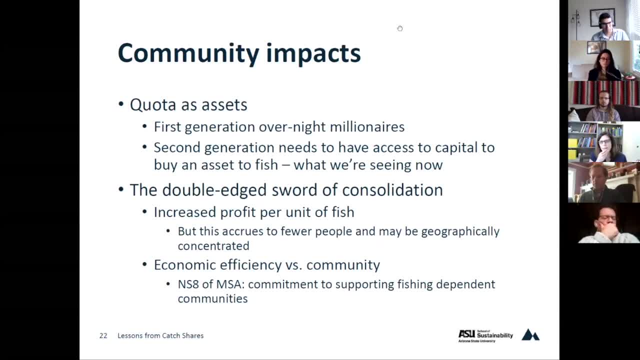 communities, And so, yes, we're increasing the profitability for some, but these may be very geographically concentrated And so there may be some distributional aspects to think about across the fisheries or across the fishing communities, And I think this can really be framed as this sort of economic efficiency versus 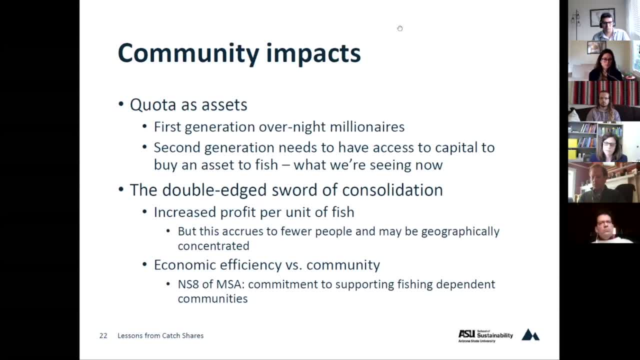 more kind of community well-being trade-off. in many contexts, And here in the US in the fisheries space, we're pretty explicit. national standard of the Magnuson-Stevens Act commits us to supporting fishing dependent communities, And so we're supposed to be thinking about those communities. 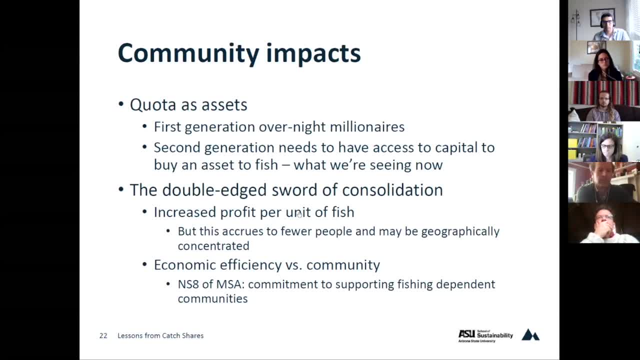 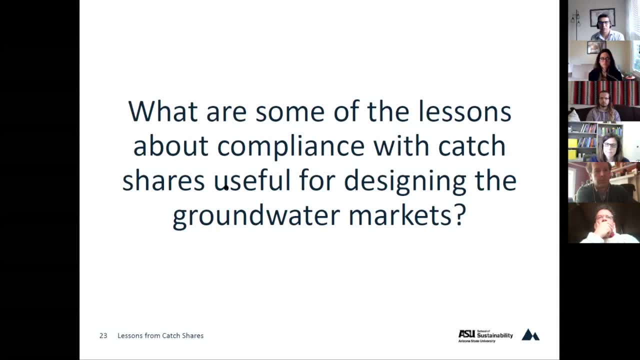 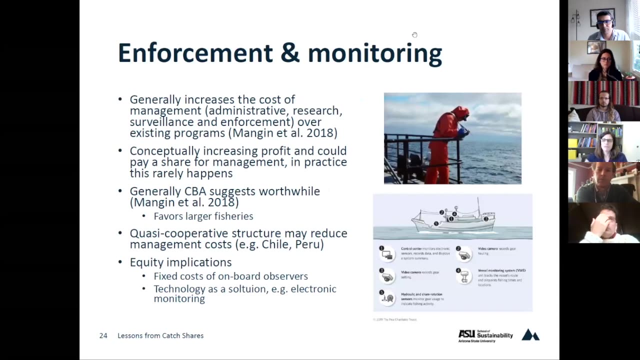 when we make management policy design. Thanks, Kalyan. And what are some of the lessons about compliance with catch shares that are useful for designing groundwater markets? Yeah, So one thing that we found in the fishery space is that catch share programs do tend to increase the cost of management. So you can think I mean. 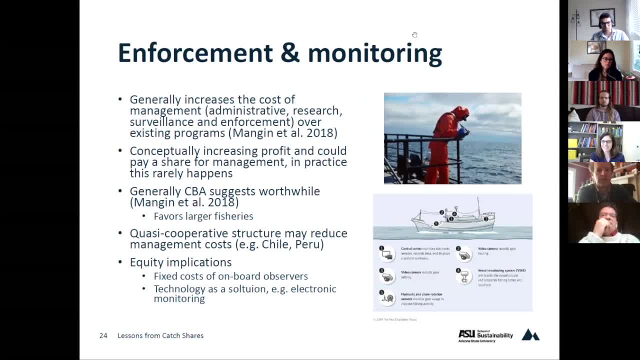 somebody has to do that sort of catch quota reconciliation. Someone's got to keep track of all this stuff. So there's sort of the administrative side. There's the research side. How do we design these programs? How are they working? We need to understand that And 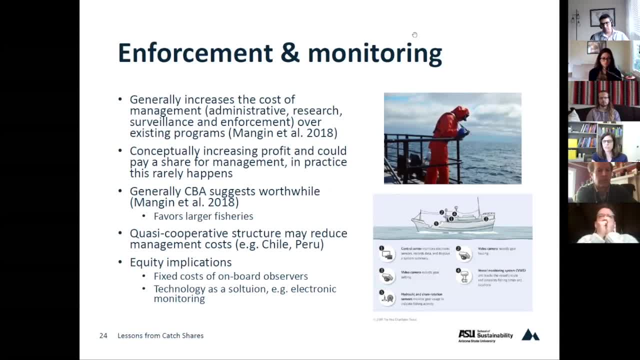 then there's the sort of day-to-day surveillance and enforcement, And so you know, conceptually you're increasing profit, But I think a really important part of that is that you're increasing cost. And so the question is, you know, does this cover the management costs And generally? 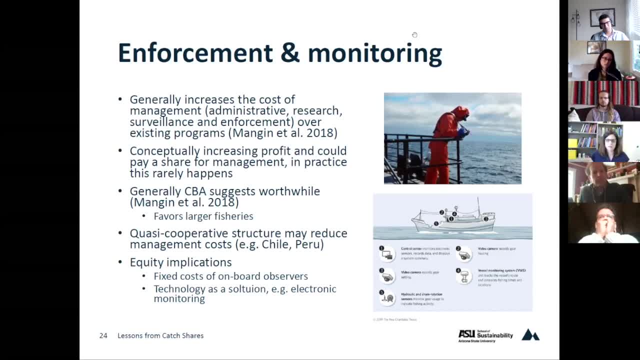 if you looked at this from sort of a cost-benefit analysis framework perspective, yes, it does. But I also think it favors larger fisheries, And this is back to an earlier slide where I kind of drew that contrast between some of the smaller scale fisheries where I think a lot of 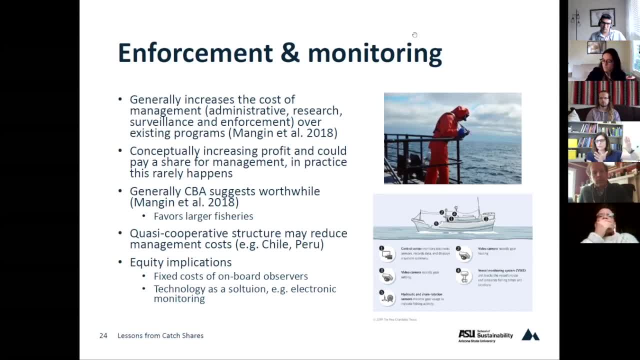 the Ostrom kind of work is really relevant, and then some of the larger scale commercial fisheries where I think markets are a better fit, And you know, one of the reasons is this here, One of the other things that I heard when I visited Chile and Peru and was talking about. 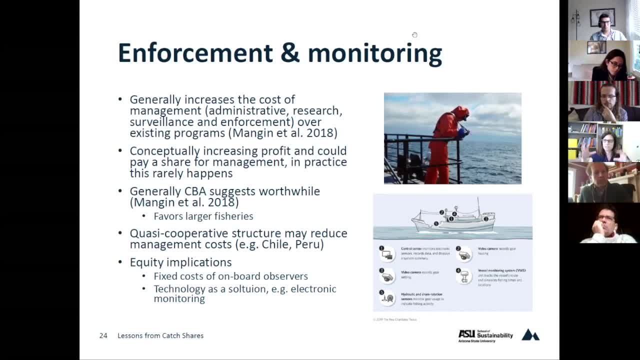 their program. they have something similar to the Northeast sectors. It's this kind of hybrid where the participants join these cooperatives, And so one of the advantages we heard was that all the movement of quota or allocation within the cooperative it was managed by the cooperative. So there's that kind of devolved administrative cost. 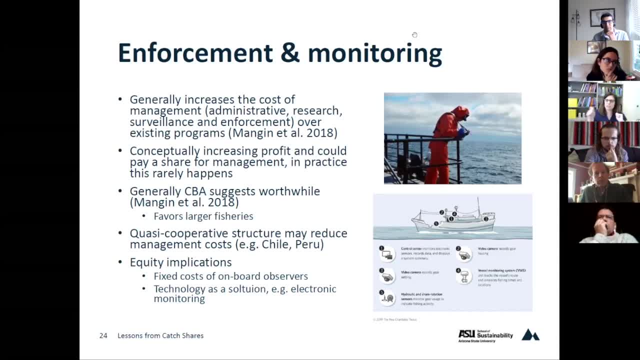 And then the government tracks just the aggregate and trades between these different groups. So I think that's something to think about. And then the last thing I want to flag on the enforcement and monitoring side is the equity implications, And so I've got some pictures up here, A lot of the enforcement and monitoring in these. 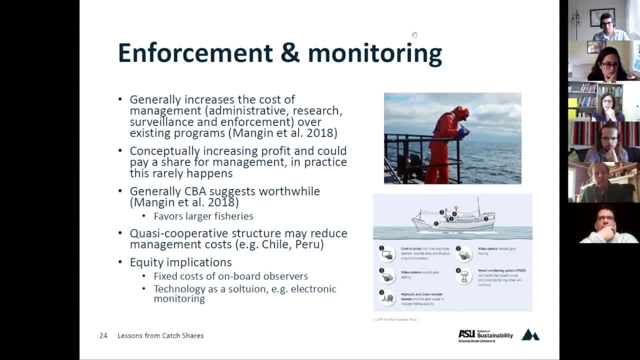 early catch, share programs and just fishing in general. in the US they have a fixed cost of onboard observers And so the first generation of this kind of enforcement and monitoring is someone physically goes on the boat and watches, as you said, to pull up your catch. But if you can think about, you know a really small boat versus a really big. 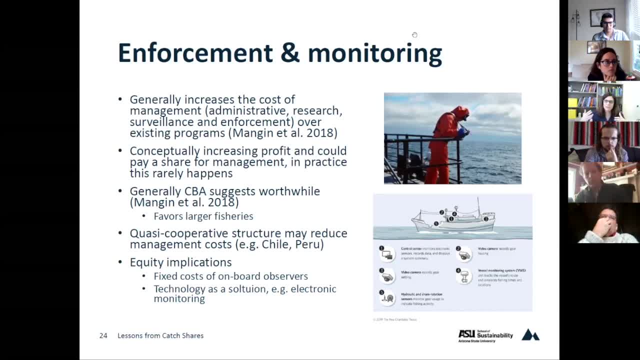 boat. you both just need one observer usually, And so that kind of fixed cost really favors larger boats, larger operations. And so in the fisheries case, technology has sort of emerged in that direction, And there's electronic monitoring options now where there's cameras. 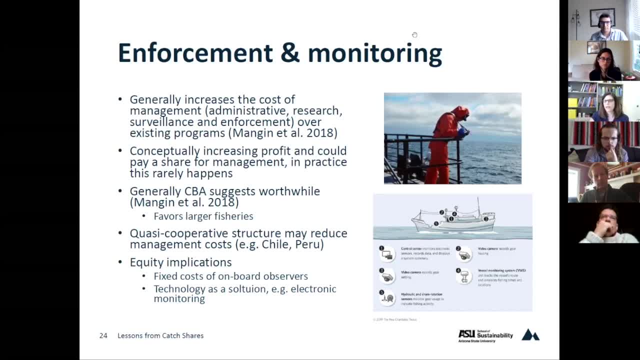 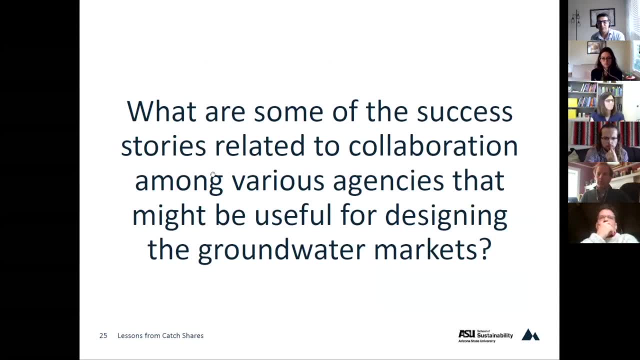 that are motion-censored, that when you go to pull the catch up will monitor it. Thanks, Kenyon, These are very interesting. And again, when we talk about designing groundwater markets, we talk about collaboration among agencies. Can you tell us some of the success? 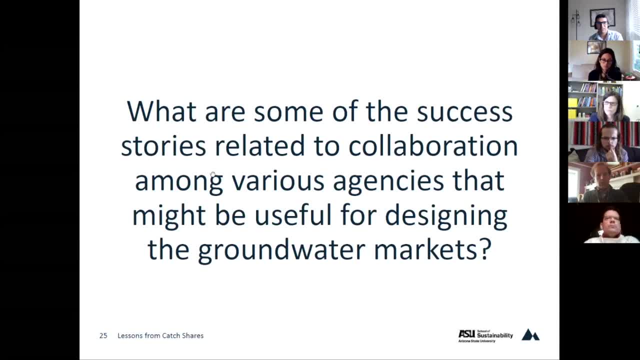 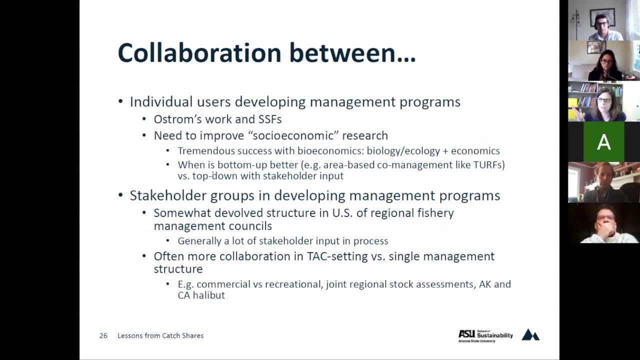 stories that you have from fisheries markets. Yeah, Here I wasn't able to find, I think, as great parallels, I think, to the water context as to some of your other questions. But the way things tend to work in fisheries is that you know you can have this bottom-up management. This is more the Ostrom. 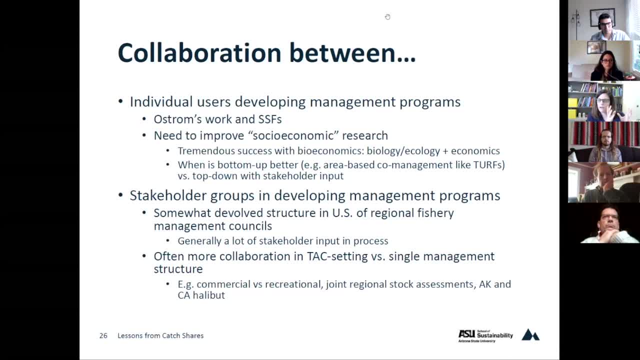 style. This could be brought about by individuals themselves. I think this generally is an area that we could really improve on. So you know, when I think of bioeconomic analyses, the list of papers is sort of endless, But I think we've done a lot less in terms of 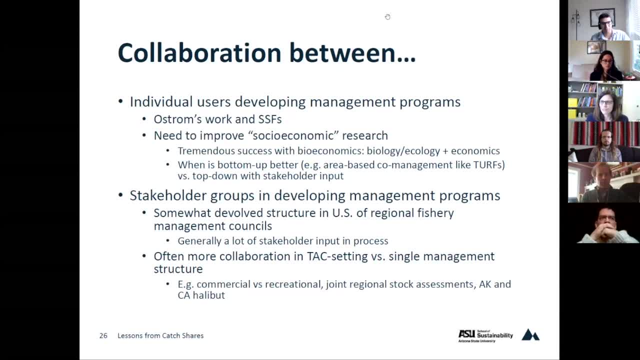 cooperation with other social scientists And so really trying to understand: when can individuals come together? how can individuals come together to implement this more kind of co-management type approach versus when? do we want to think about these more kind of top-down management approaches, And what we've seen in the US tends to be this more sort of top-down. 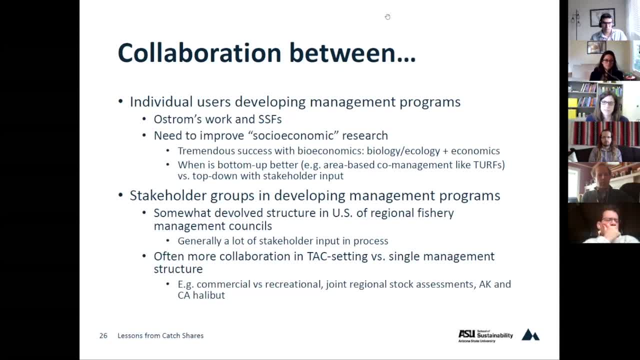 approach, especially in a lot of our more valuable fisheries, And so you know sort of segmenting things between, well, individual users can come together and collaborate versus. you know, here in the US I think the discussion more is around getting different stakeholder groups. 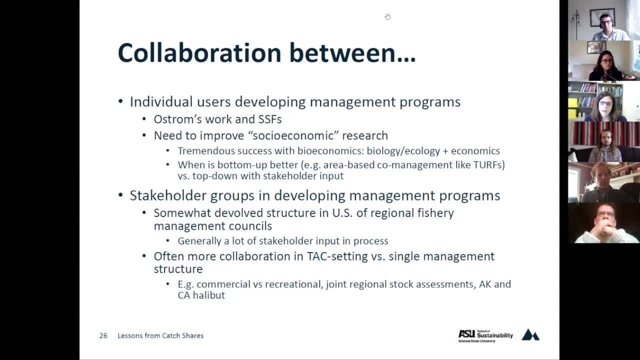 to the table and developing management programs, And so fisheries in the US is already somewhat devolved. So the US has a number of different regions and those fishery management councils are responsible for designing those programs And there is generally stakeholder input into that process and sort of a process that. 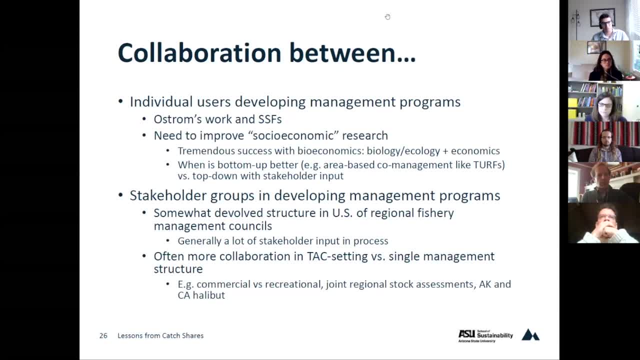 includes stakeholders there. But then you know, I think that as we look at species themselves, as we broaden this kind of scope of management, we can think about other cases where there would or maybe wouldn't be collaboration, And so certainly in the US. 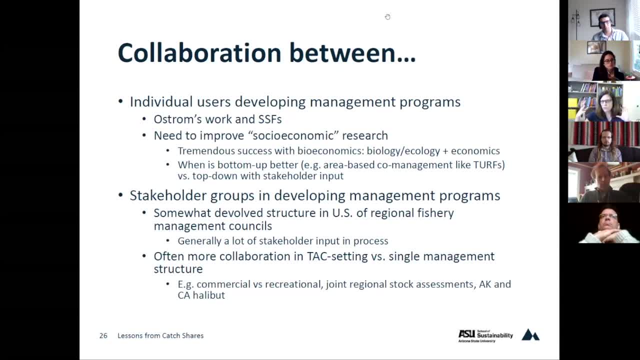 I see instances where you know the TA, the total allowable catch is set jointly between different sectors and maybe those are different types of stakeholders, so commercial or recreational. There's some collaboration between these different regional councils to undertake the stock assessments. And then I thought of you know another example, So sometimes countries- 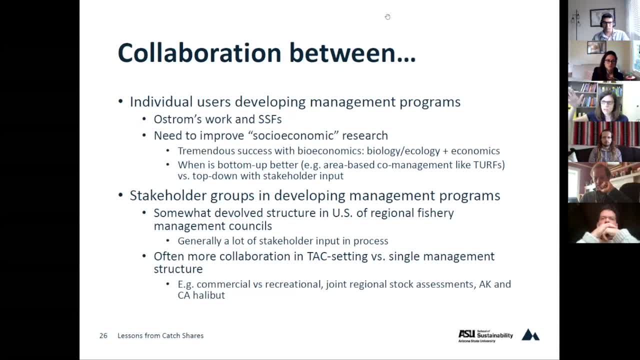 will jointly manage or assess the stock and allocate catch. So you know Alaska and Canada do that with their halibut. But overall this seems to be like an area where I just saw fewer parallels versus some of the other questions that you raised. Thanks very much, Kalyan. This was very. 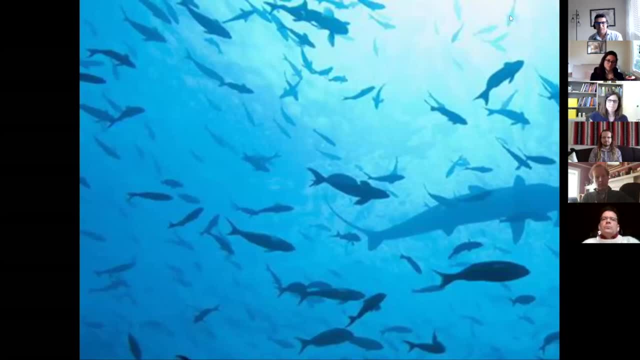 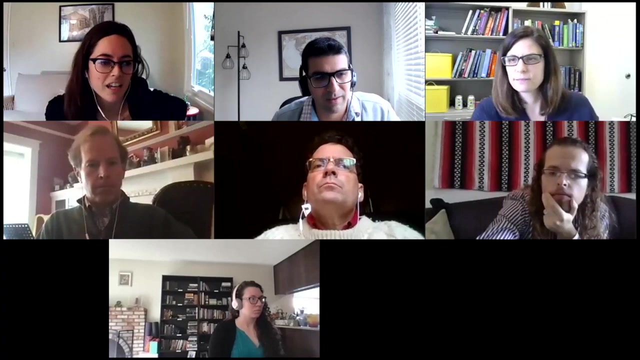 interesting, informative To all the attendees. if you have any questions for Kalyan, please submit it through the Q&A box on the bottom of your screen. Now I turn the stage to Ellen and Jamie for their discussion. Yeah, thanks, Mehdi. Thank you so much, Kalyan. That was really great. 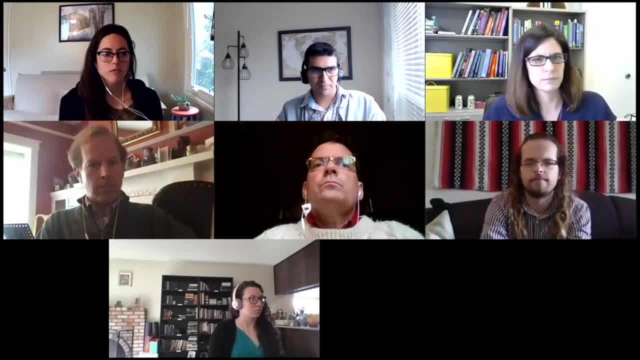 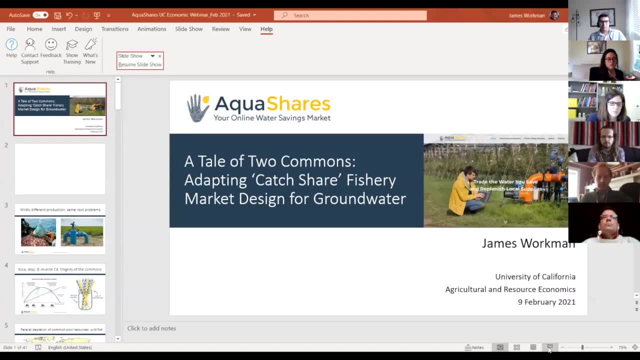 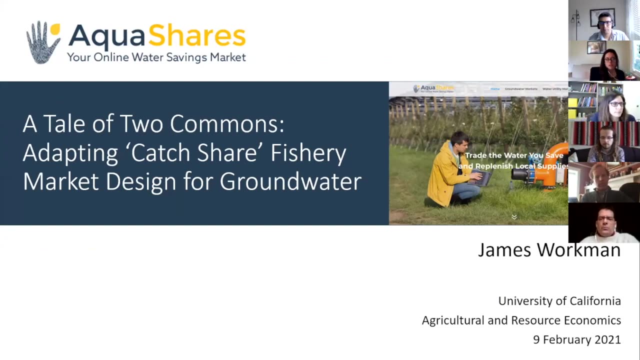 really informative. I think there are a lot of lessons we can take from fisheries and thinking about groundwater market design in California under SGMA, So really happy to have Jamie Workman here. Thank you so much, Kalyan, for being here with us. to talk about just that, Jamie, would you mind? 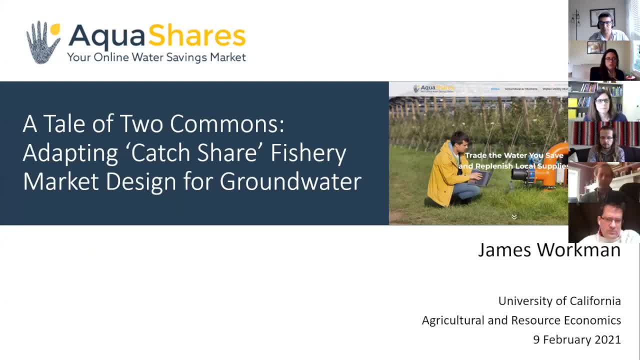 just starting with, like you know, high level, what is AquaShares? And we can go into some of the more details about AquaShares approach in a minute. But would you mind just giving us you know, telling us, what AquaShares is and then maybe kick us off with sort of telling from your point of view? 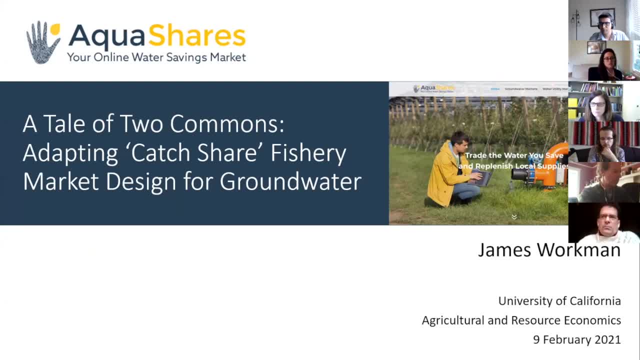 telling us what some of the similarities you see between groundwater and fisheries that has, you know, inspired your work? Yeah, absolutely, And let me know if you can't hear me. but, Ellen, thanks for this opportunity. AquaShares is a small firm that designs and operates water savings markets, And it grew 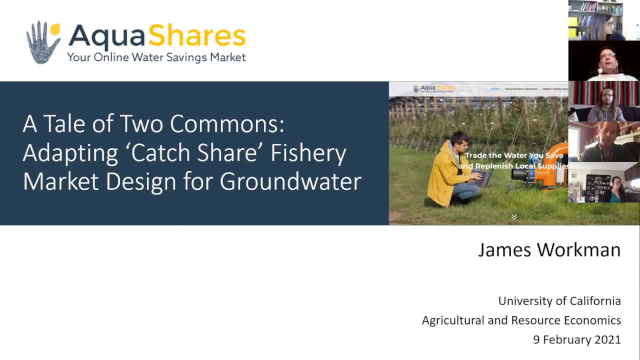 not out of a sort of an economic theory or out of a you know how do we make money off this, but out of an anthropological understanding of our relationship to natural resources, especially in the river. and you know there are three big factors that are driving the relationship to. 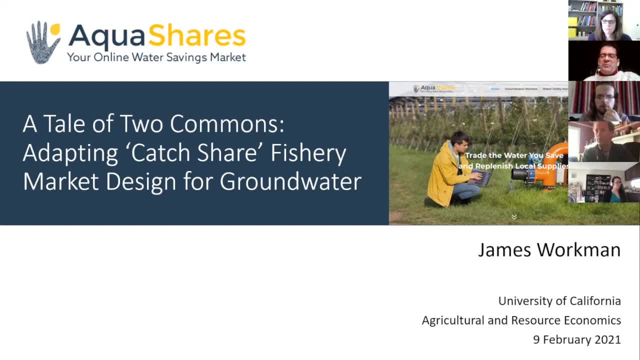 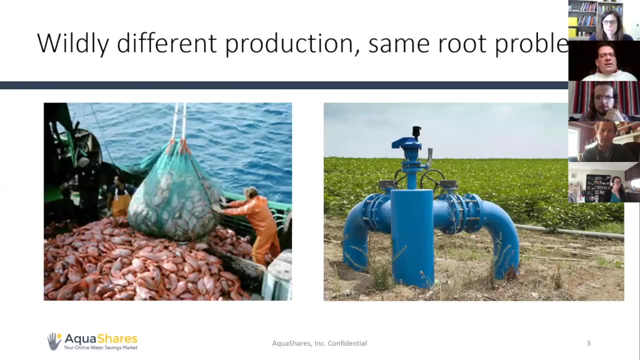 water and fisheries And the parallels driving both of them is going to be a great segue, I think from Kalyan, because they both are informed And basically, you know, in terms of a philosophy, we worship at the altar of Eleanor Ostrom. I'll get into that in a bit, But in terms 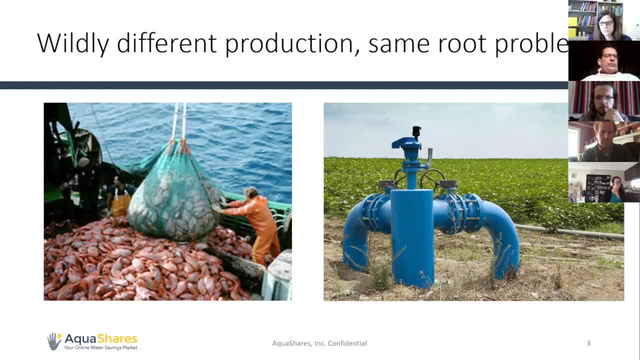 of your first question. you know, on the surface these are two totally different economies. two hundred nautical miles offshore, the others hundreds or thousands of feet above sea level. you've got these two different resources: fish- we're going to produce them, to eat them, and water is more a means to an end of producing food. 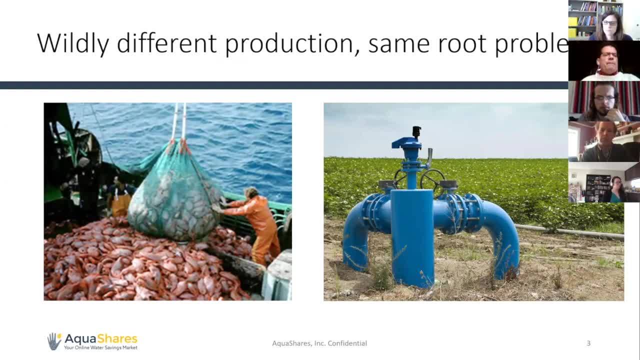 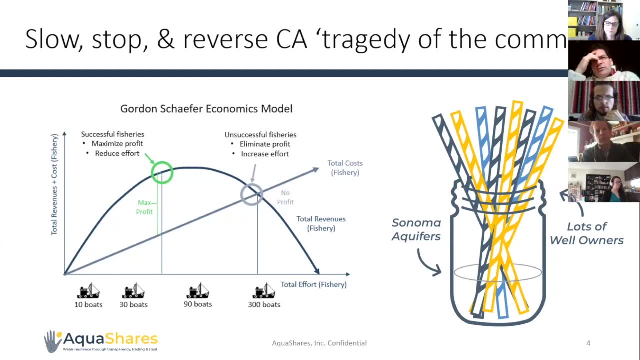 of producing energy and so forth. and then you've got this other culture of wild capture in a matter of hours or days, versus the sort of planned cultivation over months or years. but when you do scratch the surface, they come down to these same questions of who owns this wild resource before it's. 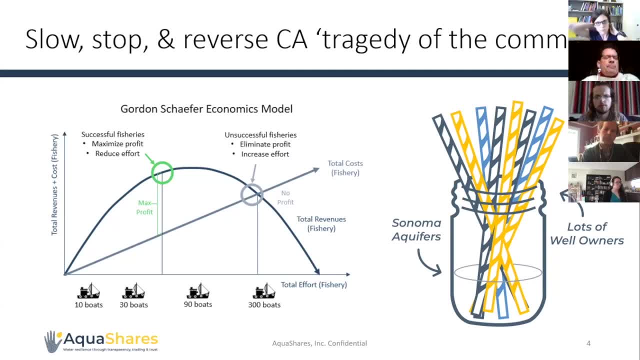 before it's brought to the surface for economic use? and how much do we need to extract from nature, can we leave behind, and where should the value of these benefits flow as a priority? and these, as Kaylin said, have subject for a lot of back-and-forth, a lot of tension, a lot of evolution. and how do we feed you know? 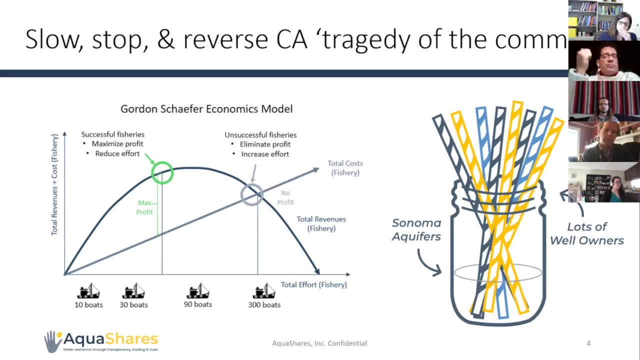 our growing human appetite with this wild resource that is- and this is both of them- finite or shrinking. it's renewable, it's invisible until it's hauled up to the surface, it's a fugitive resource and that it, you know, frustratingly, doesn't stay put. it's this great saying of you know managing fish. 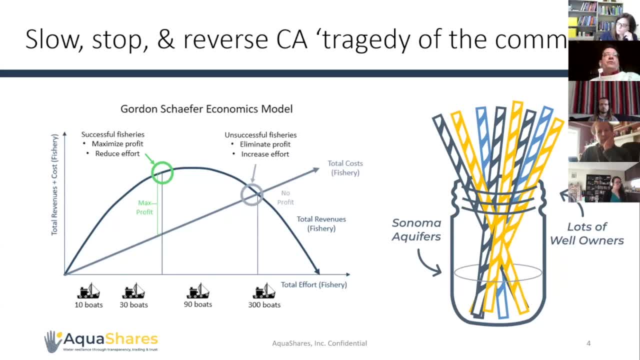 is just like managing forests, except, unlike trees, fish move and they eat each other and they reproduce, and water has got a similar kind of complexity of what's? what's it doing down there under the earth where we can't see it? and yet we can't see it? and yet we can't see it because it's just a. 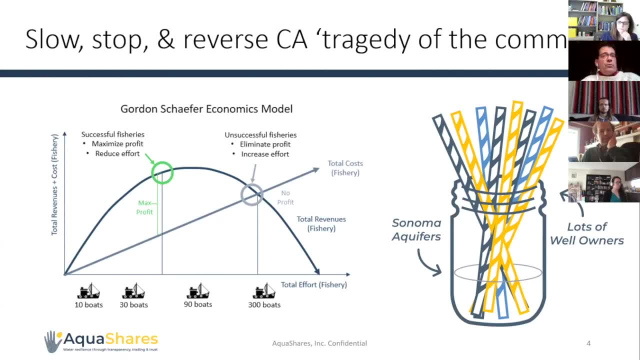 priceless, you know, worthless in its wild state, and priceless and captivity. and if we take more than you know the, the resource can bear more than its carrying capacity. we put too many boats on the water, catching too much fish too fast. it's the same thing as putting too many straws in that aquifer milkshake. it. 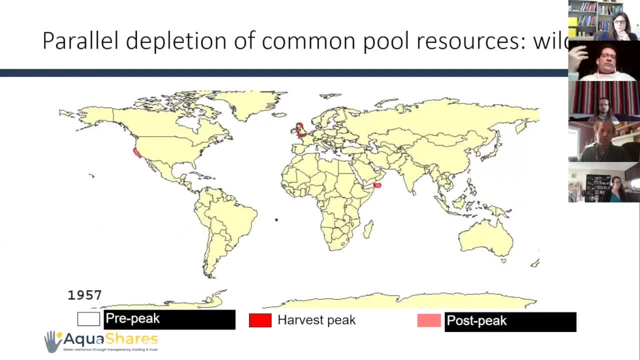 leads to collapse in many ways. quite literally- and I like this map just to sort of show things- I want you to look at California as one of the first areas. Look what happens in 1976 with the passage of Magnuson-Stevens Act: Absolutely nothing. 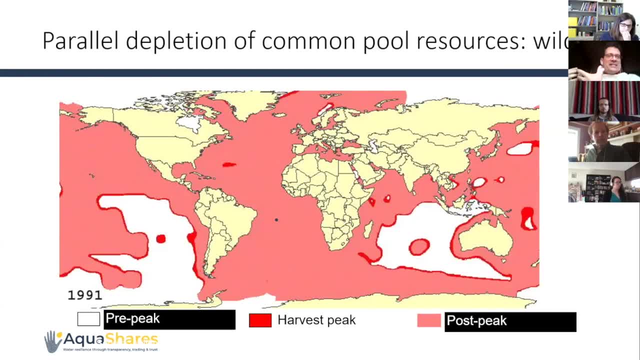 You've got this regulatory force, this landmark, put in place to say, okay, we're going to manage fisheries. and the depletion did not stop. In many ways it got accelerated and it got worse. We see a similar kind of thing where we can understand what's going on beneath the surface. 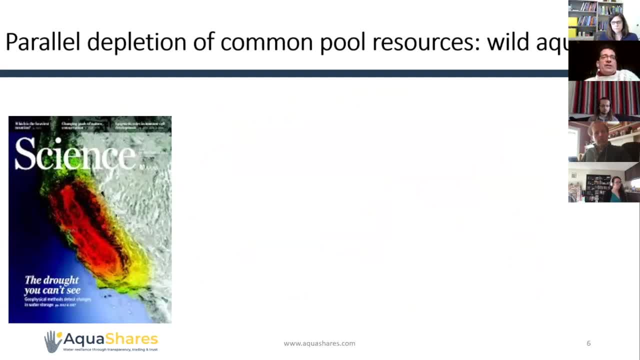 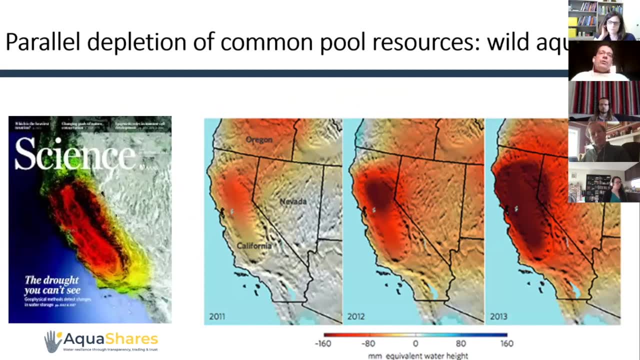 Grace is this fantastic satellite-driven technology that measures how far is the depletion happening, where is it happening, and yet that doesn't really equip us with the tools to deal with this, to stop this depletion, to slow and reverse even the over-pumping of aquifers and the over-extraction of fisheries. 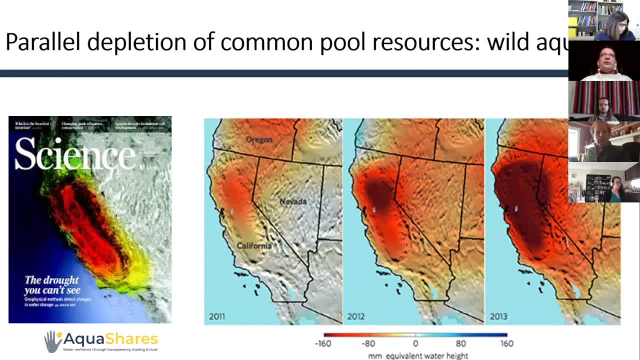 So this is all sort of the usual doom and gloom and as a journalist for many years, I thrived on that. I was like, oh look, how stupid This is. oh, we're killing the golden goose. but then I started to say, okay, let's look at some exceptions. 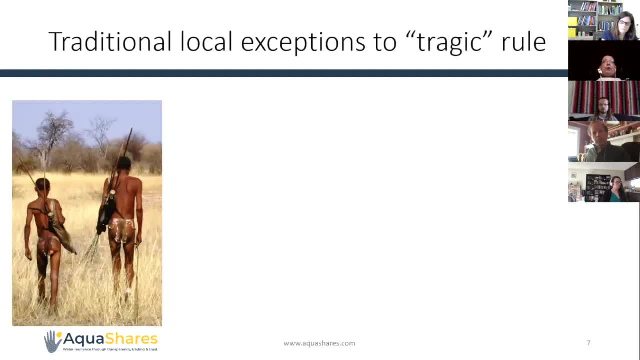 Let's find places where it's working, where people aren't over-exploiting their resources, and this took me to one of the hottest, driest places on earth in the Kalahari Desert of Southern Africa, where the Bushmen have been managing their resources, if you put it that way, for thousands of years, despite no standing water. 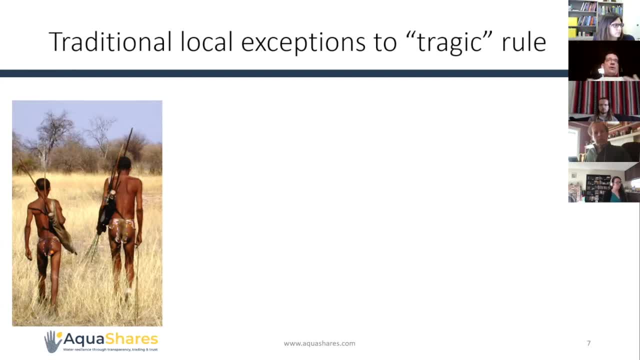 Their system was called Taro and I learned from them how they truck, barter and exchange these resources And it turned scarcity into abundance and potential conflicts over those resources into cooperation, And I wrote this book about it and it sold 27 copies and so forth. 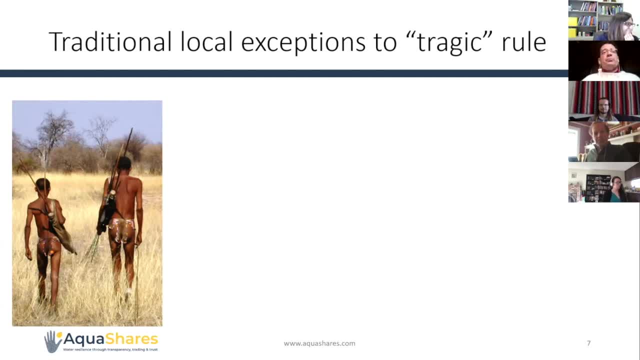 But what I learned afterwards was that it wasn't just the Bushmen. Hundreds of societies around the earth, from the Arabian Peninsula to Morocco, to then Persia, modern Iran, for hundreds or thousands of years, had these systems called subaq or aflati. 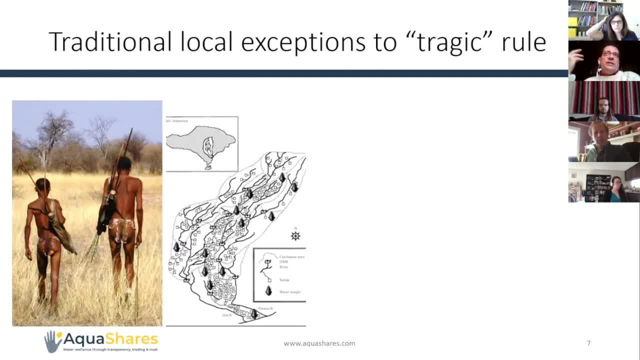 They were devolved, decentralized, self-organizing, self-management systems where everyone had skin in the game. Everyone had an incentive to use that resource efficiently, because if they didn't use up their share, they could barter and trade with someone else who didn't. 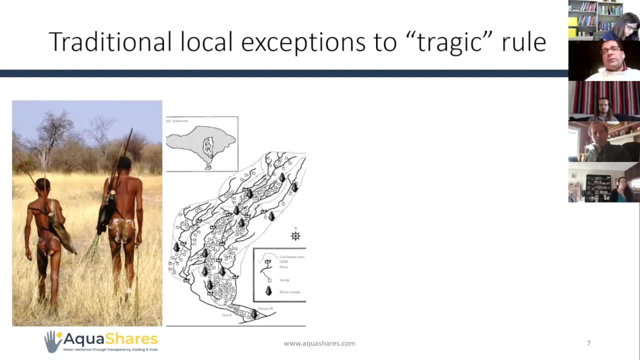 And those worked and they're still working to this day on the scale. Then I spent several years. I had the good fortune of working for Environmental Defense Funds, And I spent several years. I had the good fortune of working for Environmental Defense Funds. 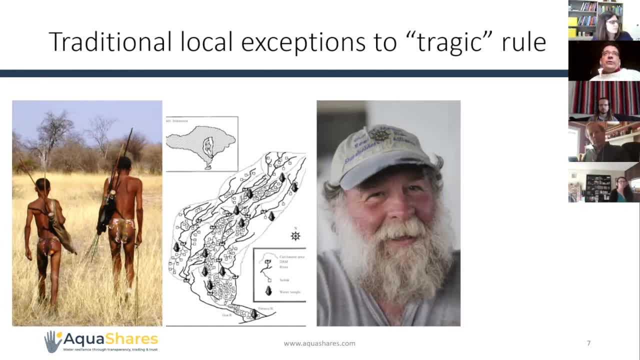 With this guy, Buddy Gwinden, who's one of the highliners in the Gulf of Mexico of Red Snapper and Grouper, And he was dead set against this whole ITQ catch share system because he figured, oh man, I got a good deal going. 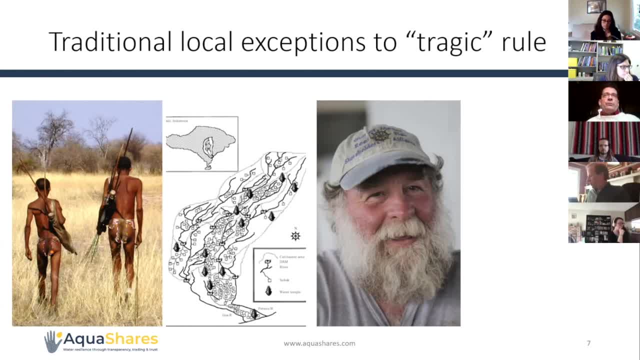 I'm catching the most fish here. This is just a way to screw me over and redistribute the wealth for me, And he was one of the people who had depleted that fishery more than anyone. But as it evolved, as things unfolded, as the votes went against him, he was one of the people who had depleted that fishery more than anyone. And as it evolved, as things unfolded, as the votes went against him, he realized: geez, this is a good system. And as it evolved, as things unfolded, as the votes went against him, he realized: geez, this is a good system. 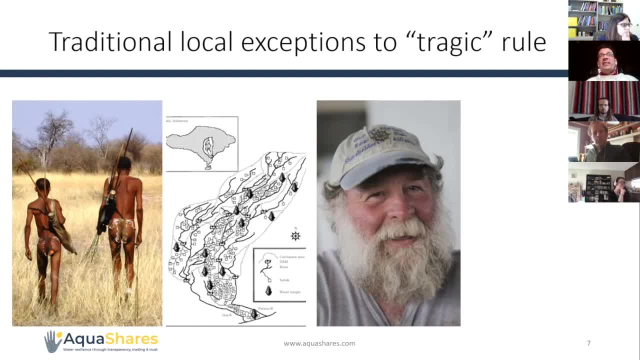 It's going to work out for me. It changed his incentives And, as Kaylin said, it made him a millionaire overnight. What it also did in the process was it gave him these incentives to hold back, to slow the slaughter of what was going on. 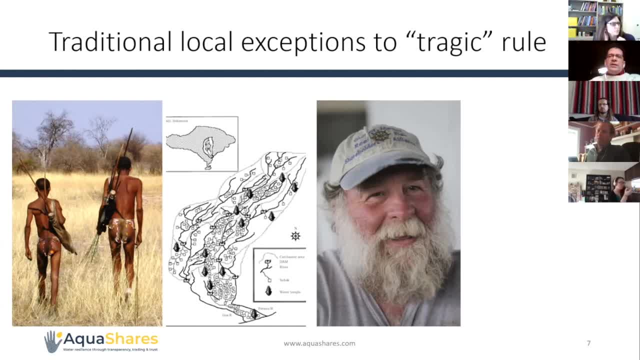 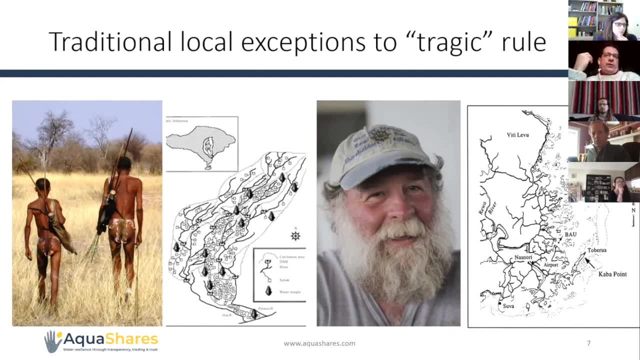 Him and hundreds of other fishermen in the Gulf could change their ways. And while this was a modern instrument, it's important for us to remember that these kinds of catch share, these co-management systems, they weren't just invented in the 60s or 70s or 80s. 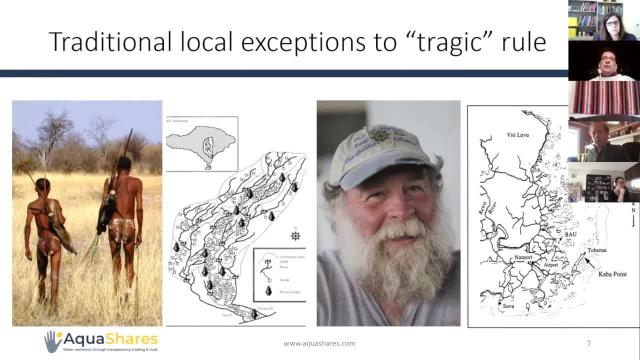 Some of them again go back hundreds of years in Fiji and Palau, off the coast of Turkey and India, and the traditional customary systems of rights-based management among people who were illiterate and innumerate, and yet they managed their fisheries in a way that is just extraordinary and complex and diverse. 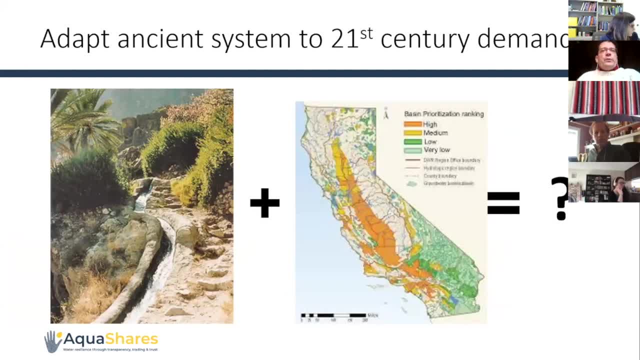 So the question for us, for aquasharers and, I think, for all of us on this webinar, is: okay, that's great, That's very quaint and all these traditional systems that worked for hundreds of years, but we've only got 15, 20 years max to be able to comply with these new things crashing down on our heads of stigma. 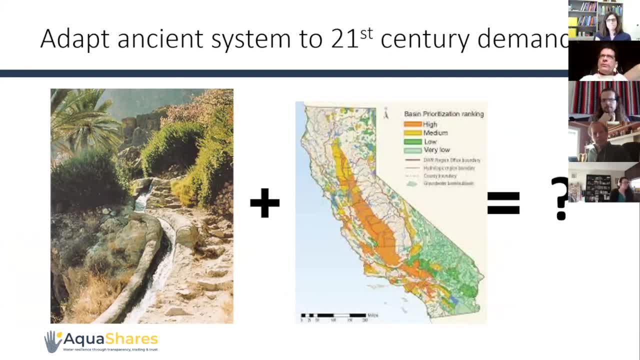 How are we going to make that work? It's not just a matter of a small little watershed or aquifer in the Arabian Peninsula. We're talking hundreds, even thousands of square miles of productive agricultural lands. So how do you scale that up in time and in space? 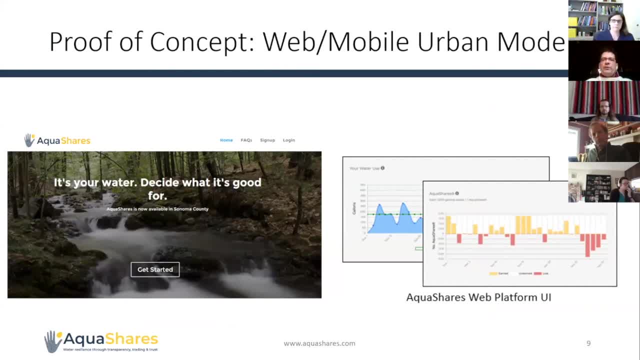 Our approach was like: okay, Well, let's look at what technology can do. We're not going to be carrying water, We're not going to be diverting physical wet water, but we can monitor these credits and let people trade what they save. 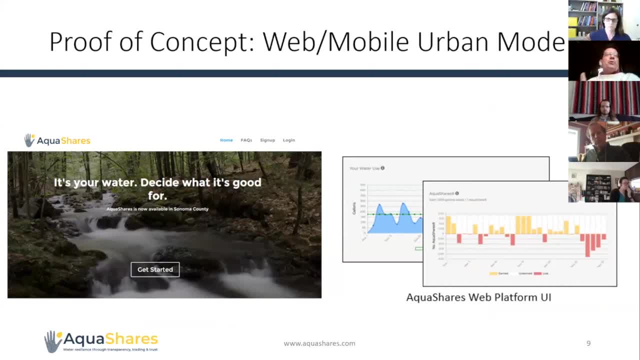 When we started this proof of concept, we cheated a little bit. We worked where there was existing institutions, namely utilities that depended on groundwater, first in Sonoma and later in Marrakech, Morocco, And what we wanted to show is: like: what do people do? 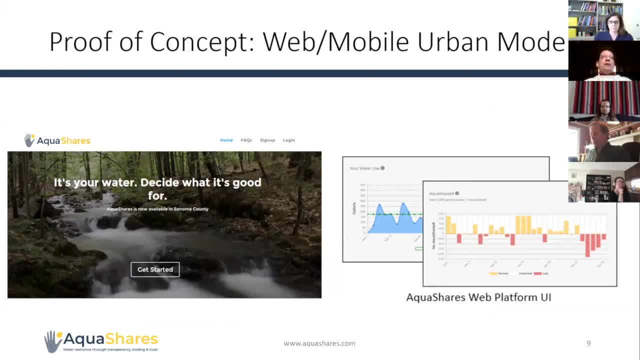 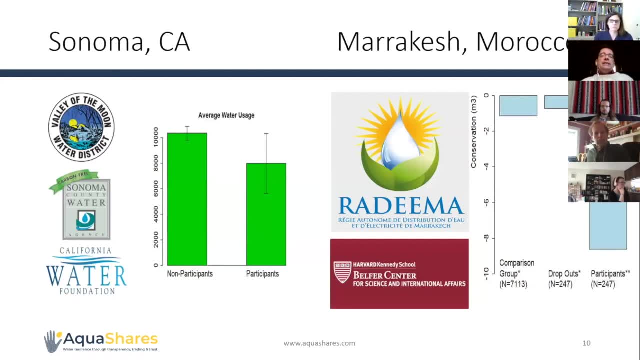 Did their behavior change when they've got skin in the game, when they've got a stake in the outcome? And, Sure enough, working with the California Water Foundation Valley of the Moons, Sonoma Water, it did. And then in Morocco, same thing. 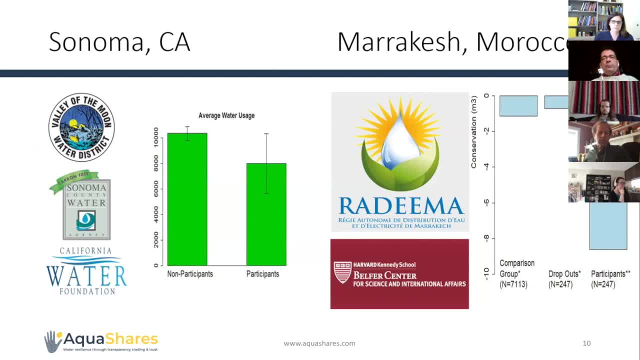 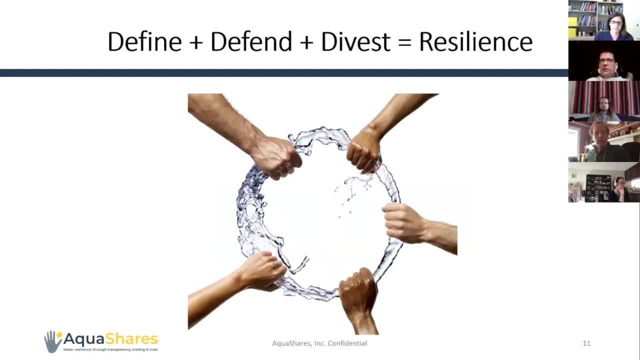 They didn't have a screen and so forth. They worked off text messages once a month, But once again, the group that was participating saved a lot of water. The question now bringing it to groundwater. in both cases, in both Sonoma and in Morocco, they said: well, this is great, but urban water only uses a fraction of that groundwater. 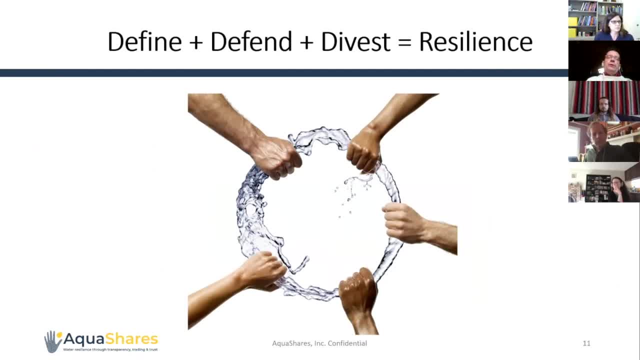 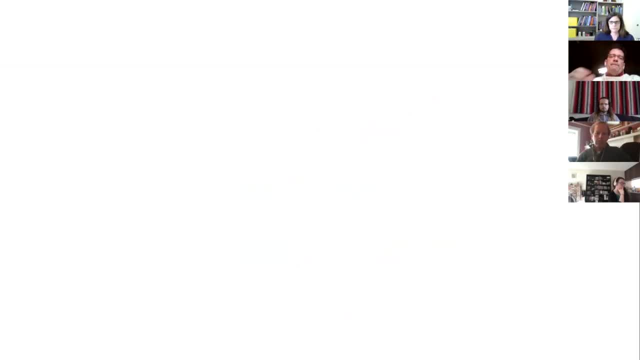 Can you extend this? Can you expand these principles, this system, This platform, to groundwater as well? And I'll stop there, basically using these same principles. Thanks, Jamie. Yeah, so in what ways, I guess. more specifically, has the AquaShare's approach been shaped by? you know what we've learned from fisheries management tragedy, of the commons work of Elmer Ostrom that you mentioned before. 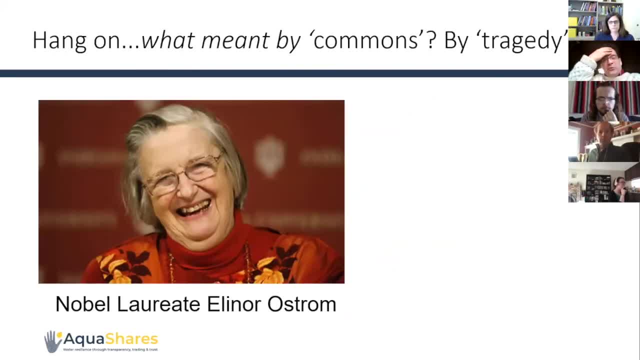 Yeah, As I said, you know, we worship at the altar of Lynn Ostrom And the reason we do is because, You know, the real tragedy for us, as we learn this more and more, is that we often now associate- thanks to Garrett Hardin's work, we associate- the commons with something bad, with something sinister, with something weak. 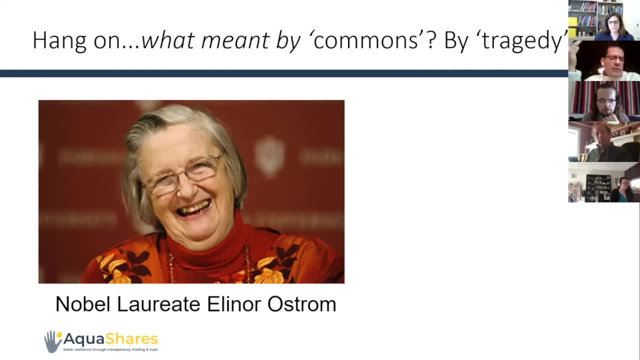 And his, you know his solution was like: oh, commons are generic, they're monolithic, they're weak and simplistic, sort of like a bumper sticker- the tragedy of the commons when you read that. And the only solutions are these top-down, centralized regulatory crackdowns. 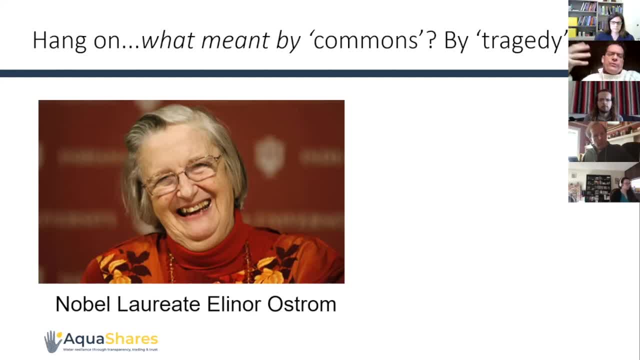 And what Ostrom gave us back was this recognition that commons are unique. they're nuanced contours, they're- they have, you know, a fascinating history, and they're a collection not of autonomous atoms bumping into each other, but a communion of subjects, of people who come to the table and say: we got a problem, we got to work this out. 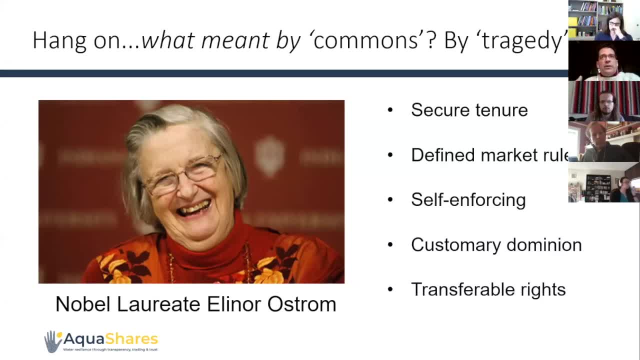 You know how are we going to do this? And finding, as she did, in fisheries and in groundwater, I think, groundwater- And you know how do people resolve these, these challenges, and they don't just sort of deplete the resource, they figure out ways to put restrictions on themselves. and it's a messy, complex process, as she says, and it's the worst kind of management, except for all the others. 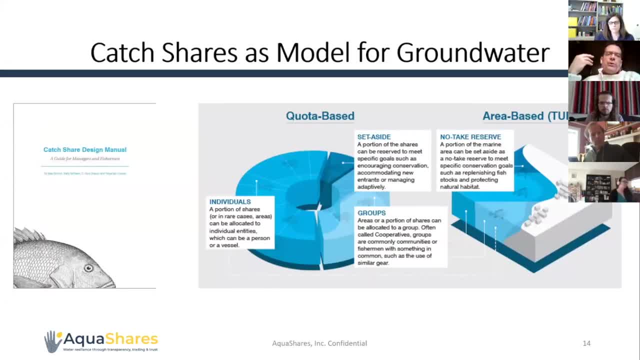 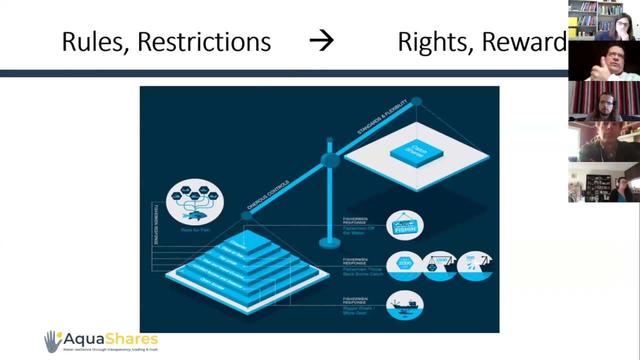 And we've taken that and, as I said, from EDF, has built on these lessons and applied them to natural resource problems, especially with fisheries, And they can learn these lessons And said, okay, instead of you know, putting these onerous top-down controls on, you can only fish Tuesdays, Thursdays and Saturdays- and saying, you know, wait, let's, or you can only use this size motor or this mesh net or this kind of equipment. 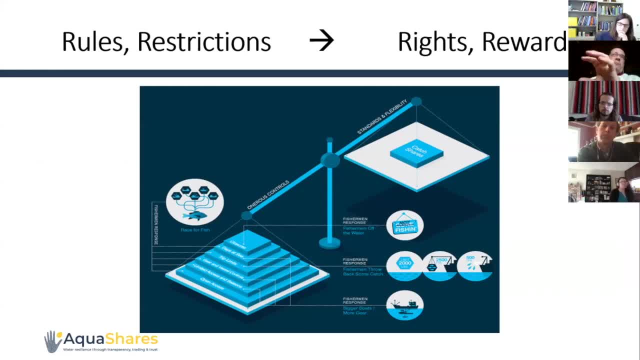 They trusted and worked with the fishermen to say, look, you need to make a profit. What if we? and we need to make sure the resource isn't depleted. What if- here's the scientific threshold- you get these quotas and how you catch that is up to you. 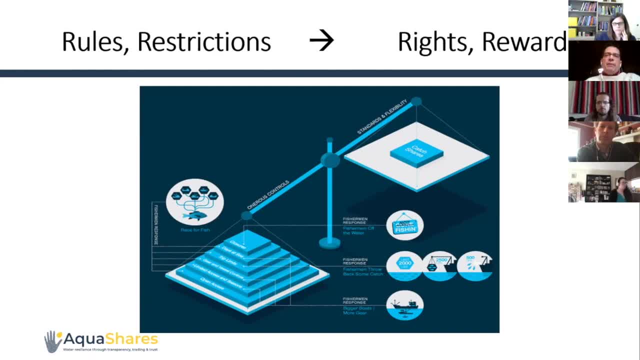 But we're going to be watching, we're going to have monitoring, We're going to have enforcement And that changed the dynamic a hundred percent. where they felt trusted, where they felt there was incentives and where they knew there was going to be, they're going to be held accountable to, to meeting that. 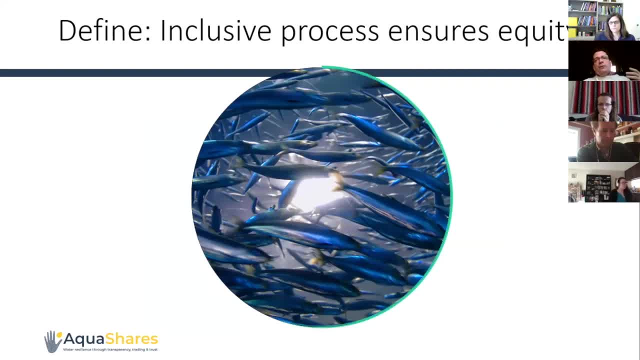 I won't go too much into this, but it's a one way of thinking of this inclusive allocation process which is, you know, 70, 80% of the time going into into catch shares is saying: okay, how do you set that initial allocation? 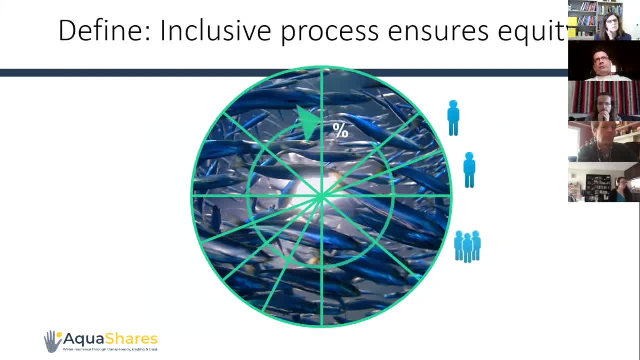 Who gets to participate. One of the reasons that went from individual transferable quotas to catch shares or sustainable management and ecosystem management is a recognition that fishing does impact more than just, you know, individual fishermen. It involves the coastal community. It involves the processors. 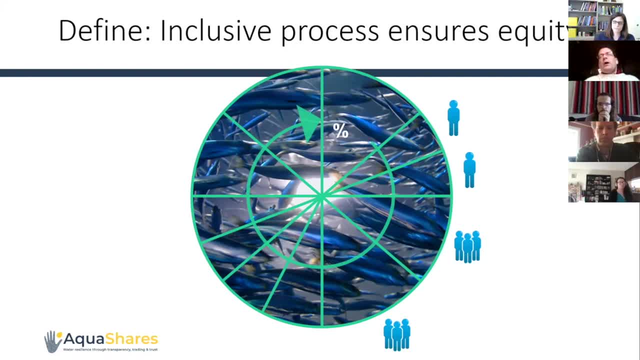 It involves the recreational fishermen, the subsistence fishermen, And what's been fascinating to me is seeing how, over time, these catch share systems do adapt, They do evolve, They create this wealth by restoring the fish, And then they bring more and more participants. 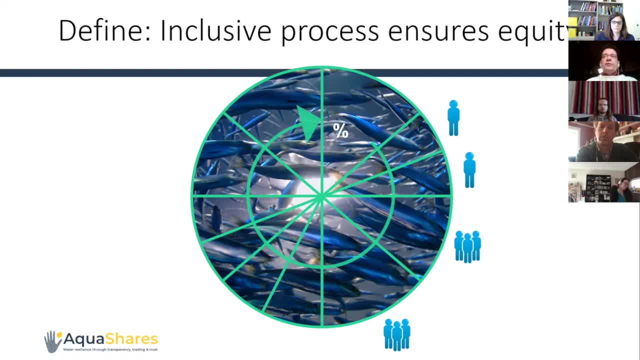 Into it New entrance. As, as Kaylin said, you need to have some loan programs, but the people who are actually loaning- you know- money or share to new fishermen are the people who actually have shares of the fish, because they want to make sure that there's a new generation. 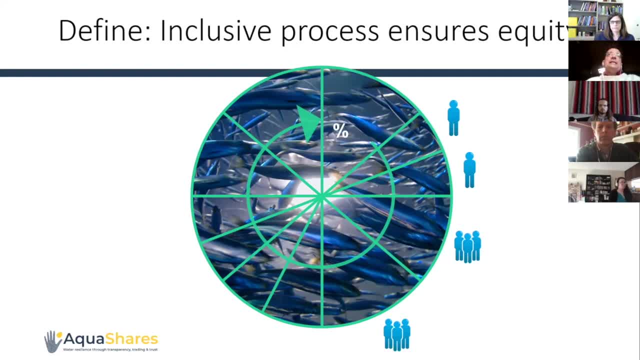 to come along and participate, Same with Alaska, the communities that she mentioned, some of the coastal communities, are among those that are generating and benefiting from that wealth. So there's this: make making sure it's an inclusive process, that that is equitable. 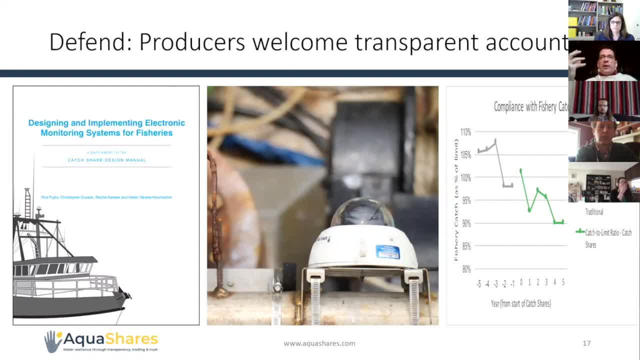 Kaylin mentioned this as well- on on on fishing boats and saying, okay, we can now have these electronic monitoring. That's an expensive upfront cost, but boy, it saves a lot of time, energy tensions and so forth. If you get everybody to buy into it, it has to be all or nothing. 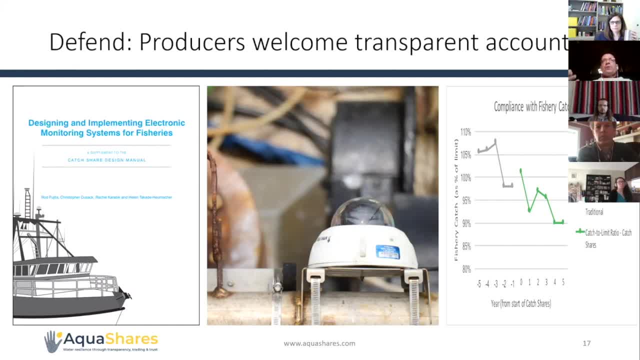 It can't just be: oh well, we're going to have observers on two thirds of the boats and the other third is sort of wild west. Make sure that everybody agrees on the terms And and the conditions of compliance. And again, what's fascinating is that fishermen- probably second only to farmers, are very, very guarded with their privacy. 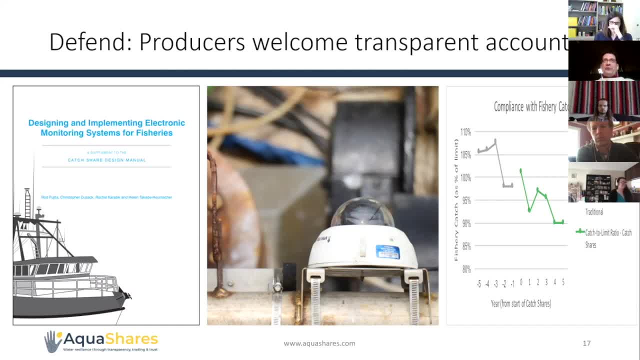 They don't want anyone to know when they're fishing, where they're fishing, how deep they're fishing, what gear they're using, Until they have a secure share of the resource in the water, And once that happens, they want to make sure that everybody's planned by the same rules. 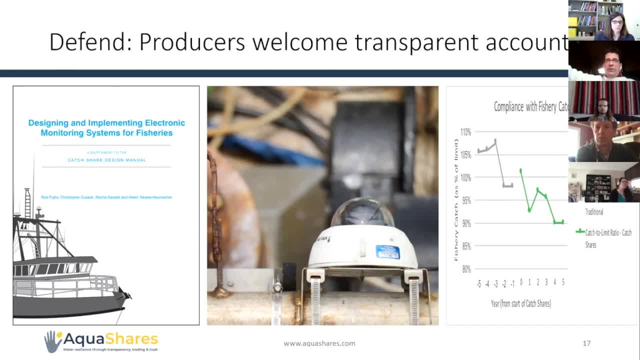 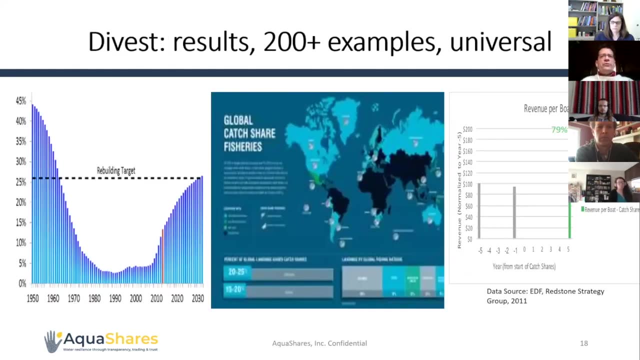 And they know that if they can't cheat, that guy over there 20 miles away and whatever he's doing in his fishing boat, can't cheat, and they start to move towards sharing of data, and that's the magical element of trust that is a key part of this: divesting your share, you know? granted it's like, is it need to be? what kind of a market? what kind of transactions? any market or transactions at all? 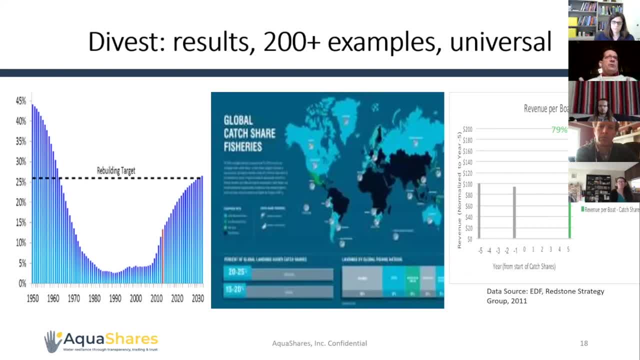 The main thing, whether it's a traditional fishery that you know, going back centuries, or traditional water system, Is that you need to be able to pass down your share to someone else, And if you can't do that, then you have every incentive still to exploit it. 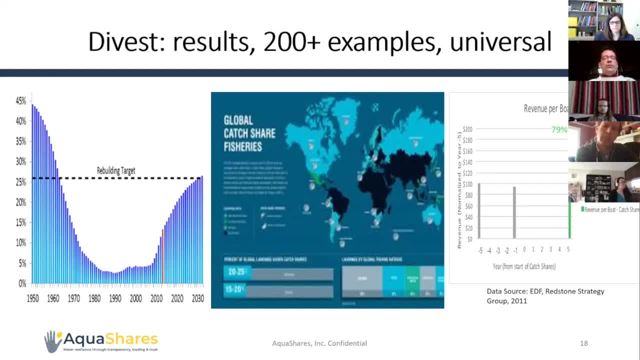 While you're, while you're alive, because then it just goes back to someone else and that's human nature and that's that's certainly a challenge in terms of the nuances of that. but when you do have that long term incentive, It's amazing. the fishermen started saying you know, we used to fight the regulators saying here's the catch limit and say no, no, no, that's too low. 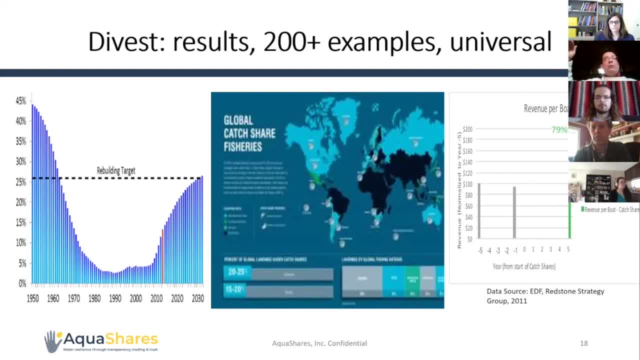 Now we're fighting the Regulators saying that catch them is too high. we want it to be lower so that it will recover faster, because we're looking 510 15 years down the road. That's one of the reasons why it has been so. 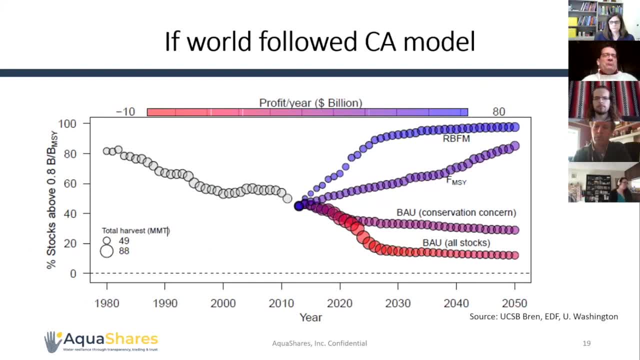 I want to tip my hat again to another UC branch is not part of the three here, but to UC Santa Cruz, where Chris Costello and Steve Gaines had worked with EDF to sort of model out is extraordinary, you know, understanding of what would happen if catch shares were implemented. 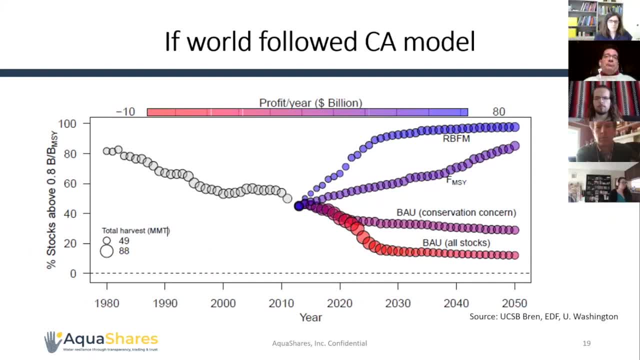 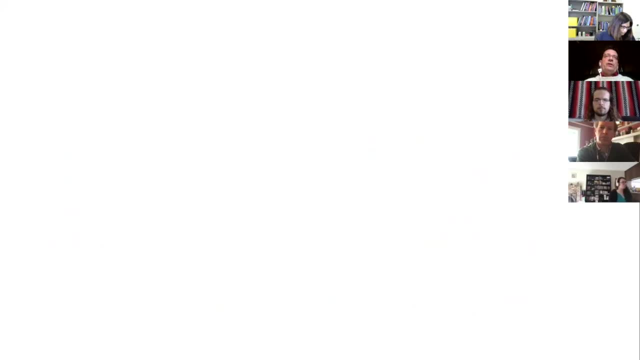 In different parts of the world, In different parts of the world, especially in some of the key places, if the California model was expanded and the business as usual, you know, continued depletion, even you know traditional management or regulatory crackdowns weren't going to be as effective as the catch share model and that's given us, you know, inspiration and hope. 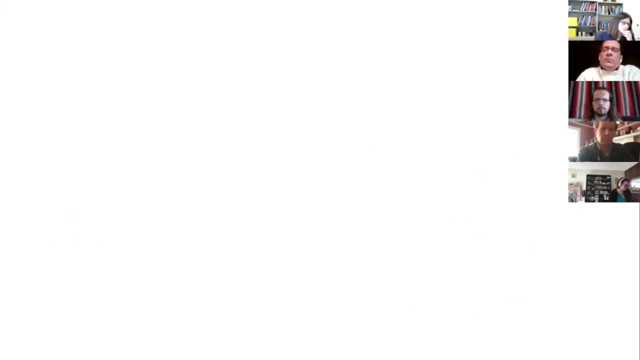 Great Thanks, Jamie. Yeah, I mean you touched on a lot of things that that came up in Caitlin's talk as well, like the stakeholder engagement And the importance of that in in sort of designing it and and like this adaptive market design and transparency and that sort of thing. So I'm curious if you could elaborate more on sort of how some of these concepts really manifest in practice and, like you know, sort of walk us through AquaShares approach from design to allocation to operation, and how do these, these lessons from fisheries, really manifest in the process? 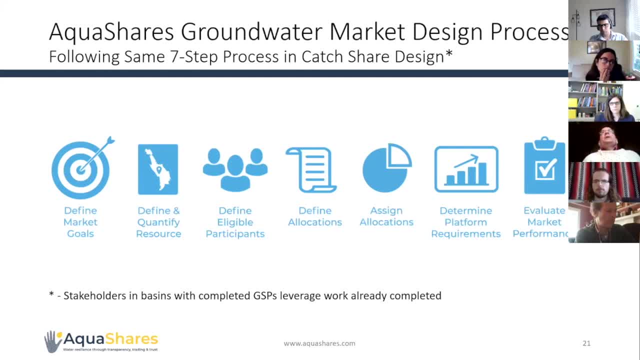 Great. I mean Honestly we. We relied pretty heavily on the Environmental Defense Fund approach to fisheries management because they had to sort of scale up really quickly lessons from Eleanor Ostrom and these traditional fisheries and so forth over decades or centuries. And how do we? how do we do this? in a you know way that is rigorous and yet flexible, that allows for breathing room. It still moves. you know the process. 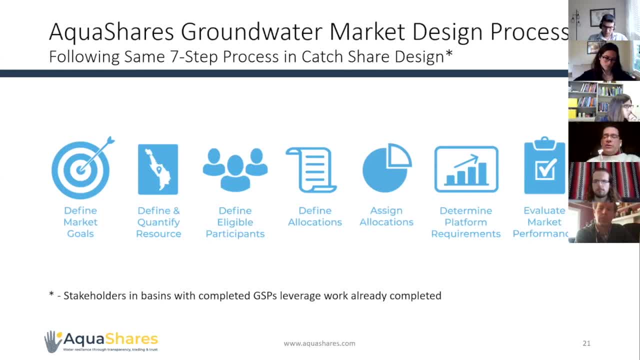 In the right direction. And this is important for every GSA, you know, as they're not just as they're putting their GSP together but saying, okay, we've got to go from, you know, this level of pumping and extraction to this level. How do we do that in a way that's fair, that's compliance, that's, you know, keeps people at the table, that avoids lawsuits. 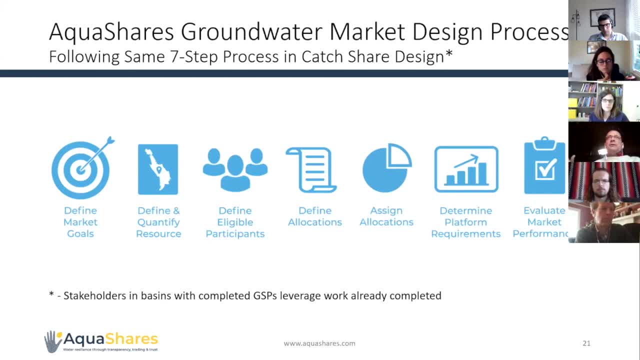 That protects groundwater dependent ecosystems, that includes disadvantaged communities, all these challenges that are, you know, driving people, And so you know. I think it's really important for us to be able to bring these lessons up the wall and bringing them to each other's throats, of saying there is a way forward And so we, borrowed from Environmental Defense Funds approach this seven step process. 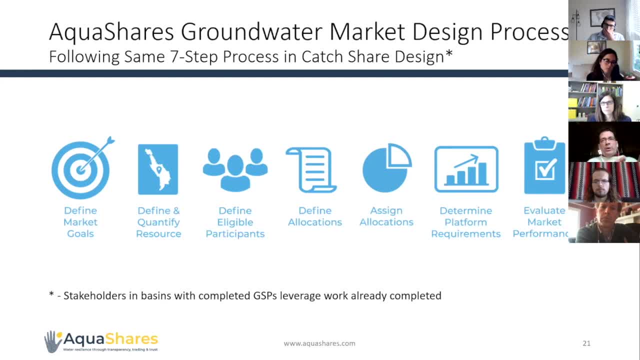 Where you start and the order is really important. Most people want to jump ahead to: what's my allocation? How much water do I get? When do I start trading? What's that water going to be worth to say whoa, whoa, whoa, whoa? Let's define what the market goals are. 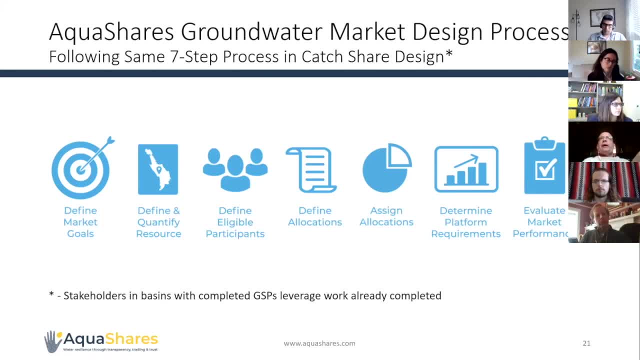 Do we want to have a purely export economy? Is it going to be 100% agricultural or do we have social values? And when we started doing this, It was like, oh, we actually want to preserve the Rural character of our county. We really think we need to set aside some for tourism, because the benefits from from coming to visit these trees that are found nowhere else are essential. Okay, let's, let's mark that down. 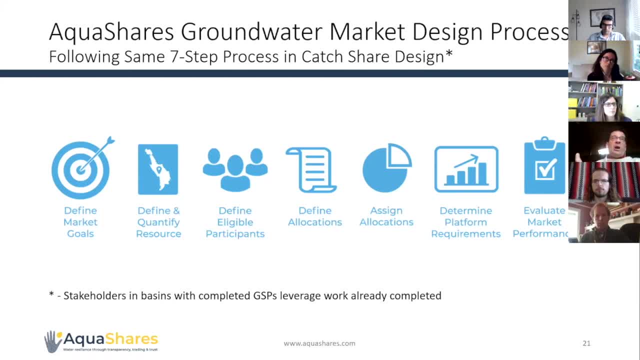 Okay, let's quantify the resource and there's like: well, we've got a shallow aquifer, We've got a deep aquifer, We've got a confined aquifer. Let's map those out. The hydrologist have done a lot of that work, but it still has some bearing of. like you include the water upstream in the watershed that flows down, or is it just within the boundaries there? 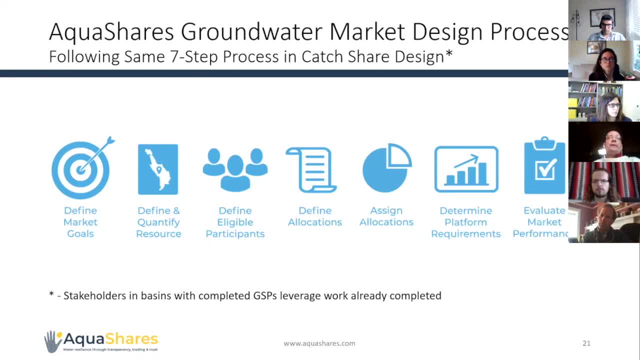 Oh, that's a good point. Let's look at that, Okay. well, who gets to participate in this, in this system? Well, everyone, No, Well, maybe not everyone. And we are just guiding this process. So they say: wait, if you don't have a well, what's your stake in the game? Somebody says, Well, I'm an environmentalist, That's my stake in the game. or someone else says, you know, I'm a social advocate. 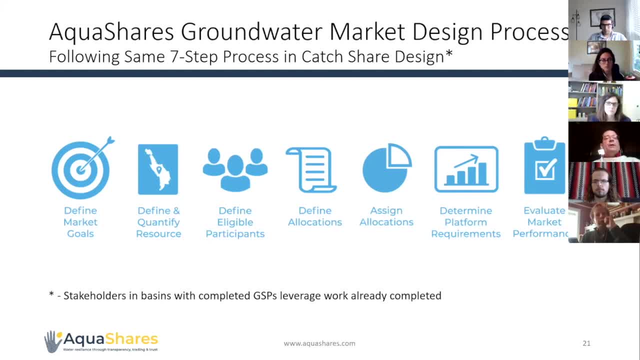 I want to do that. I want to make sure I can afford to live here. That's my stake in the game. So you work through these things and then you start to define the allocations. All right, get to these goals to make sure you're including these participants in this resource. Here's some of your options of allocations and here's how you can assign them. Here's how they can, how long they can last. Here's what happens if there's, you know, some water left over or building on the fisheries that aren't caught. 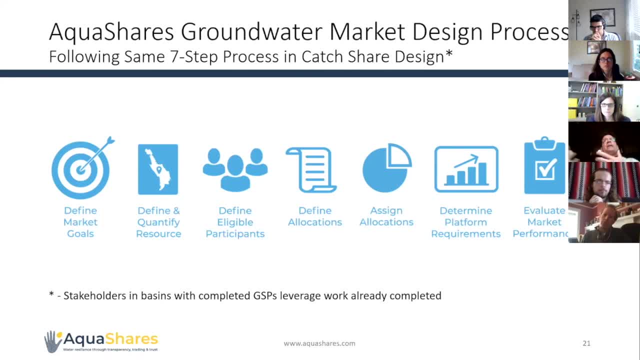 And then determining the platform requirements. What do you guys need to do to see, to know, to have confidence that someone else isn't cheating and that you're playing by the rules and so everyone's playing by the rules, or that the system is working for you? 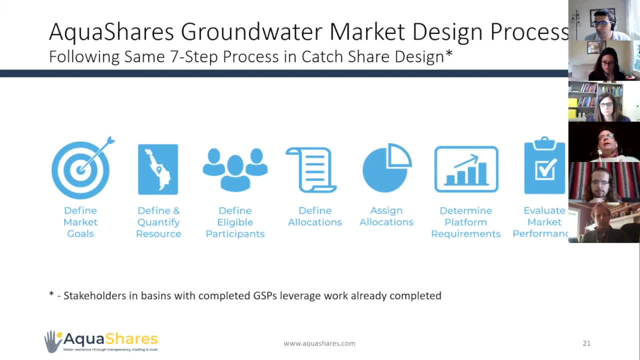 And this last one is really important as well- evaluating and monitoring the performance of the markets, that it's not just a once off Boom. done that, you have this room to evolve, to adapt, to improve the system, based on what you learn from each year, that each you know, each day, each week, each month. And this last one is really important as well- evaluating and monitoring the performance of the markets, that it's not just a once off Boom. done that, you have this room to evolve, to improve the system, based on what you learn from each year, that each you know, each day, each week. 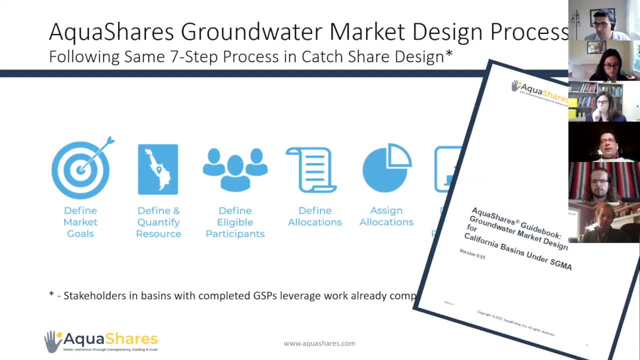 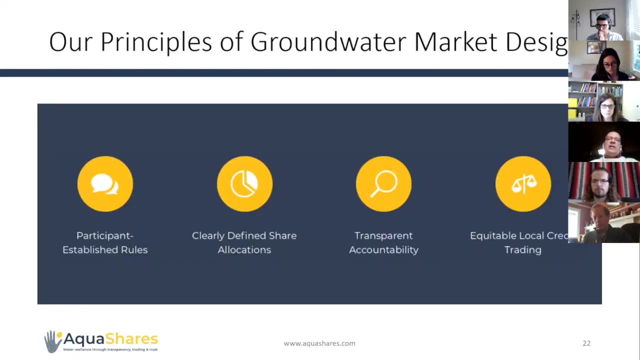 And this basically led us- and I'll talk about that later- into developing an 80 page design manual of how can a GSA use this approach in a very structured and rigorous manner that doesn't force anything, that keeps people at the table. It's based on these, you know, four principles of participant: established rules, clearly defined share. allocations of transparent accountability. 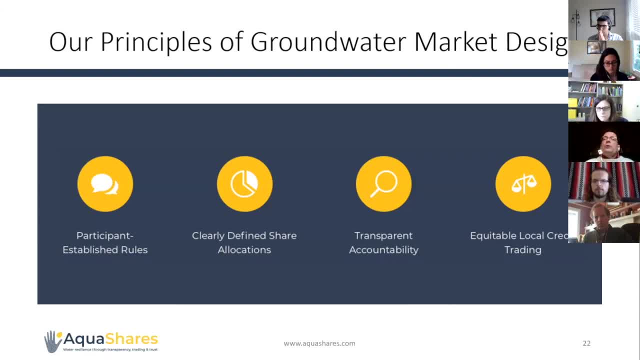 It's based on these, you know, four principles of participant established rules, clearly defined share allocations. of transparent accountability. making sure that this is equitable. and local trading- that you don't have some speculator in New York that's going to be jumping in and participating and skewing the outcomes. 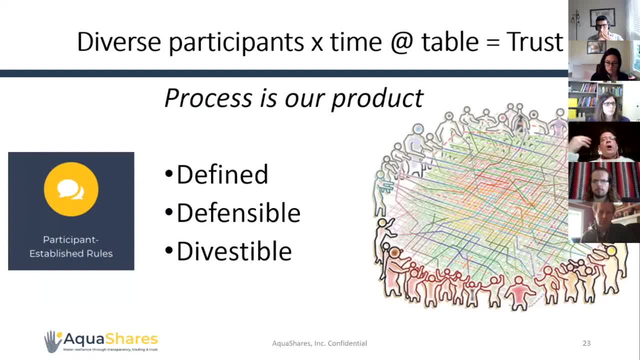 Again learning from Eleanor Ostrom, that the process it's a messy process, it's a difficult process, it's contentious and it's the best way possible moving forward that you need to have a diverse group sitting at the table bickering with each other, hashing these things. 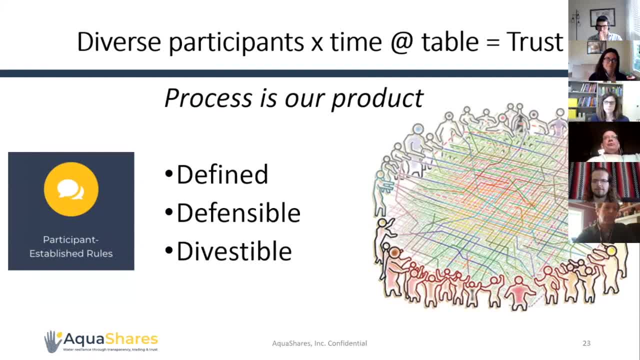 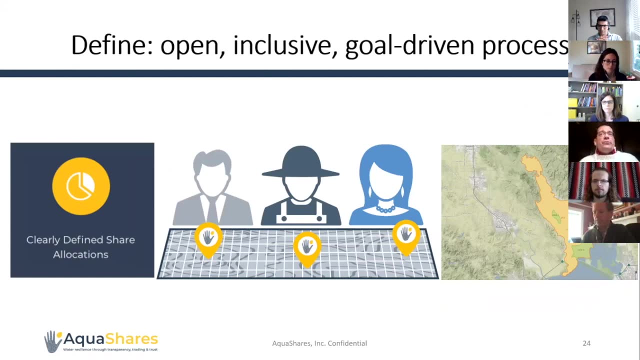 out, slamming their hands on the table, storming out of the room but then storming back in because there's really no other alternative of how they defined and can defend and divest of these shares. Working that out through this open and inclusive and based on goals and rights-driven process. 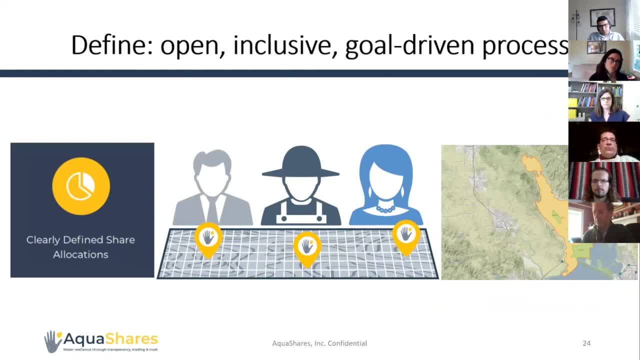 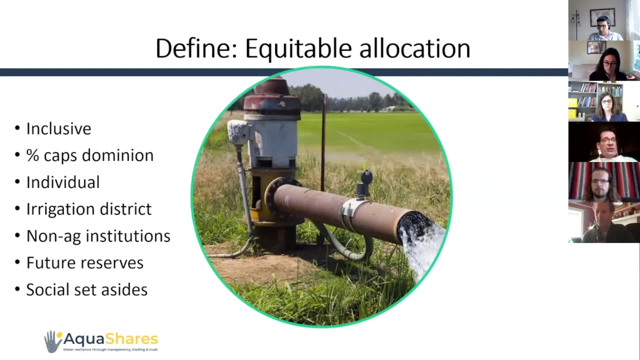 that looks at the place, that keeps all the stakeholders in mind, and you're looking at a map and saying, okay, where can and can't we, You know, clarify some of these shares? This will look familiar: Making sure that there are concentration caps, if desired, so that no single sector or no 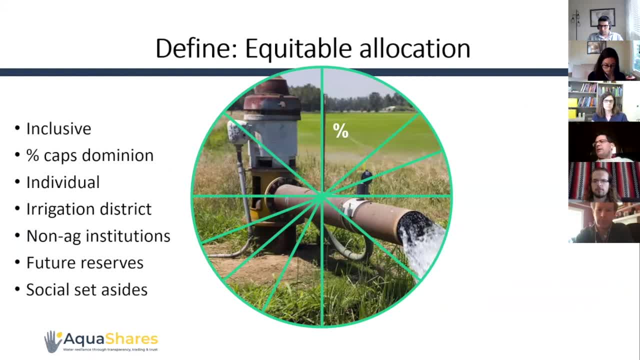 single individual can dominate the market, can make sure that there's- you know, no one else can get their shares, and so forth. Making sure that there's social set-asides and reserves and includes non-commercial, non-agricultural institutions. 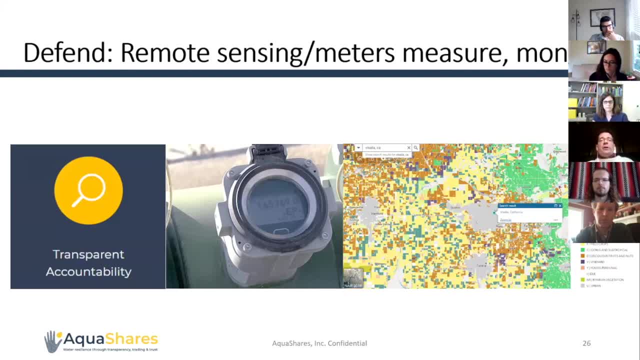 Finally, this is the equivalent of those onboard monitoring, of making sure that the meters are in place, that people know how much they're using and how much others are using, and that this process is transparent, that there's feedback loops so that you can ensure that you're improving that. 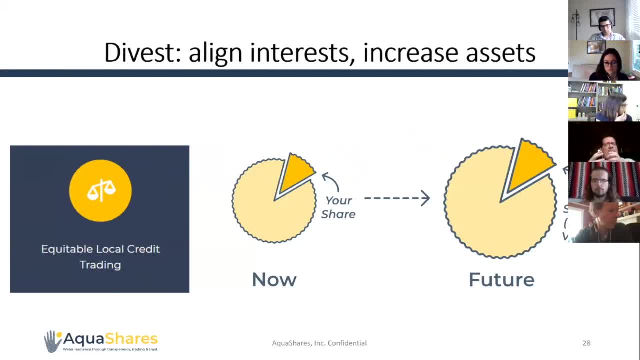 And again going to that divestiture of making sure that if we do this now, if we get this right, if we, you know, hold back over the next couple years, we're going to have more water to use in the future. 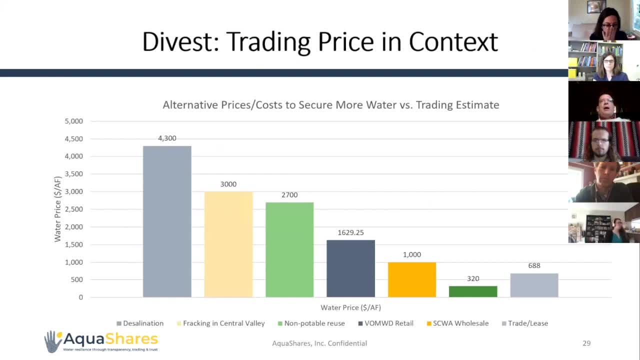 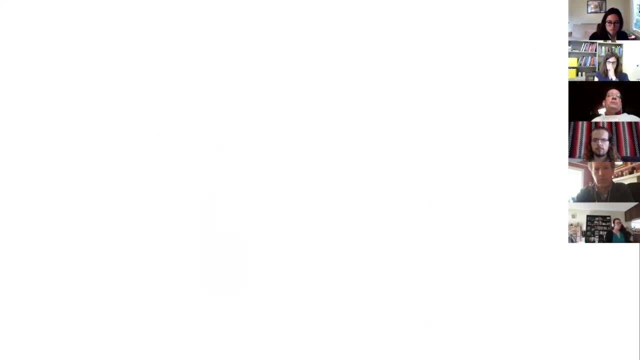 And that's going to give us ever more flexibility and it's going to be a lot better than all these other alternatives like importing water or desalinating water or treating water that are on the table now. Great, Thank you, Jamie. There's one last question and then we can open up to audience Q&A. 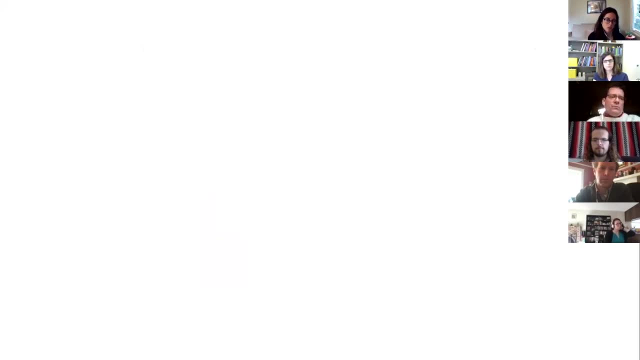 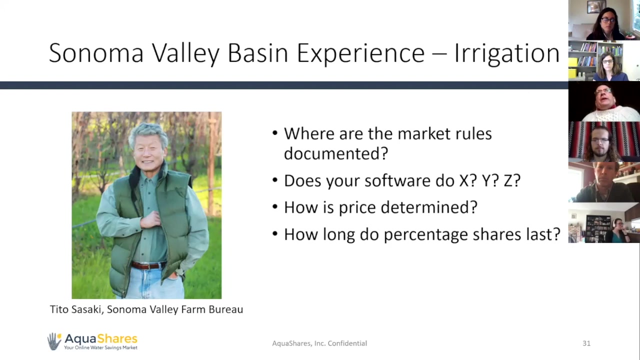 I'm curious if you could elaborate on some of your experience so far with groundwater markets, sort of if you have any successful collaborations Among various agencies and stakeholders that you could share with us today. Yeah, Thanks, Ellen. I mean Sonoma was our best and most involved process coming out of the initial, the urban 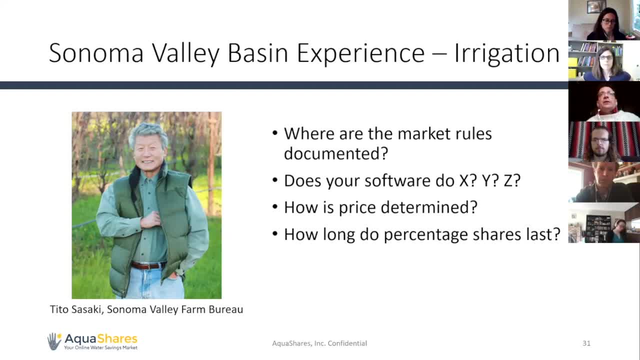 system there- Sonoma County Water Agency- and they had some very progressive and diverse stakeholders that were already looking at this problem, And so they called us and said: look, you know, is this something that you can help us with? And we sat down with this diverse group that had been, you know, they knew each other. 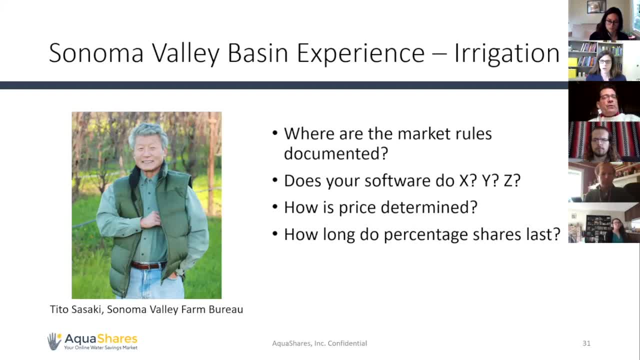 You know, from a meeting occasionally just sort of trying to figure these things out, And the questions that they brought up are the kinds of questions that you know we sort of anticipated, but then there's a lot of new ones. Generally they say: you know, does your system do this? 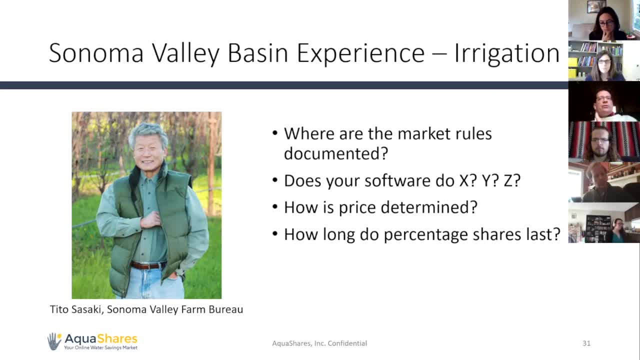 Does your software, you know, result in that? How do you guys determine the price? How long do your percentage shares last? And the main point for this constituency is to say we don't do anything, Our software doesn't do anything. 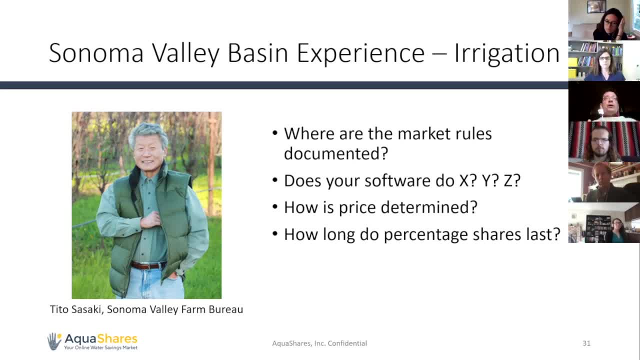 Right, The market, the software, the system, the design process is just a means to an end. You guys got to decide what that end is And that sort of threw them back for a second because that's something they had in mind. 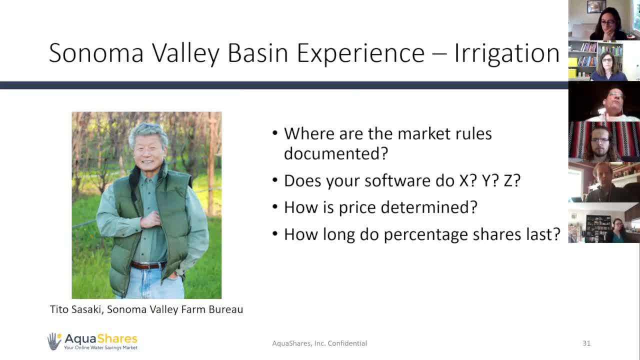 maybe in their head, but they hadn't really hashed out together of what they want that water to be used for, how they want to give it the most value: social value, environmental value, economic value, political value, The large, you know. fifth generation. 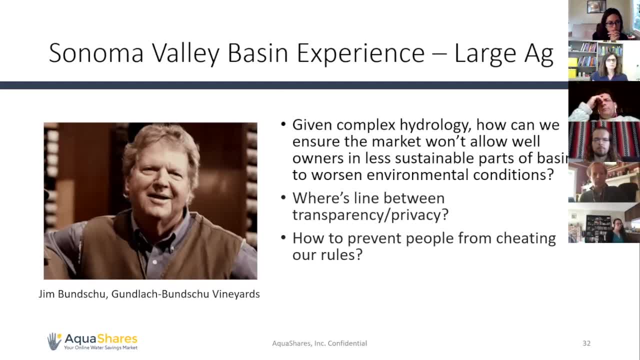 Uh, agriculture, uh, irrigator Jim Bunshu, um, you know, came in this really kind of skeptical, really not not hostile or anything. He's like open to this, but he had questions about transparency. It was just like geez, you know, is this going to let everybody know how much water? 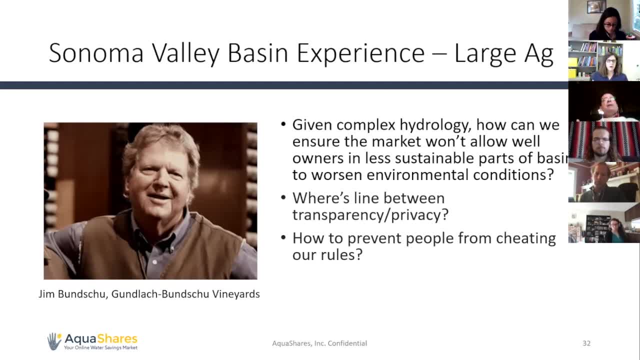 I'm using, Am I going to be get a black eye? But over time he started to say: you know, this is actually a way of building trust And that trust is much more important- uh, in the longterm that I want to know who else. 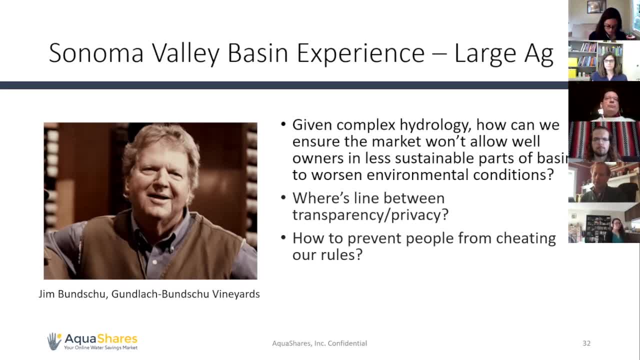 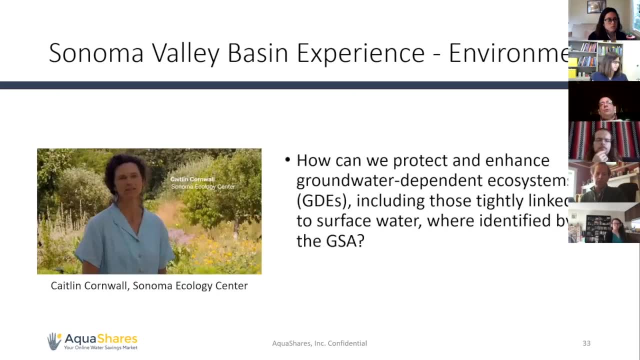 is out there what the rules are, how they're being complied with, Um and uh and preventing others from cheating. and that way I know I can't cheat, Others can't cheat as well. Um, the, the ecology, the, the environmental, local environmental group, you know, had a. 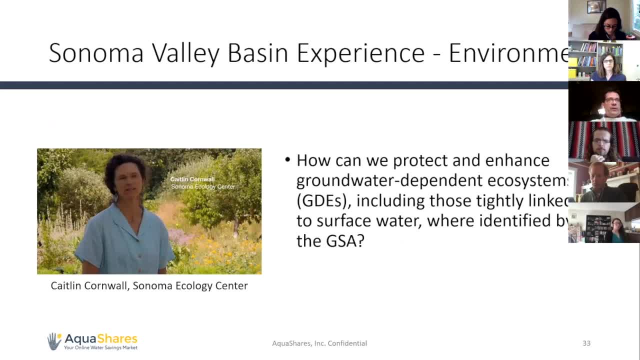 very strong saying: is this going to- just, you know, set aside those groundwater dependent ecosystems? And there definitely were some tensions between the producers and the environmentalists on this. but when they started looking and hashing out the details and looking at their goals, 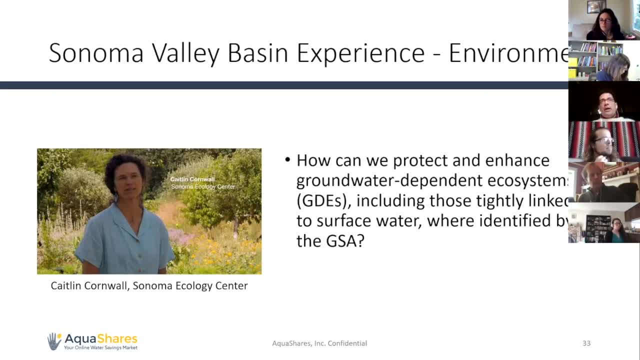 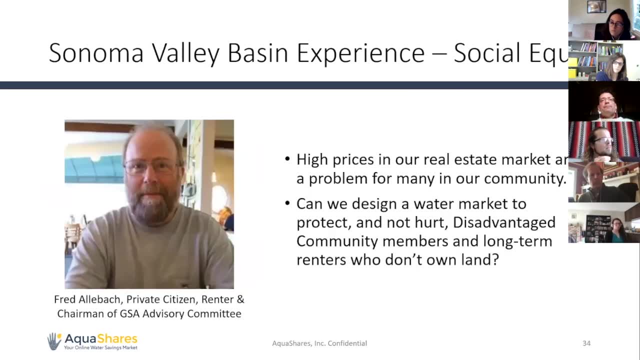 of timing of extraction, the location. They found that there was a lot more flexibility built in uh and open to them that they could build on Um again, uh, uh. Fred was a great social advocate saying: look, I'm a renter here. 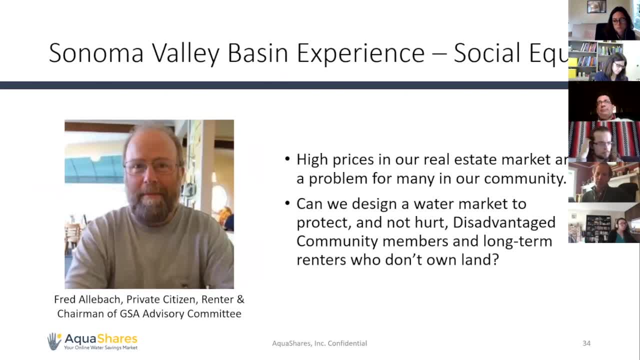 I've seen prices go up on everything. is water now going to be the last thing that pushes me out, uh, out on the streets? Um, and you design a system that incorporates the needs of people like me of uh, of farm. 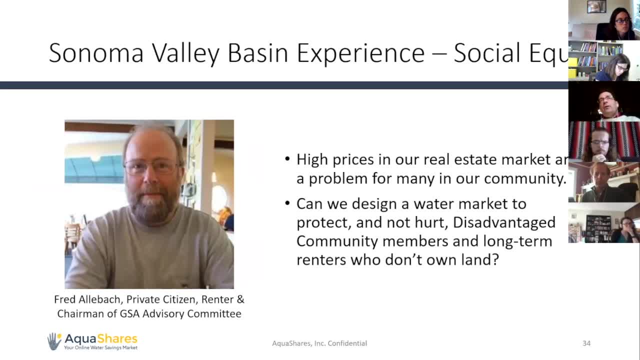 workers of, of migrants, of uh uh, others, That disadvantaged communities. we started working on that again. commercial guys were Oh, I don't know about this until they started looking at the knees and it was a rounding error for some of them to say, Oh yeah, no, we can definitely include that as part of. 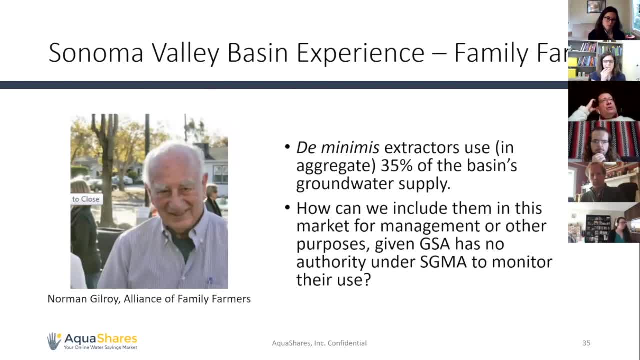 the outcome, Um, and finally, the family farmers, and this is an important uh, parallel with with fisheries I don't think we'd really gotten into is that you know, you often think of recreational fishermen, uh, as a small component compared to the huge commercial fishermen. 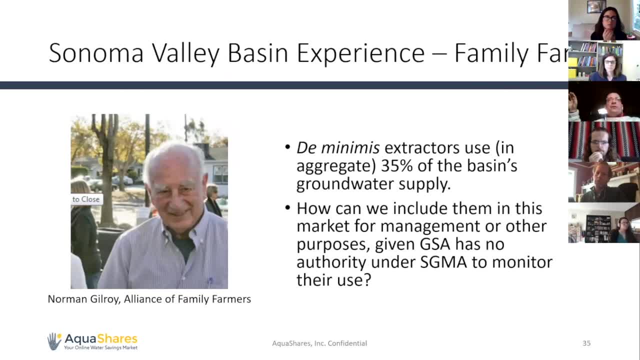 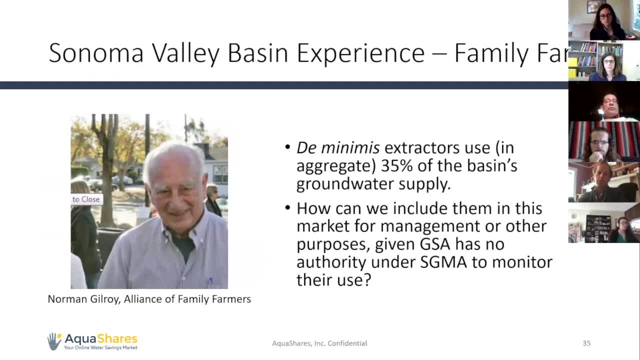 fish taken by recreational fishermen- And Sonoma- this was a case that I think we're starting to see- of these decentralized well owners that maybe only use two to five or six acre feet a year but, in aggregate, eat up a lot of the basins groundwater supply, uh, and they may be de minimis. 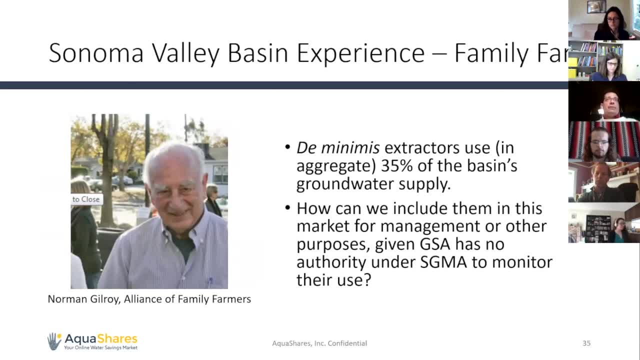 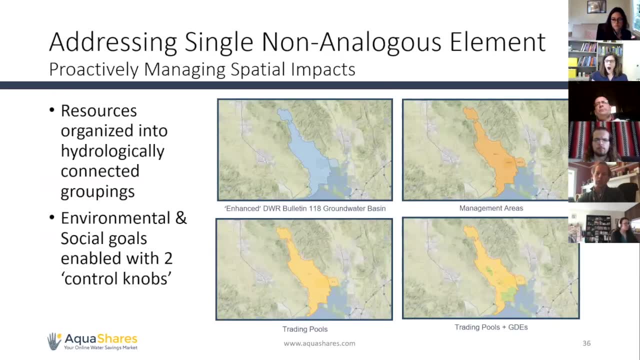 And so how do they get incorporated? Do they want to be incorporated and have an opportunity to benefit from using less? uh? who speaks for them? And bringing that into the equation was also essential. Finally, there's- it's not all- parallels. you know fish. there may be hundreds of different species, different reproduction rates and so forth. 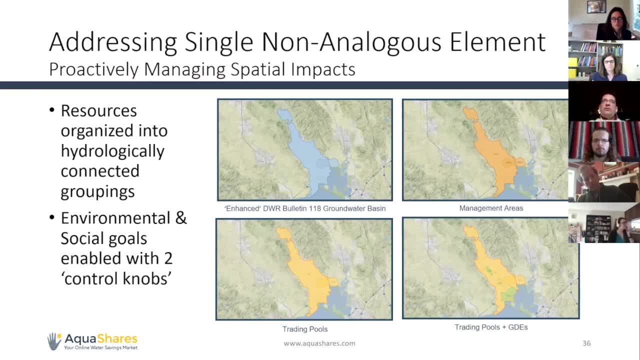 And that was a complexity along California's coast- that the catch shares adapted and worked out. Similarly, in groundwater you have the different levels, the different spatial impacts of hydrologically connected or disconnected aquifers And needing to define and adapt your trading pools, your capacity, to those 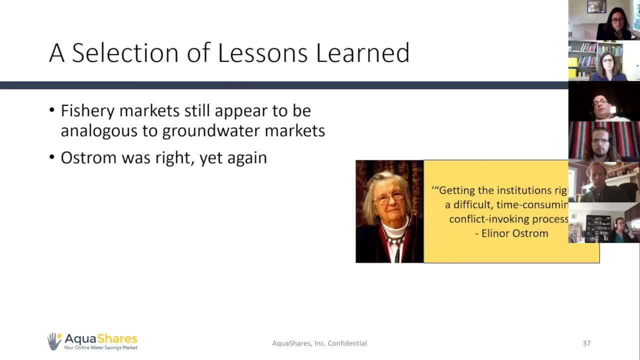 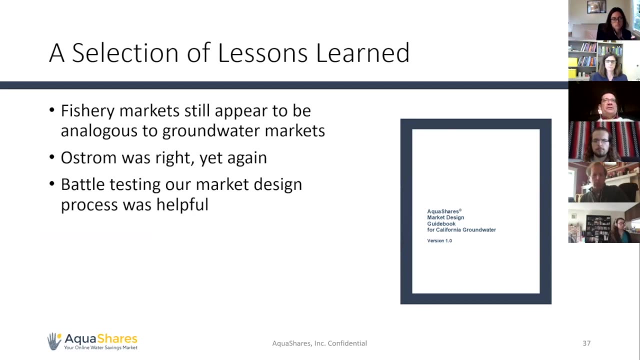 Again, just building back on these lessons learned through this process. Ostrom, yep, she's right for us to sort of use her as the guiding force. There is a strong analogy. We were able to borrow a lot of the lessons and processes and steps and timetables and principles from catch share market design. 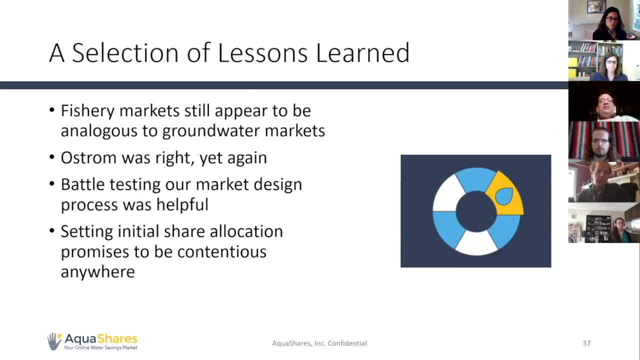 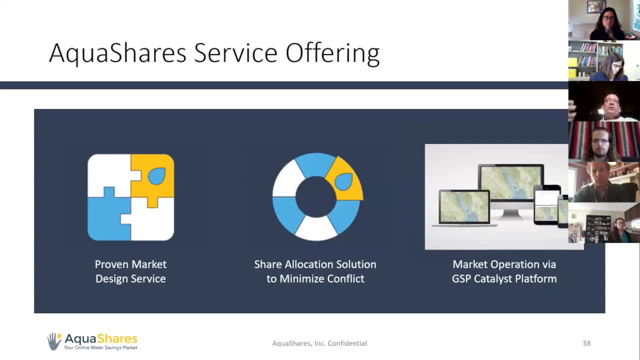 For Groundwater. and, yes, setting that share allocation is going to be contentious, but now we have at least now this foundation that is in instead has worked in 200 cases around the world. You've got share allocation solutions that can minimize the conflict and then you can have this transparent process for operating that, that market. Thanks for this. 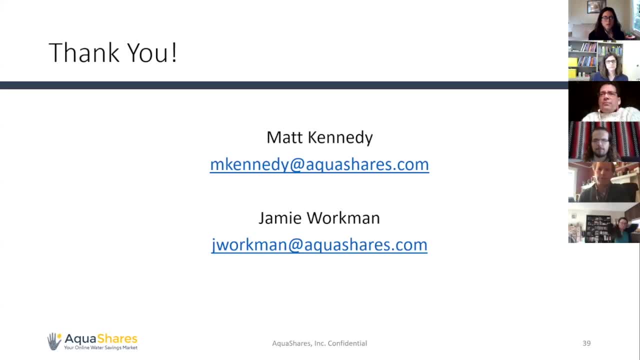 Thanks so much, Jamie. I gotta hand it over now for Brittany to Brittany, Who's going to manage some of the Q&A. Yeah, so we have a couple of questions. If anybody else in the audience has questions for any of the panelists, feel free to enter them in the Q&A. 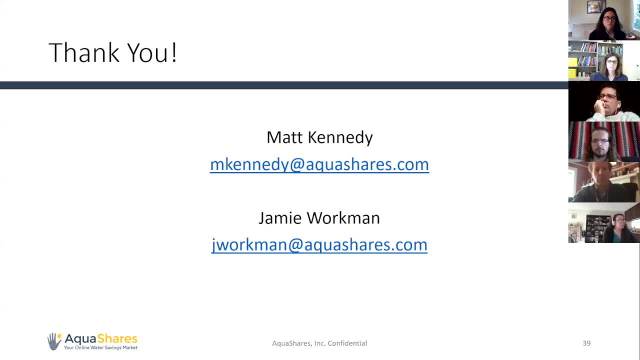 So we'll get started. We had a couple of questions from Emmanuel, who has now logged off, but hopefully he will access the recording after this. So his original question was for Arthur, but I think probably You all may be able to answer it. 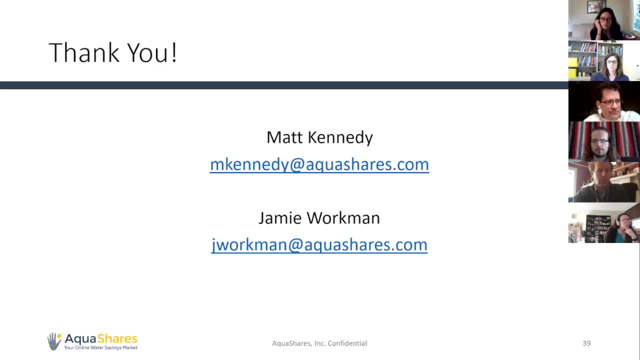 To contribute to this. So he says you suggested a fee for managing groundwater basins, essentially implying that it serves as an extraction costs or fee. How would you set it up? would it serve as a price for for groundwater trading? for groundwater We know that there is a marginal user costs reflecting the inner temporal opportunity cost of groundwater use. 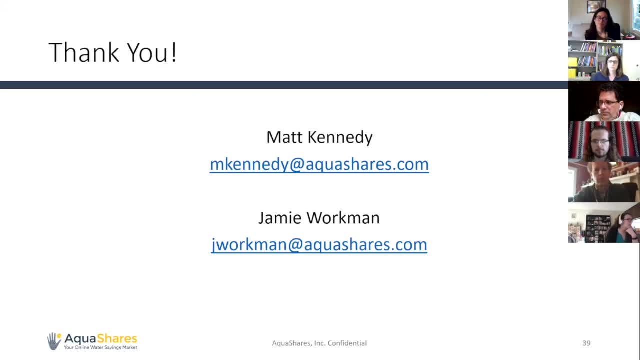 So we'll go ahead and start with Arthur, Do you have any Response to that? and then people can add in. Yeah, I'll say, in terms of optimal management, There's a lot of different ways that you can set up a basin, or at least optimal in the sense that economists think about it in terms of economic efficiency. We've certainly heard there's plenty of other considerations too. 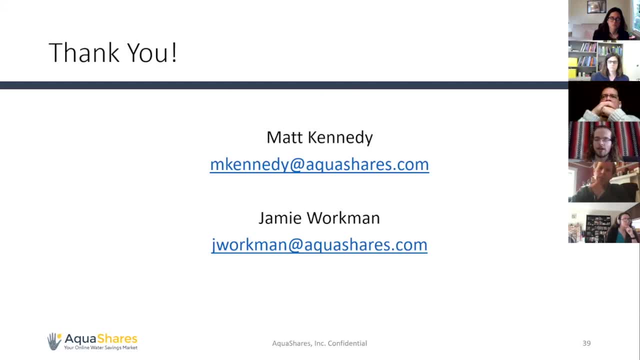 But you know, in theory you can set a fee at the right amount that will Incentivize just the right amount of efficiency, Incentivize just the right amount of efficiency Improvements and things like that that can bring a groundwater basin back into sustainability. 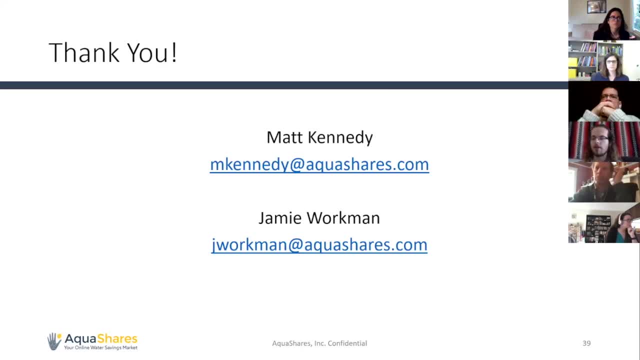 Or you can do that with other tools like allocations and trading, and might not need to impose any outright fee whatsoever. But in terms of how fees are actually being used under Sigma, First, I want to say that a lot of these GSPs are really vague about a what exactly the fee is going to be based on and also what level it's going to be set at. 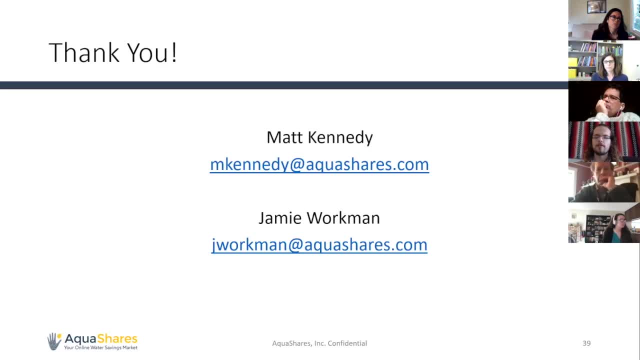 But it's also quite clear that many of the GSA's Are using Fees. they're not thinking of these primarily as a way of incentivizing reductions and extraction by imposing a price on extraction- although that might be a secondary benefit- But they're thinking of them largely as just a way of raising funds in order to support the administrative tasks of the GSA's, which is Caitlin mentioned. there's there's administrative costs associated with the types of actions that these GSA's are going to be undertaking, So I think that explains why we see a lot of these GSAs being used under Sigma. 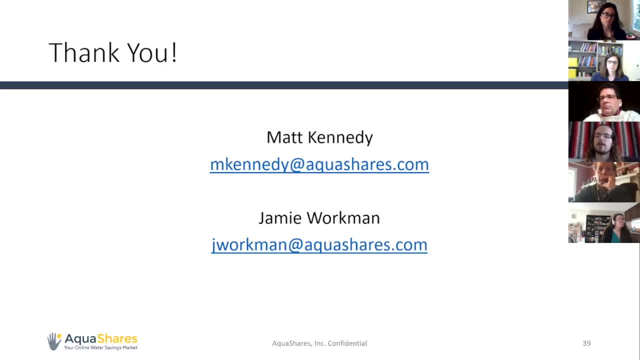 So I think that explains why we see a lot of these GSAs being used under Sigma. So I think that explains why we see a lot of these GSAs being used under Sigma. So we all know that there are many Locate fees levied upon things like irrigated acreage. 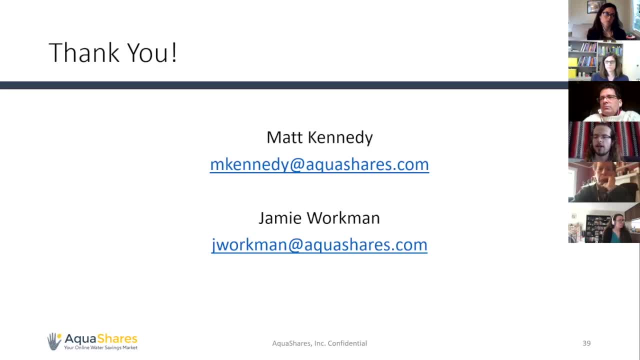 We all know that there are many Locate fees levied upon things like irrigated acreage Or even just planted acreage that have a much looser connection to extraction itself. Saindra Rose, Great Thanks, Arthur. Jenny or Kalynn, do you have anything to add to that? 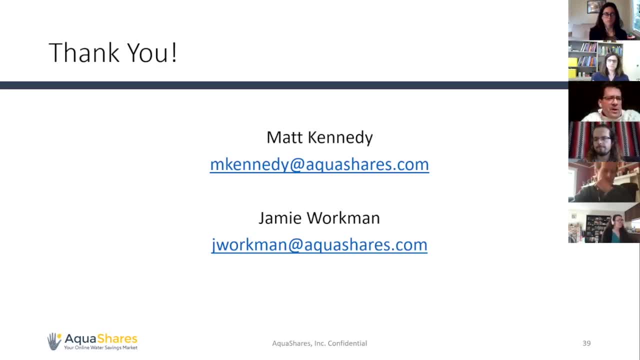 Katelyn Mercury. I would add a little bit that A fee is economically and effective tool and it's a political suicide technology as well. that, uh, unilaterally imposing a fee that you know economists tell you is, you know we'll get the results you want, it will generate backlash, you know, ironically, will generate backlash among. 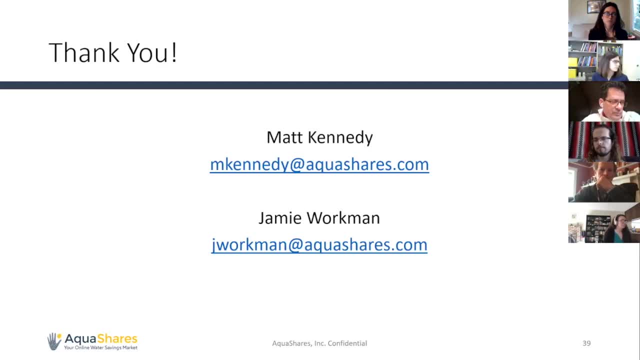 the lower water users. um, we've seen this, uh, at the urban level for for for decades, uh, that you know, raising the price of water from um 50 cents a cubic meter to 55 cents a cubic meter can can topple a government. um, i've actually seen it in a town that i i lived in. i tried to warn them and 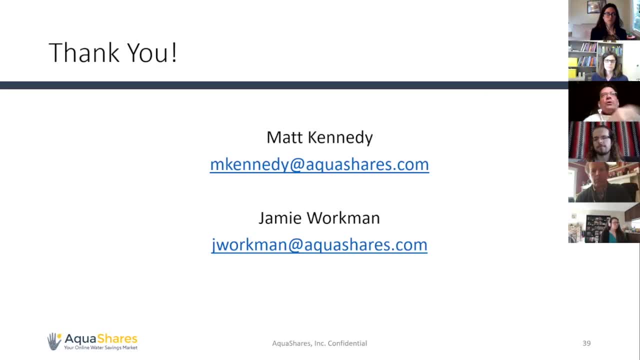 they said, nope, we need to raise some revenues. we're going to double the the rates, and that whole board was voted out the the next election on that issue. um, so it is an effective tool, but you often it's one of the reasons you don't see economists running for office. uh, on a, you know, vote for me. 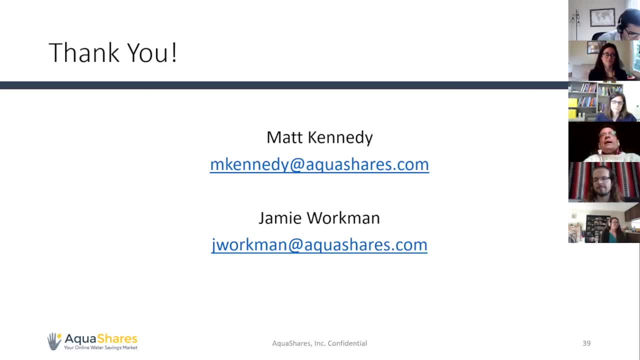 and i will raise fees across the board. um, what i, what i you know, i think, is that, if you can get the same results, uh, and this is one of the reasons why there's, you know, movement towards or embrace the government, and i think it's a good thing to do that. um, and i think it's a good thing. 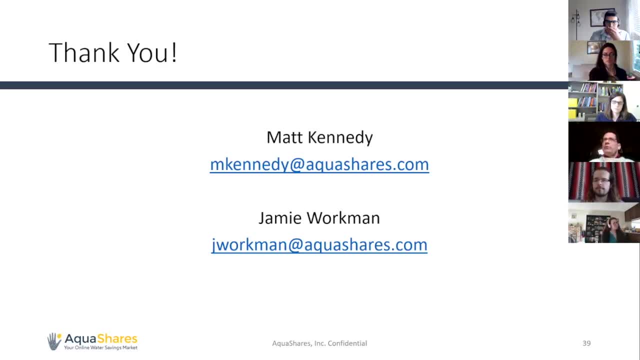 to do that, um, and i think it's a good thing to do that, um, and i think it's a good thing to do that- is that it encourages innovation, not just efficiency. it encourages investment of people looking- uh, you know- a few years down the road, if they have some stake in the outcome, if they can. 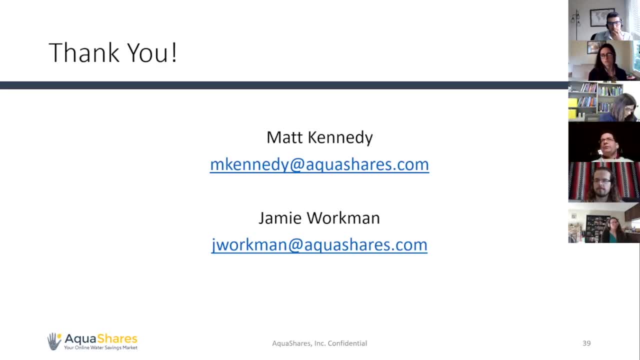 benefit from it instead of just, you know, paying the price of of what they're already using. okay, great, all right, we'll um move on to emmanuel's second question, which is um for caitlyn, but again, i think um probably jamie can add add to this as well. um, we have been trained as economists to look at economic efficiency at. 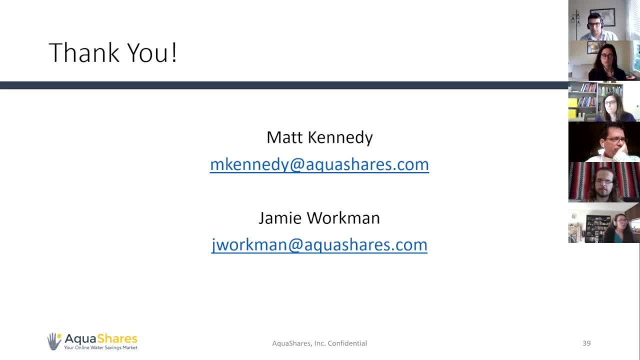 least from an academic purview. on the ground, though, as we engage with stakeholders, we are often asked to address equity or distributional issues or questions as well, um, and some of our policies mandate us to do so. can i ask how we best address equity or distributional issues? 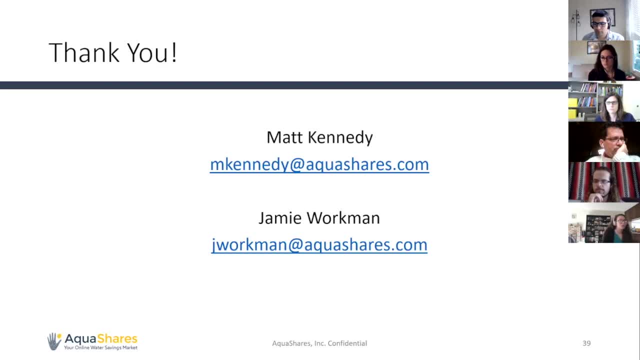 balance that out, balancing the needs and demands of everyone else's while meeting our policy goals. is there anything we can learn from the fishery economics literature? how does groundwater market do that? um any best practices that you would suggest? there's a lot of questions in there, so 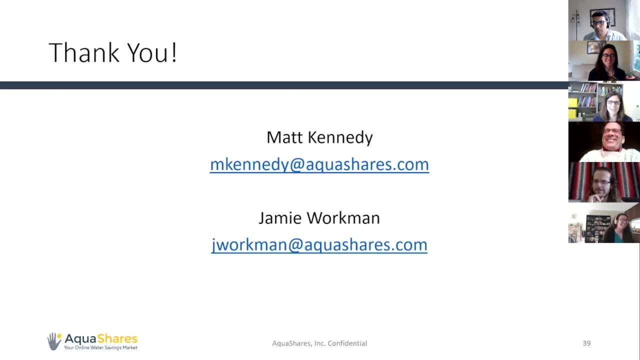 there are a lot of questions. yeah, i'm not sure. uh, i can remember them all off the top of my head, but let me dig in a little bit and then maybe jamie will jump in after me. um, i guess just a couple big picture points. uh, i think that there's a lot of opportunity for economists to collaborate more with. 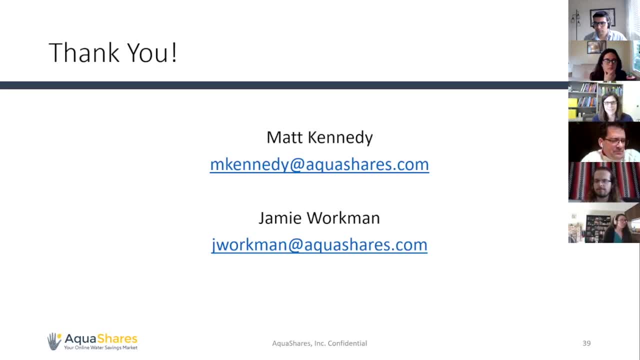 non-economist social scientists, and so not to think that we really have the answer here just by ourselves, but that this might be a really good opportunity for more sort of interdisciplinary collaborations. um, in my own experience- and i think this would be borne out sort of searching through the fishery literature, these are harder things to quantify sometimes and 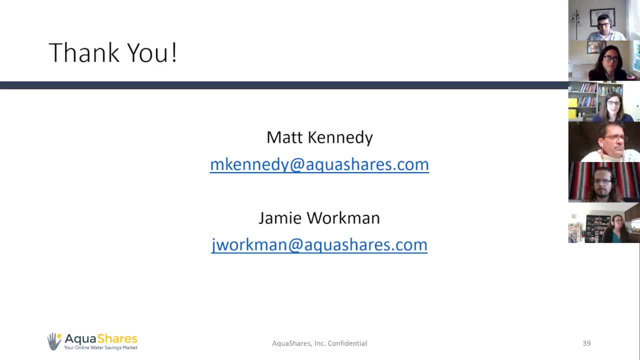 i think they're. they're hard for other non, uh, economists, social scientists, to quantify, and so, uh, i think, sort of by nature these are, these are harder things to assess versus something like, you know, ecology goals, what's a sustainable fish stock level, or something like that. so i think these are are more challenging in some ways. um, i think that 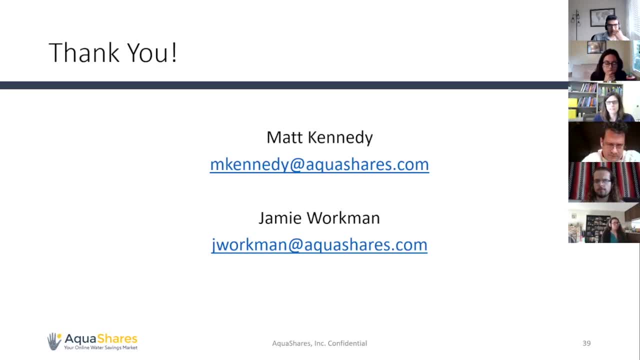 economists do have a lot to add to this space, in the sense that i think a lot of the modeling approaches that economists use can be used to inform um some of the the really hard questions that policymakers are facing, and i guess, in framing my answer that way, i would also emphasize that 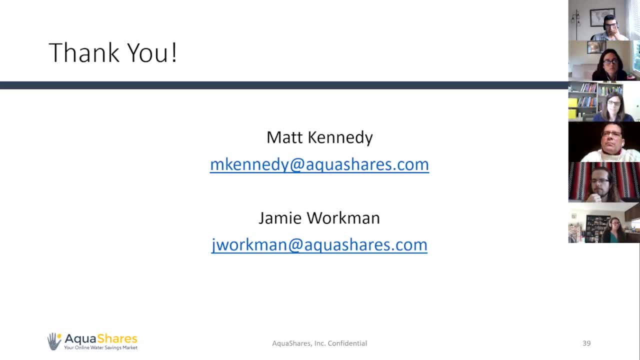 you know, i don't think that economists necessarily need to say here's the answer, but that there's a lot of power in some of the tools that economists have developed over time to better articulate what the trade-offs are between different, say, program designs or things along those lines, and so to use. 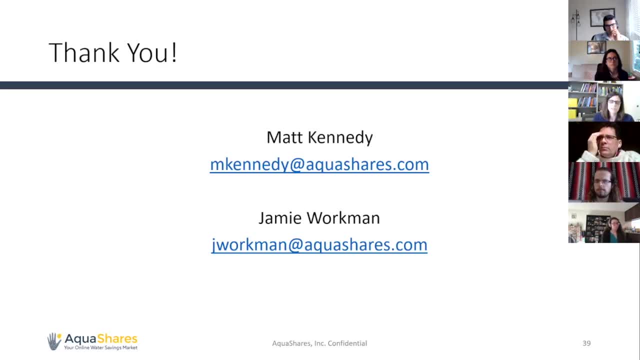 the tools to really try to present options to the community and uh and to flesh out what are the potential projected sort of outcomes in terms of some of the uh social outcomes they care about. where will the allocations end up, uh? what will the final number of participants be? 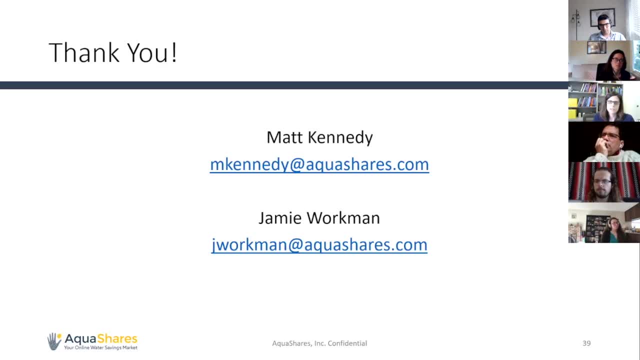 uh, under different policy designs, so i don't know. jamie, did you catch more questions? do you have things to know? i, i think that was a great answer and i, i, i would only add that one of the things to for us to keep in mind in both groundwater management and- uh, you know, fisheries management. 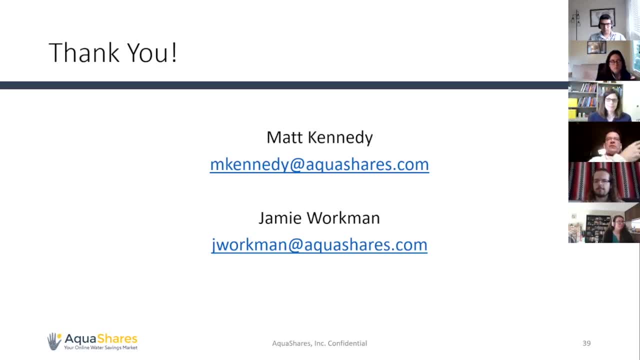 we're not managing groundwater, we're not managing fish, we're managing people and the most effective strategies. people don't like to be managed. they'd much rather manage themselves, and so this is a governance issue. this is a democracy- small d democracy issue, and um, i don't want to get too. 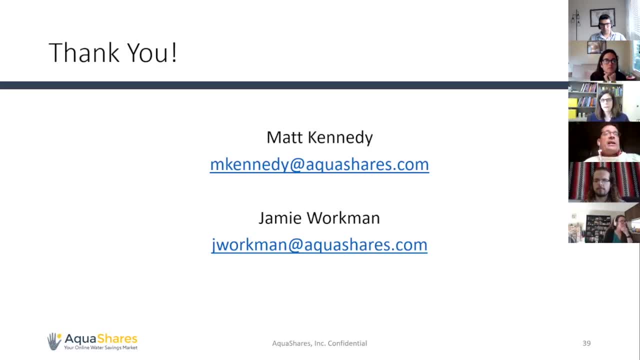 overblown or whatever, but i, what excites us and what excited i think, uh, lynn ostrom, um, anyone who's worked on a catch share or you know a market design for, um, for for groundwater, is a sense of, of being present at the creation and i feel sometimes like it was. 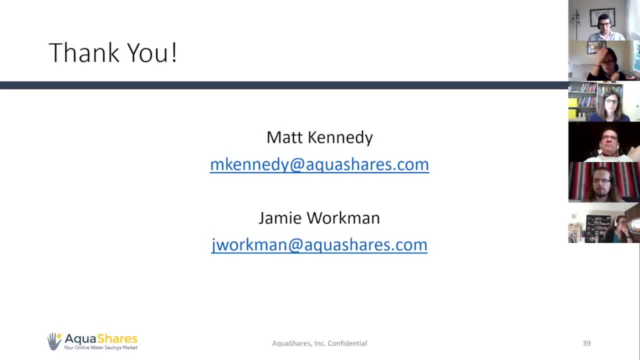 you know like it might have been with a constitutional convention, um, the difference being, instead of a bunch of old white male property owners, you got a much more diverse group at the table and and had, in, you know, 1989 or whatever, uh, you had, uh, women at the table. 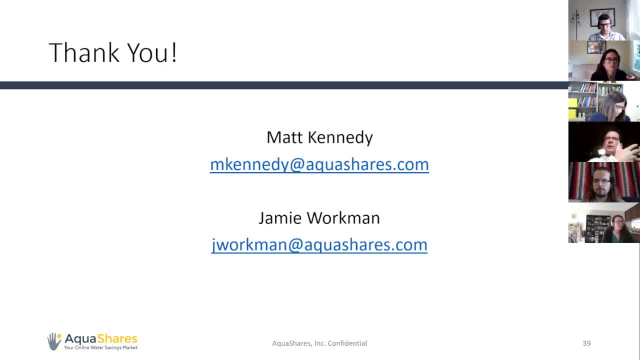 youth at the table, non-property owners, slaves- uh, ideally liberalized slaves at the table? um, you would have a much different constitution than the one that we're still working with. that said, the, the creation of this management of the commons, you know, leaves the room open for evolution, for improvement, for iteration over time, and so that the the first 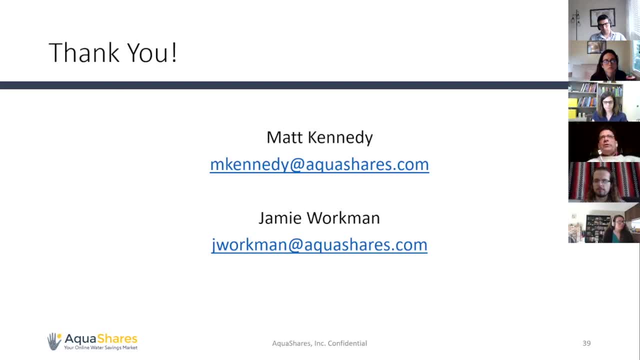 catch shares, like in iceland, that benefited and made millionaires out of, you know, these icelandic fishermen. that's not the kind of catch shares that we're looking at today and they are much more inclusive of environmental, of social, of of governance and political inclusion. um that, uh, that they wouldn't have. 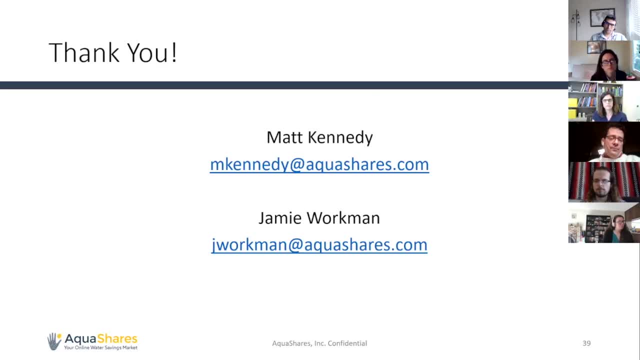 crossed their minds, uh, in the past. all right, thank you both for your answers, um. the next question is for kaylin. have there been any examples of taxes or fee type economic instruments for managing fisheries? um, for managing the quantity that you would extract i? i guess i'm going to go back. i thought that, uh, arthur. 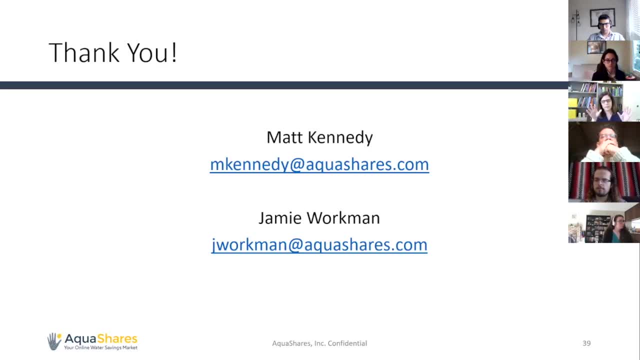 did a really nice job dividing um these tax and fee kind of questions into: are you using it as an instrument to manage the total extraction or are you using it as an instrument to, uh, extract some of the profit to fund management and britney? can i just 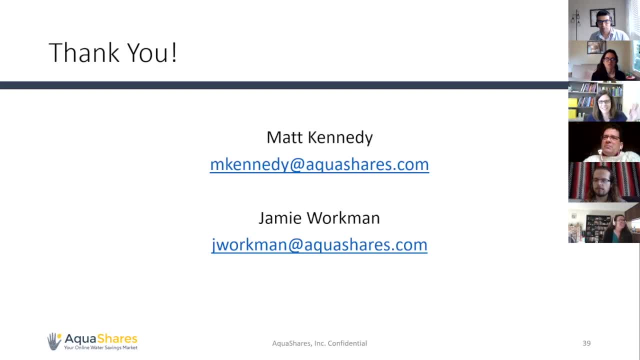 i'm going to go back to you. can you understand? you read that and i. i think i didn't catch which question that relates to. um, i'm not sure. uh, ellen, yeah, sorry, that was a question that came from me. um, i was just i mean, i guess, yeah, i, we had all this discussion about markets for managing. 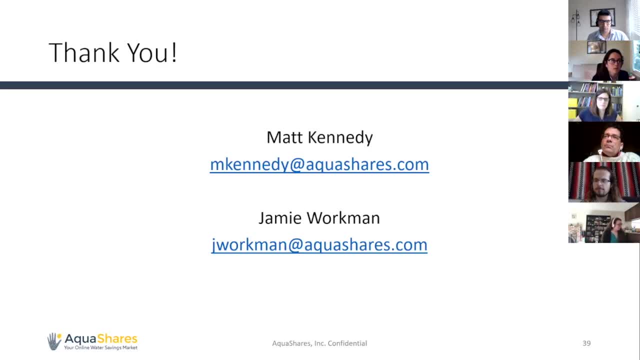 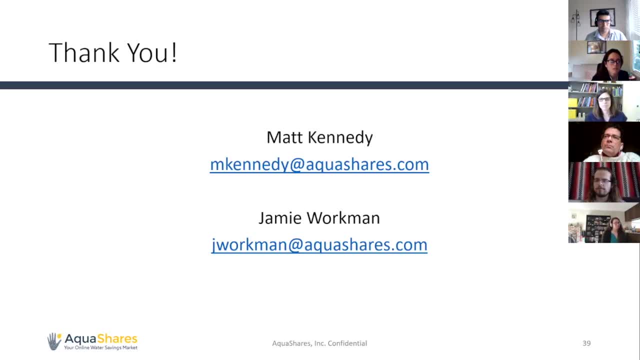 and i'm going to go back to you and so you know, obviously there are. there's this administrative component, and that's certainly what's being proposed in the sigma context, or these fees to cover those administrative costs. and i was just curious if there have been any examples. 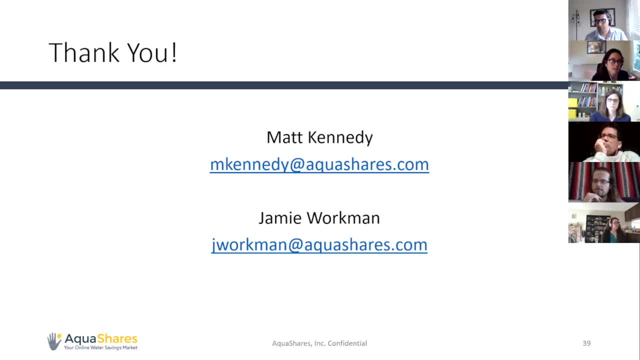 in fisheries management historically, where taxes were used as a tool for achieving sustainability of those fisheries, not just covering these administrative costs, and maybe it never has happened because it's just too politically contentious. but i was just curious if you had any, um, if you had any examples off the top of your head. yeah, i think that's a really great. 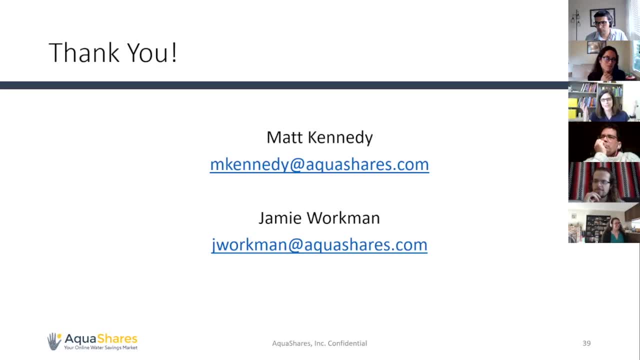 question now that, yeah, why? why not? if we always do, we kind of contrast the tax versus the cap and trade, if we're thinking about environmental regulations or something like urban right, um, and yeah, historically that has not gone over in the fisheries context, for you know more political. 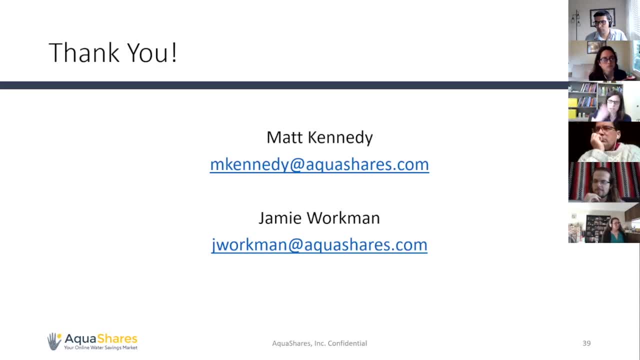 reasons, but one of the things that i think is really interesting, i would add. you know, jamie talked a little bit about the fish and water context and how a lot of the fish that are in the fisheries context and how diverse people are to paying to access these resources. but if we think 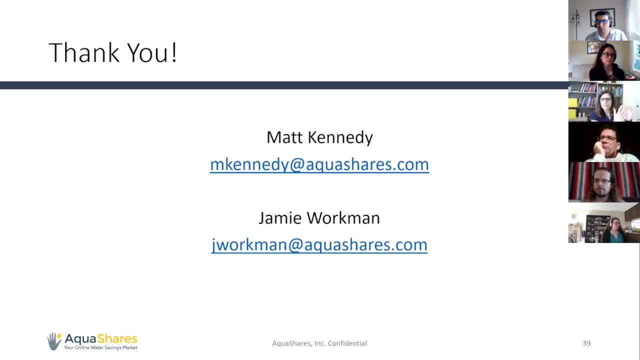 of something like oil there. it's very well accepted that you know these is uh, this is something that is our country's resource and so if you're going to access it you pay for it. but somehow that has not transferred over and i think maybe because of the history. so you know, historically especially, 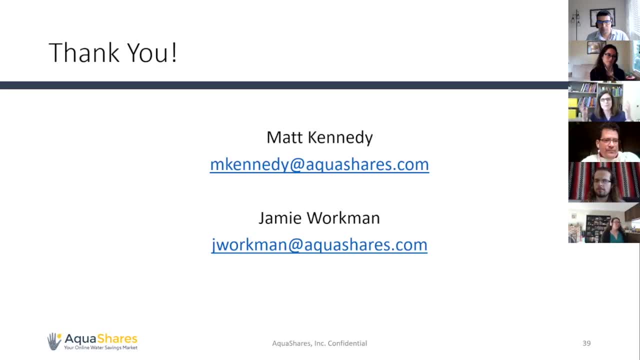 on the east coast, access was free, and so if it's free at one point, um, is it really hard to then revert to a scheme where you would really heavily tax for for access? and so, um, no ellen, i think the answer is that, uh, sort of the precursor to these programs that really think more about economic. 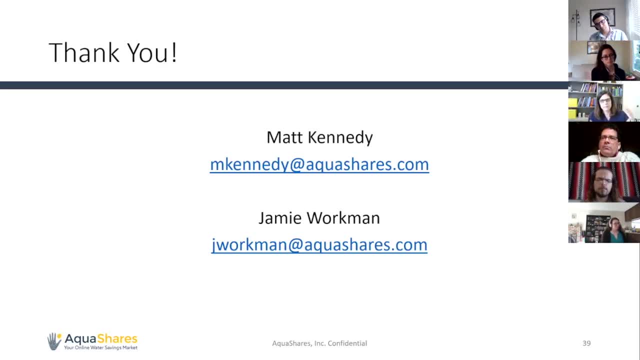 efficiency. if you're thinking more of an environmental kind of limit, you would implement something where you would just track the landings and then you would close once that environmental limit uh was hit. and so when we think of contrasting different management regimes and fisheries, that would be more of the contrast that that i would build. yeah, thank you. 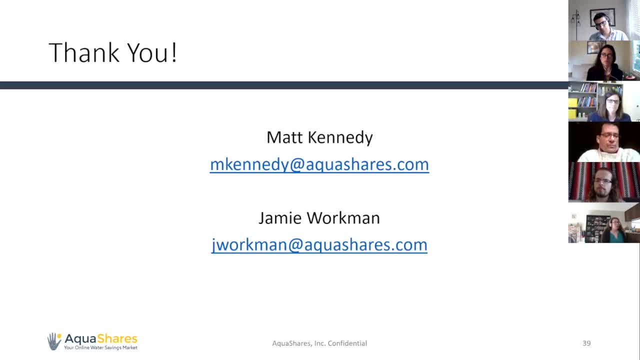 all right, um, and then i think caitlin kind of covered the the second part of your question, ellen, um, about what i don't even know. oh yeah, i actually covered that. sorry, couldn't even remember what the second part was. i think that's all of the questions that we have and i guess we're 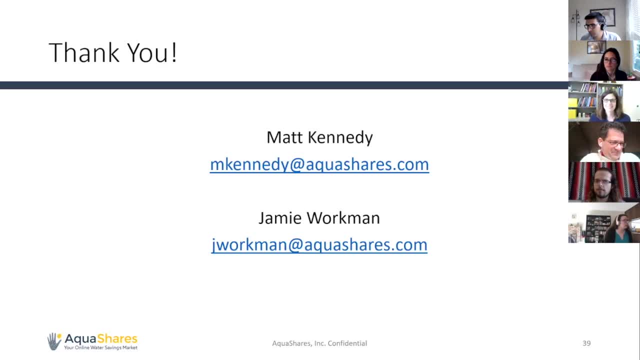 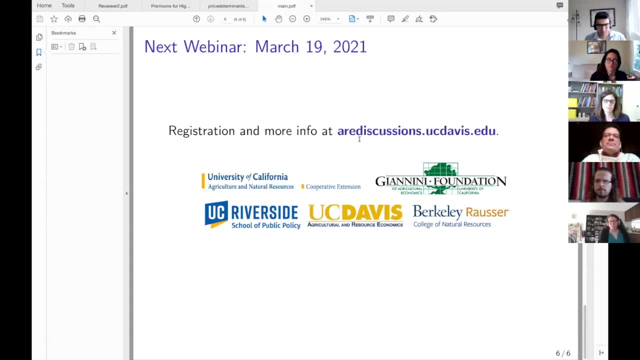 we're just about out, so i'll go ahead and um share my screen with the last um. can you see everyone? so, um, yeah, i just wanted to highlight. oh, thank you for all of the panelists that took part today. this was really interesting. i learned a lot about fisheries. 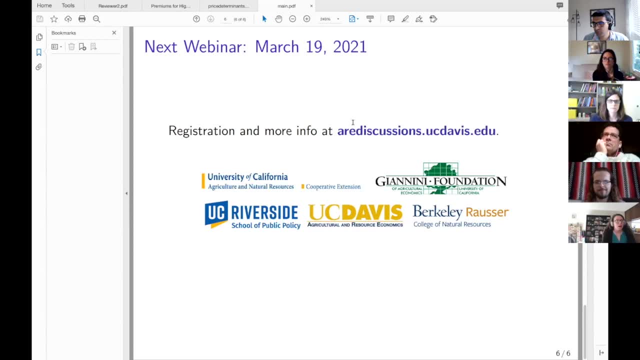 and and sigma, and how we can sort of link the two um and so next, the next webinar will be march 19th. we're still determining what um that will be and getting the speakers around. but, um, you can look for updates on our website, airy discussionsucdavisedu, or or check your email, um, and you can also subscribe on the website. 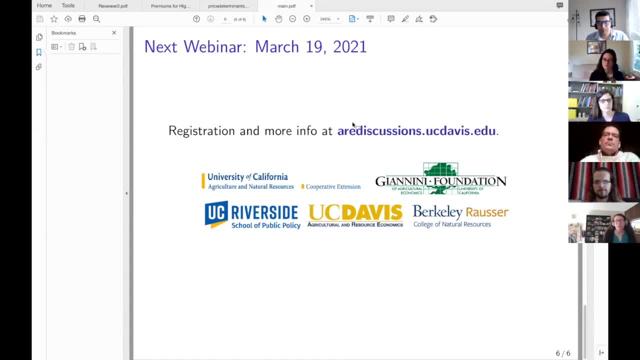 as well. so, thank you all for joining and, um, i think that's it great. thanks for organizing. yeah, this is great. thank you, thank you, thank you.